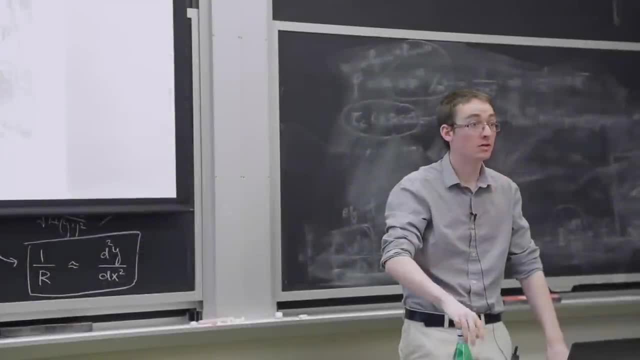 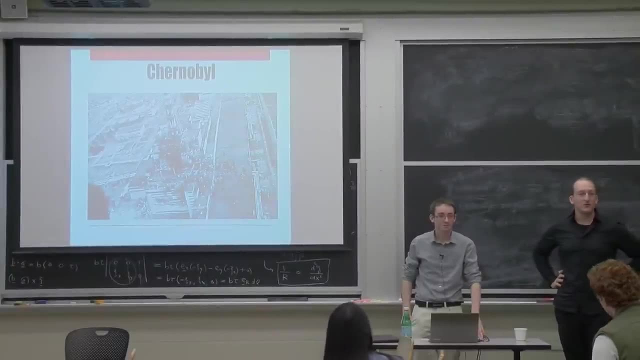 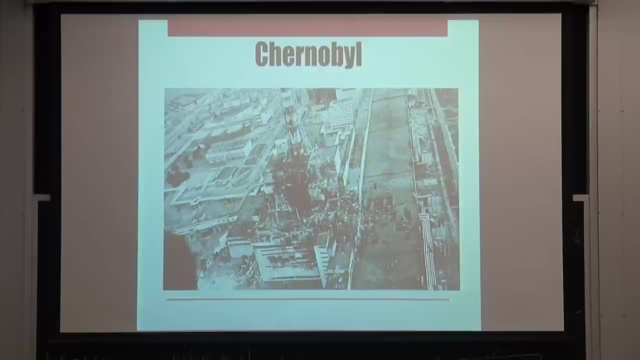 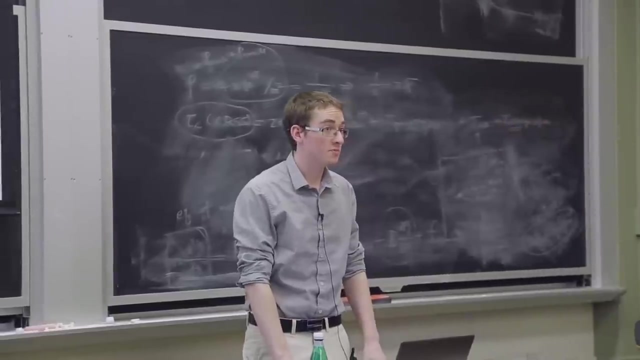 All right. so first off, I'm actually going to go over a bit of the reactor physics involved with the Chernobyl accident. I realize you guys have already covered this to some extent, but I didn't plan on doing it. I didn't plan for that, so it's in my presentation. 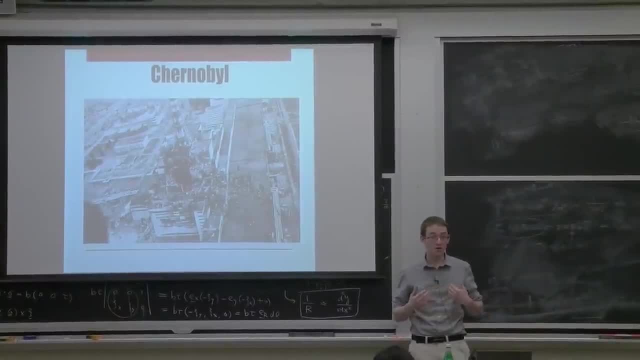 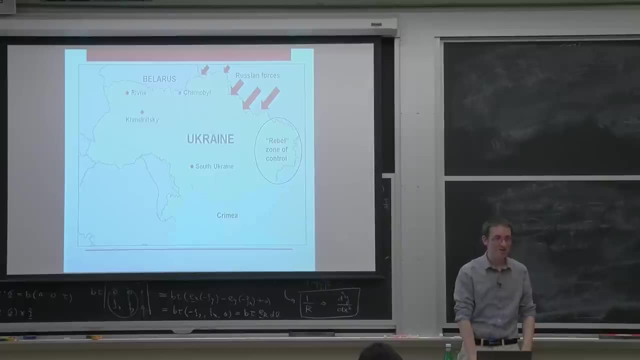 Also, I am a little sick, so I'm probably going to start coughing. Apologies, I'm not dying, it's just a cold. I have heard that joke about eight times in the last two days and I'm so done with it. 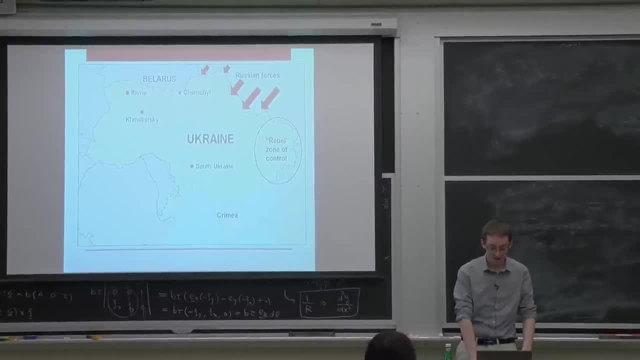 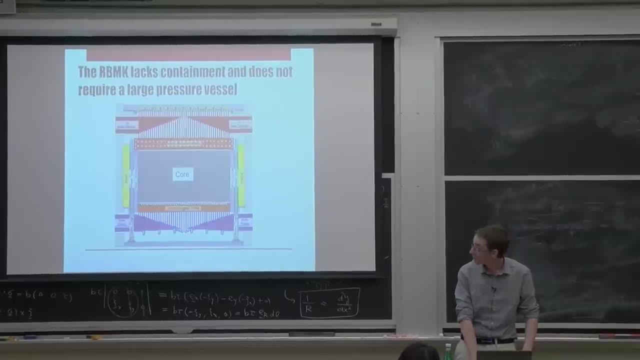 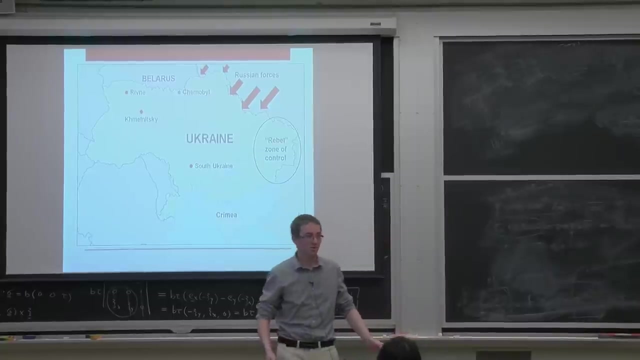 But yes, it's not radiation poisoning. All right, where is Chernobyl? Ah, dang it. come on, No, go the other way, The other way, yep, okay, there, Okay. so one of the first questions I got when I said I'm going to go and visit Chernobyl is: 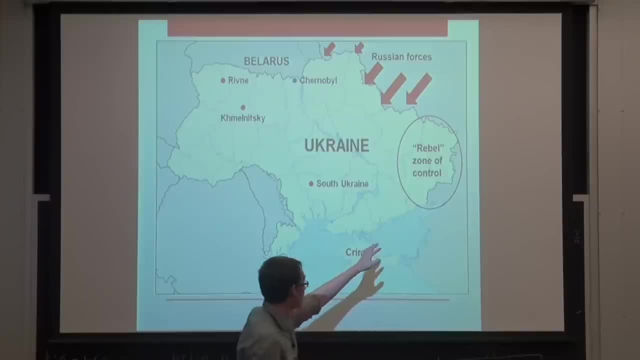 wait, isn't that a war zone? Not quite So the Ukrainian. the war in Ukraine is mostly in this portion over here. It's not entirely under rebel control in that area, and I say rebel in quotation marks, because rebel means Russian. 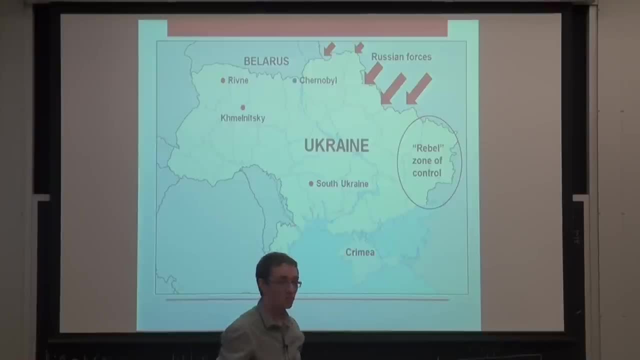 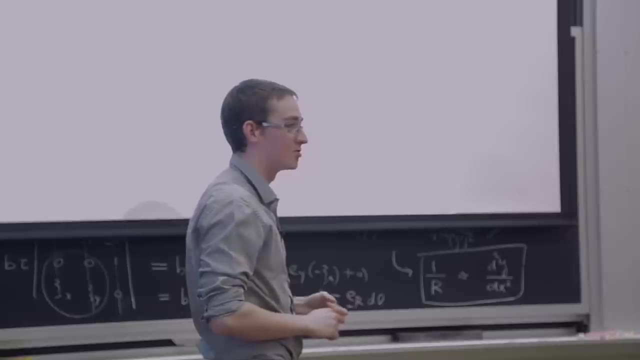 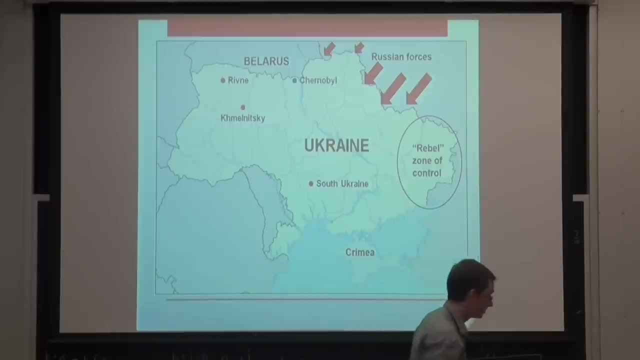 However, if you notice those arrows, Russian forces are built up all along that border. so while it's not an active war zone, it's certainly not a place to be spending a large amount of time. That said, Chernobyl is north of Kiev by about I don't know. let's see 200, 250 kilometers. So it's not completely out in the sticks, right? Hopefully this gives you a good sense of roughly where it is. All right. so what does the Chernobyl nuclear power plant look like? It consists of four finished reactors. There are two unfinished reactors- Unit 5 and 6, that are not shown in this image. 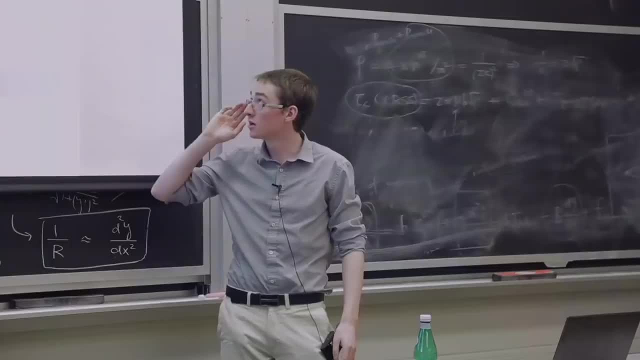 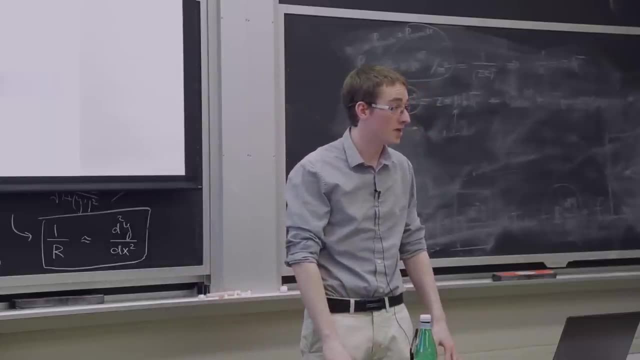 Units 1 and 2 are located at the right. Those were constructed in the 1970s and early 1980s. All of these reactors are of the RBMK type. Units 1 and 2 operated with some success. I'll go into that later. 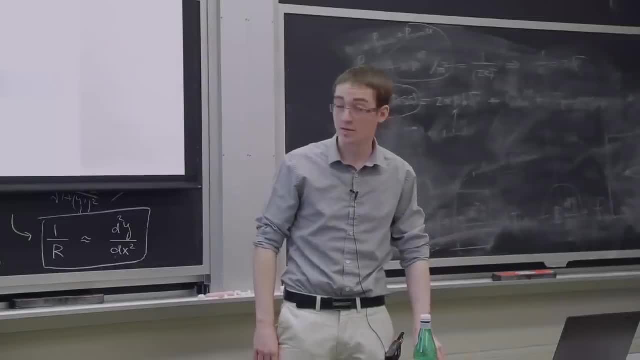 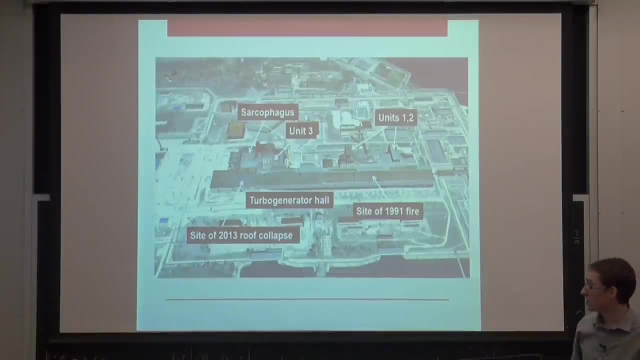 For a number of years before the accident that happened in 1986.. Also, I have some call-outs up here that show some of the incidents that I'll talk about here a little bit later in the presentation, But this just gives you a general idea of the layout. 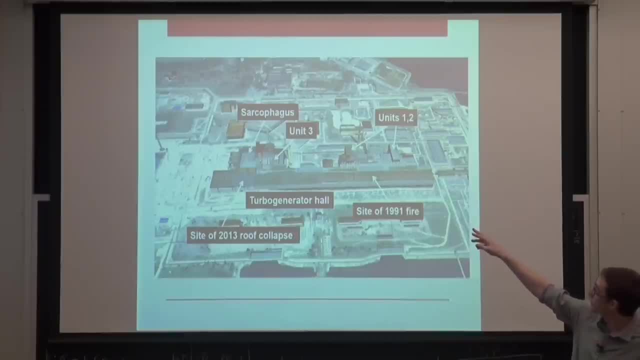 So it's two separate buildings for Units 1 and 2, and then Units 3 and 4 are in one building, all connected by this turbo generator hall. So this is where the generators that turn the steam from the RBMK into power are. 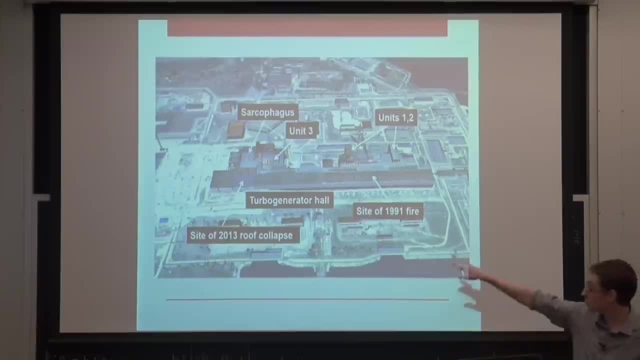 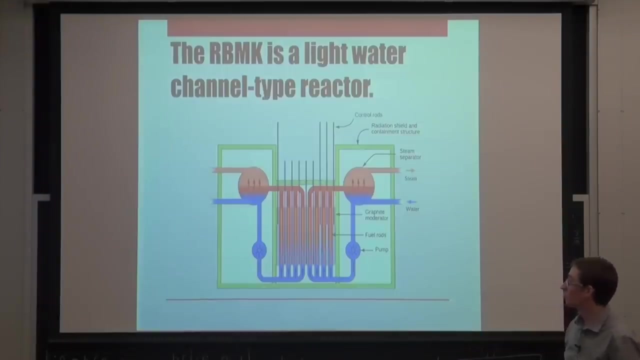 This is one giant. Well before the accident, this was one giant, not-separated hallway, basically, So you could walk from one end to the other, theoretically All right. so what is an RBMK? An RBMK is a light-water-cooled, graphite-moderated channel-type reactor. 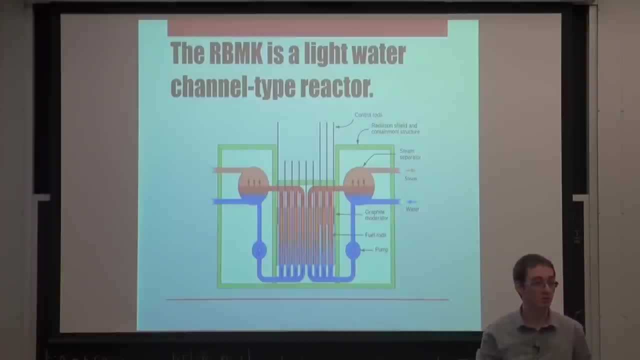 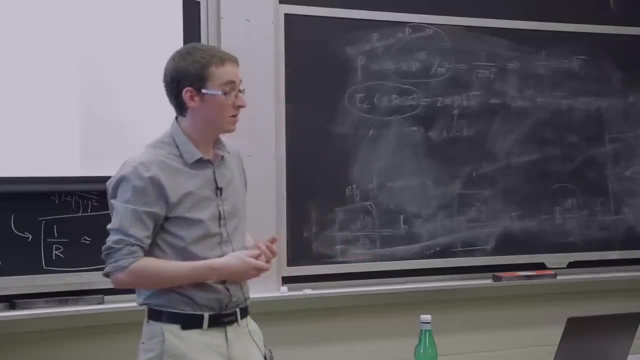 This means that it does not have a giant pressure vessel like you would see in a VVER or an equivalent American light-water reactor. Why does that mean anything? Well, building giant pressure vessels is very difficult, If any of you have done research on manufacturing of nuclear reactors. 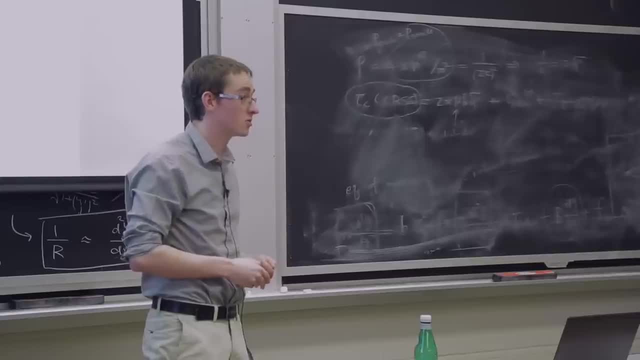 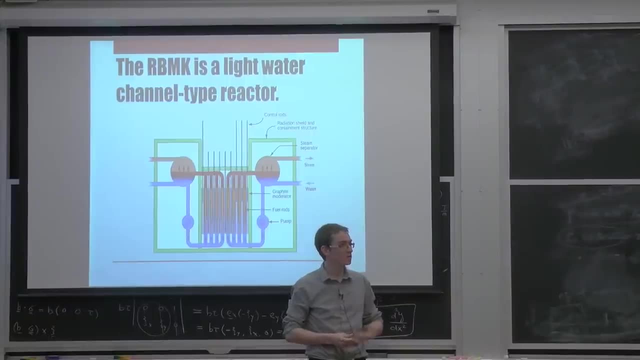 you'll find out that the equipment necessary to construct a reactor pressure vessel is not actually something we even have in the US anymore. Is it Korea that does it for us now? Japan that does it now? In the Soviet times it was. 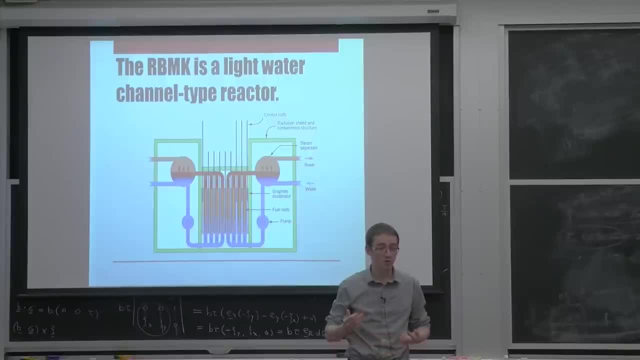 It was very, very difficult for the Soviet Union to produce such pressure vessels at any kind of reasonable rate, So the RBMK got around this by using individual channels that were their own pressure vessel, so to speak. So the way this works is: let's just start on the cold side. 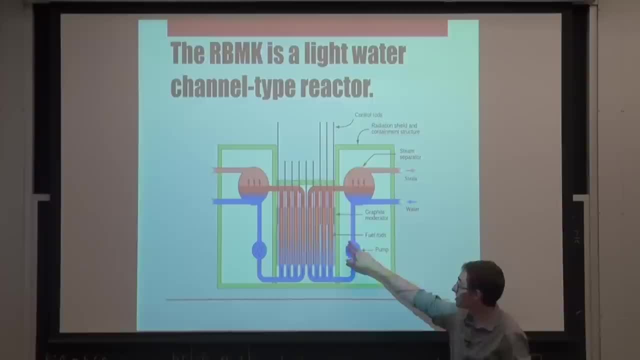 You take in cold water. it goes here through these things. These are main circulating pumps, MCPs, as you'll see them referred to later in the presentation. It goes up through the bottom of the core. These are the hot fuel rods. 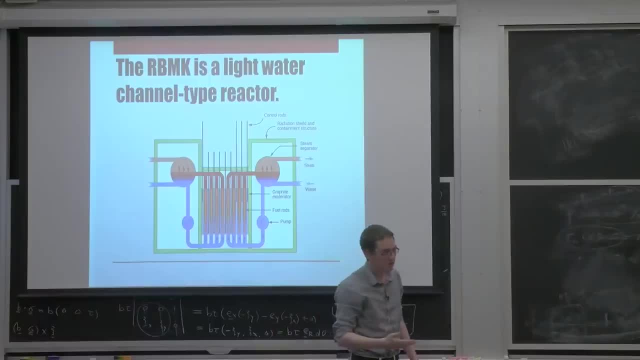 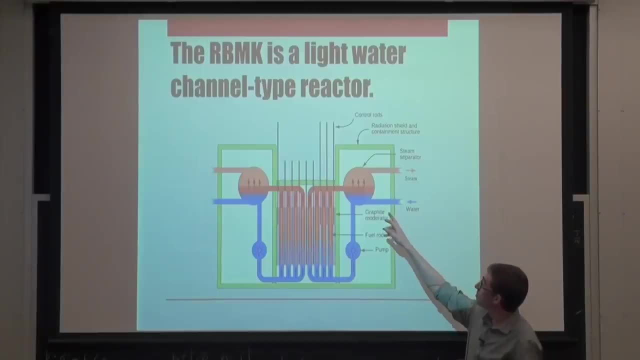 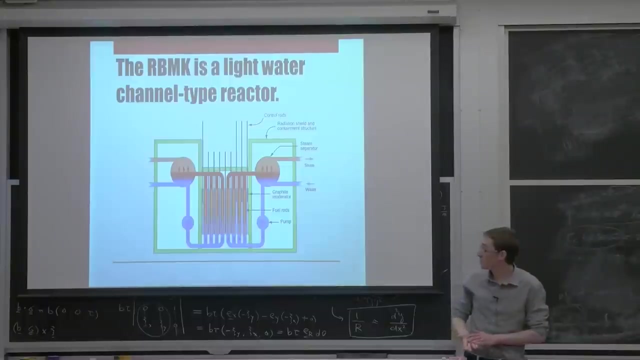 The water goes from liquid to steam phase. as it's flowing through the channels, It comes out the top, goes to the steam-water separators. Steam goes to the turbines, turns the turbines, makes electricity. The important thing to remember here is that we've got a giant graphite core. 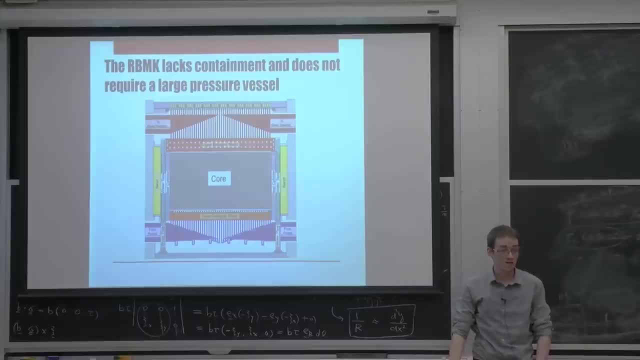 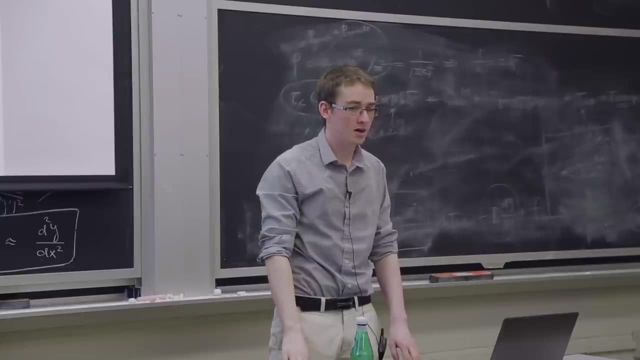 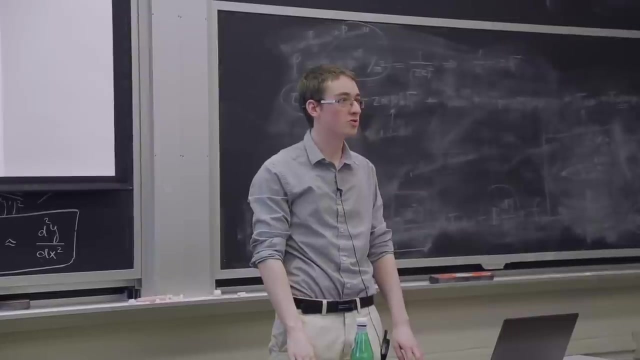 The graphite is what is doing the moderating in this circumstance. It is not the water. This allows you to run very low enriched uranium, So you could theoretically run an RBMK on. I believe it was 1.2% was as low as they could go. 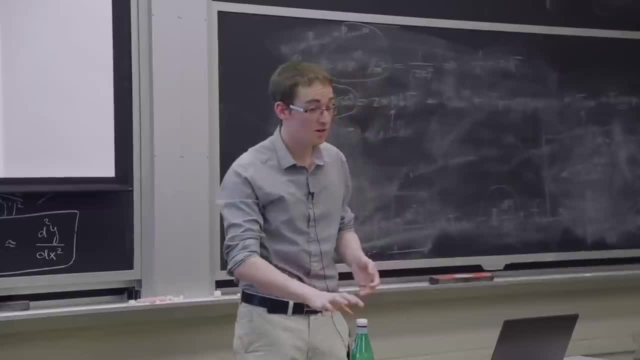 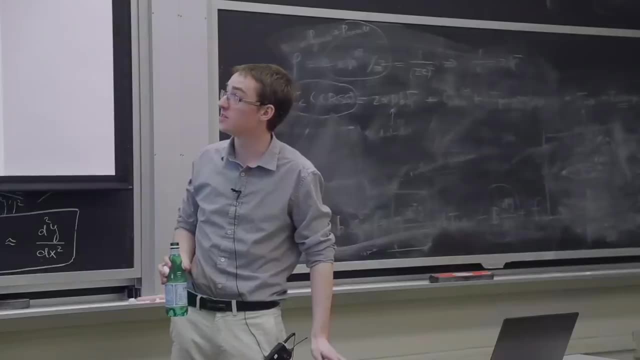 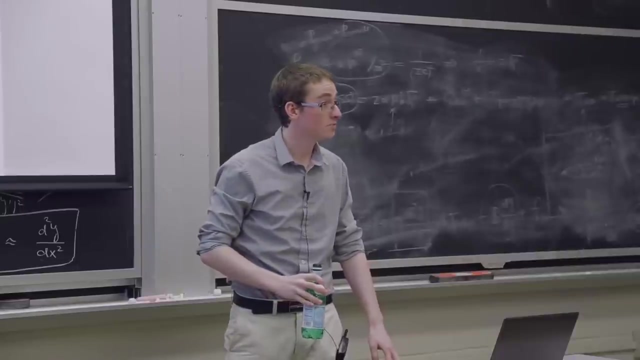 But regardless extremely low enriched uranium, which is convenient if you don't want to waste a lot of time enriching uranium. The problem with this is that you have a giant core. If you recall the scattering cross-section for graphite, it's pretty small. And the amount of energy lost per collision is likewise also fairly small. So the core on this thing is, let's see, 11.5 meters across The core for an equivalent American reactor. so well, there's no real equivalent to this. 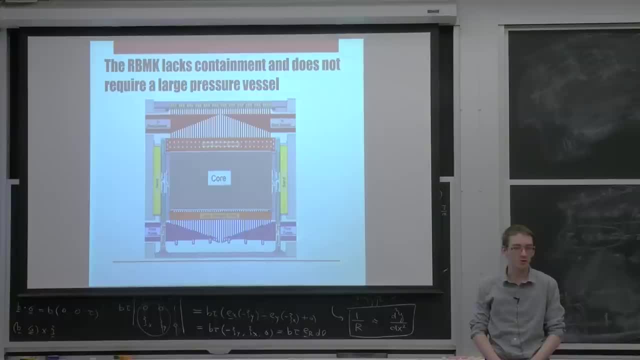 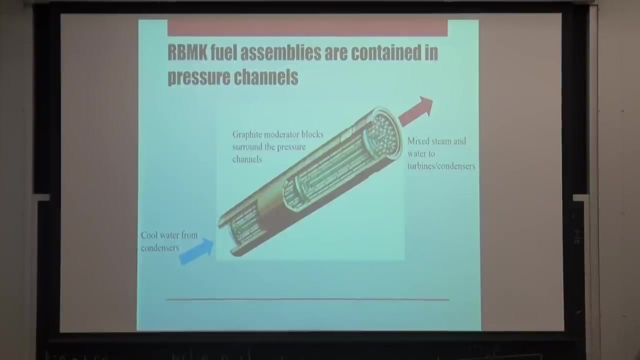 but for, let's say, an AP1000 reactor of equivalent electrical output is about 4 meters across. The core is huge. As I already discussed, this is what the individual pressure channels look like, So cool water comes in the bottom. 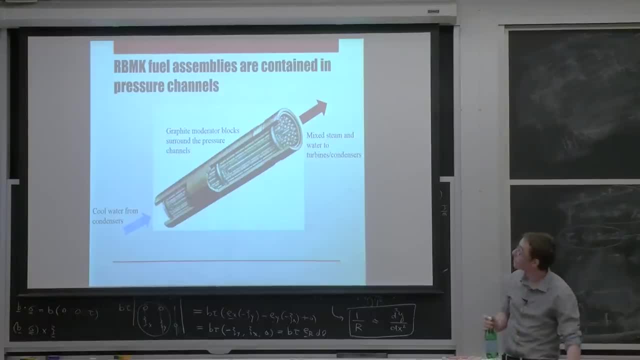 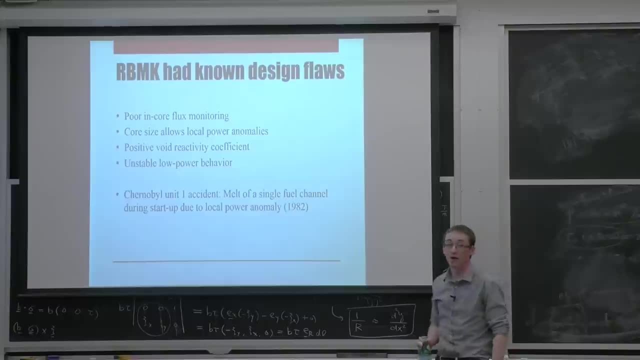 goes by, the fuel rods pops out the top. The RBMK has some serious design flaws. So, as I said, the core is huge. This allows local power anomalies to form really, really easily, Each if you look at the core. one portion can be kind of neutronically separated from the others, because neutrons just don't make it all that far when diffusing across the core. So you can have very, very high power in one corner and very low power in the other, which is not something that can develop in a physically smaller core. 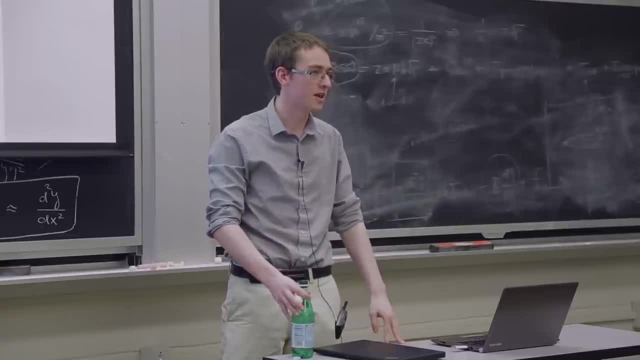 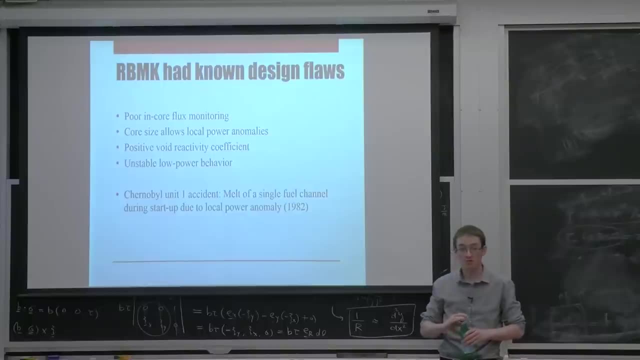 which has a characteristic scale equivalent to that of the neutron mean-free path. Further, the in-core flux monitoring on the RBMK is seriously deficient. So there are a variety of neutron detectors that exist around the periphery of the core, but they're wholly insufficient to catch these local power anomalies. Chernobyl actually found out the hard way. on this one, In 1982, Unit 1 suffered a quote- localized core melt- not really something that can happen in an LWR or really any other type of reactor, But a couple of the fuel channels actually experienced. 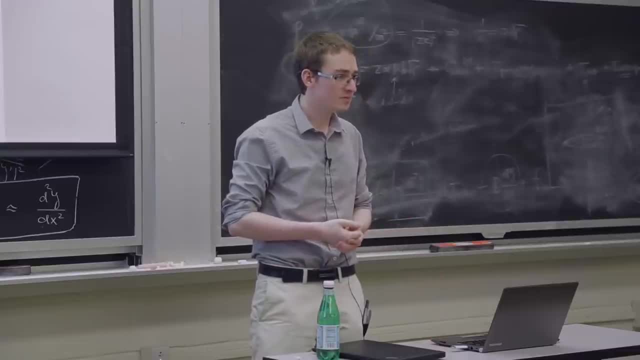 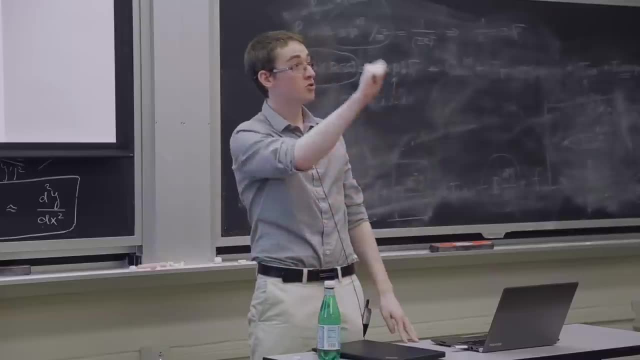 one of these local power anomalies and ended up melting. So if you go into the control room of Unit 1, you can see that on the fuel channel cartogram on the wall there are two of them that are just sharpied out and those are the ones that melted. 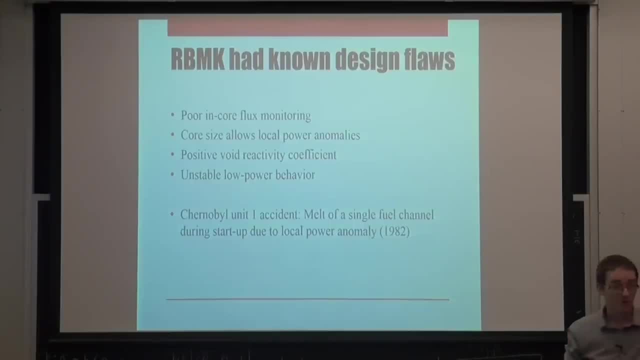 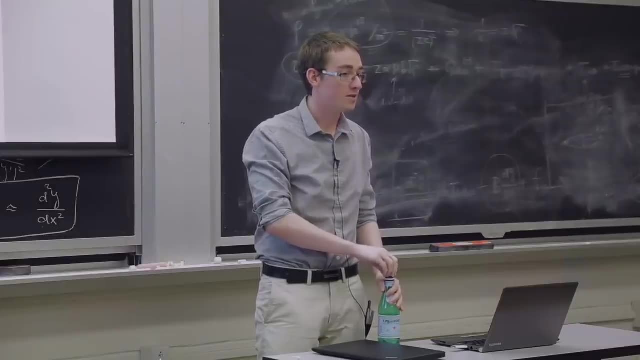 Further, it has a positive void reactivity coefficient. What does that mean? Well, when the water boils in the core, the density of the water there goes down and the power of the reactor ends up going up. because the water is primarily acting, not as moderator. 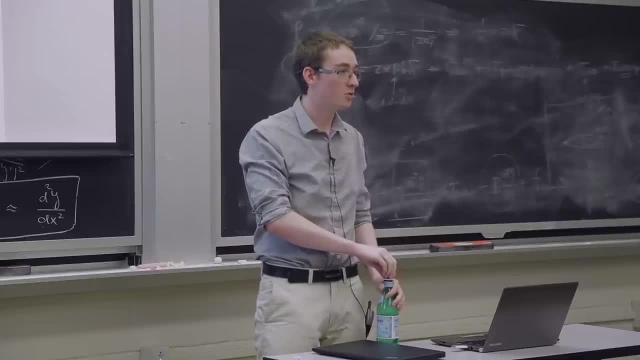 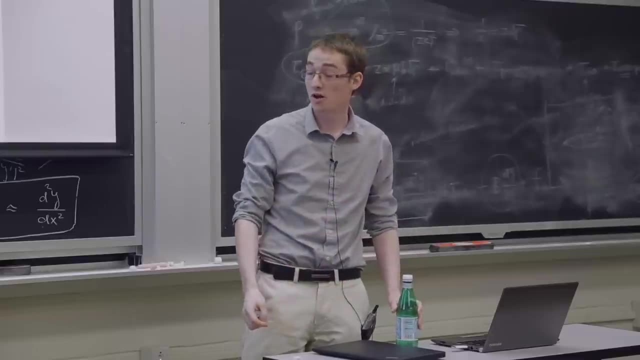 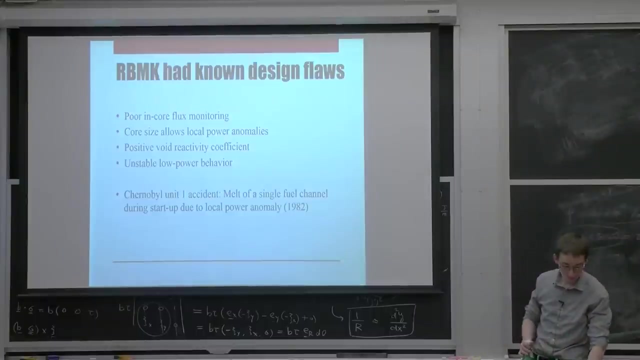 but as an inhibitor, It's a neutron absorber. This is bad for a whole variety of reasons and they found out quite catastrophically in 1986 exactly why. Further, the system is extremely unstable at low power. So how did the 1986 accident happen? 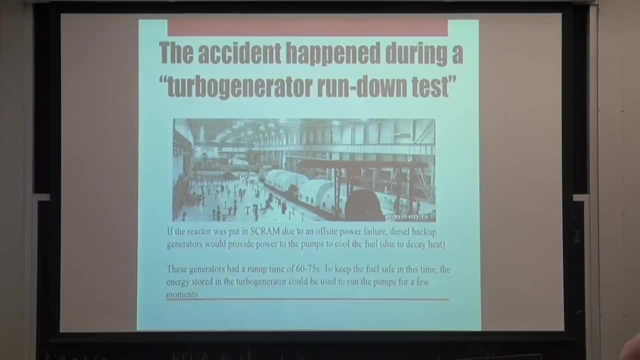 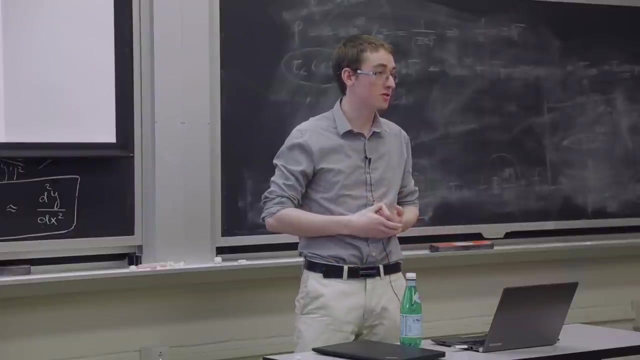 It was part of this thing called a turbo generator rundown test. The general idea is that if you have an off-site power failure and your main circulating pumps no longer have off-site power, you somehow need to keep water flowing through the core such that the fuel does not melt. 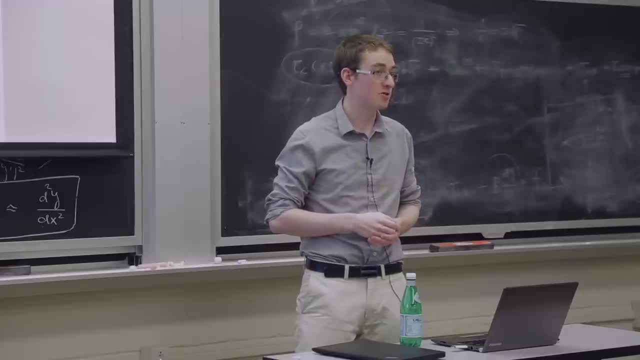 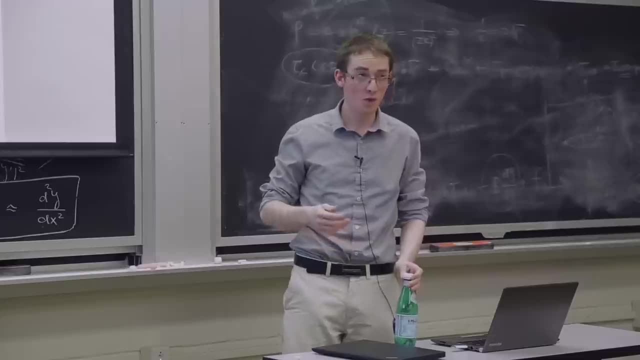 The problem is that the backup large diesel generators are just that: They're large, they're diesel and therefore they're very, very slow to come online and come up to full power. The way that you can bridge this gap is by using the energy that you've stored in the turbines. 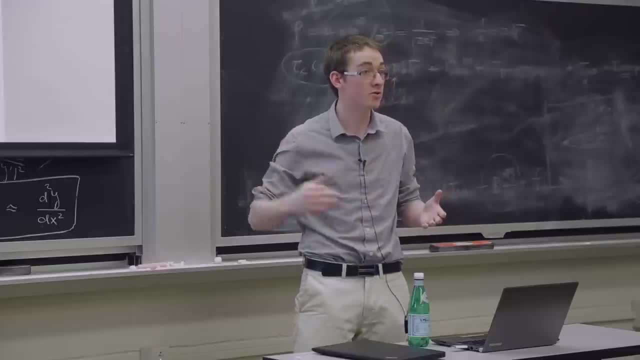 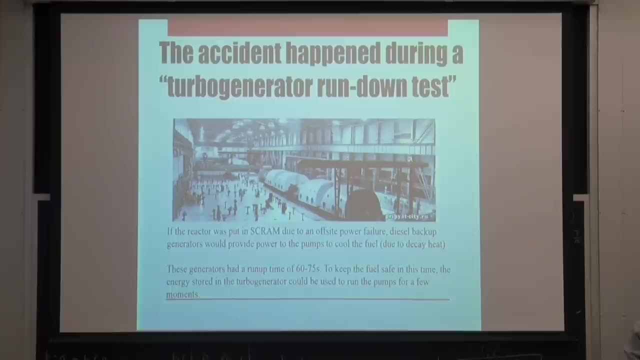 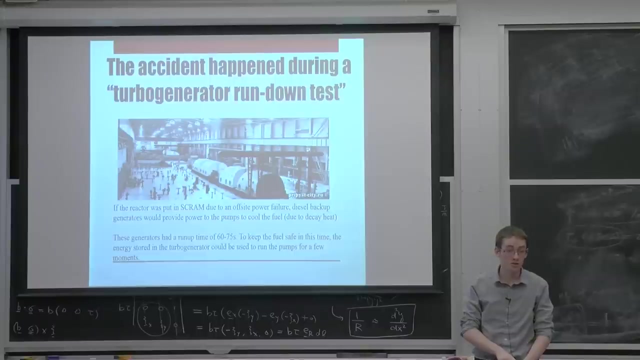 to effectively power the main circulating pumps until the diesel generators can come up online. When Unit 4 was fully constructed in 1983 and turned on for the first time, they had never actually done this test where they did a turbo generator rundown, despite the fact that it was required by law in the Soviet Union. 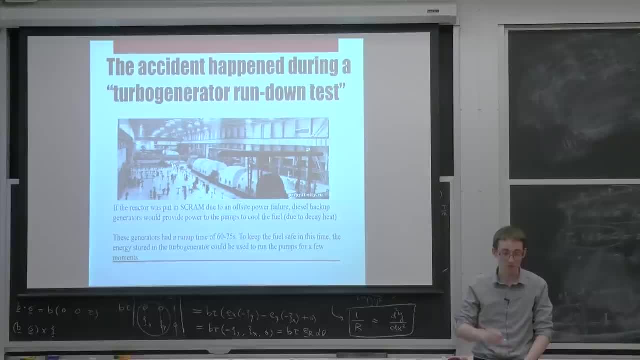 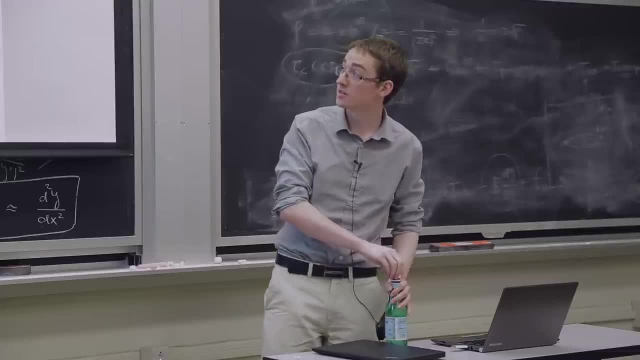 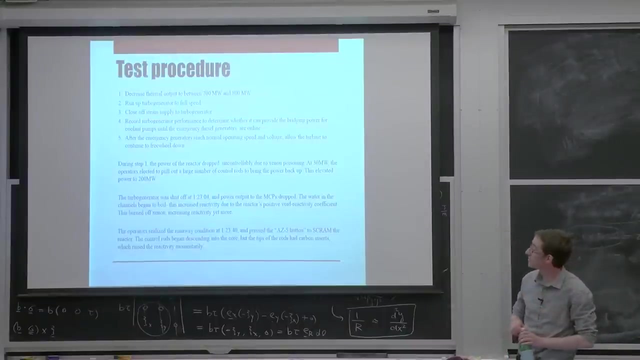 that all new power stations should have this test performed. It was delayed until 1986.. And yeah, it was delayed until 1986, is the long story short. The test procedure- sorry for all the text on this slide- is basically as follows: So you would ramp the reactor down, so you would bring it from a normal thermal output of up to 2,400 megawatts thermal down to 600 or 700 megawatts. You'd bring the turbo generators up to full speed so you'd store as much energy in them as you possibly could. 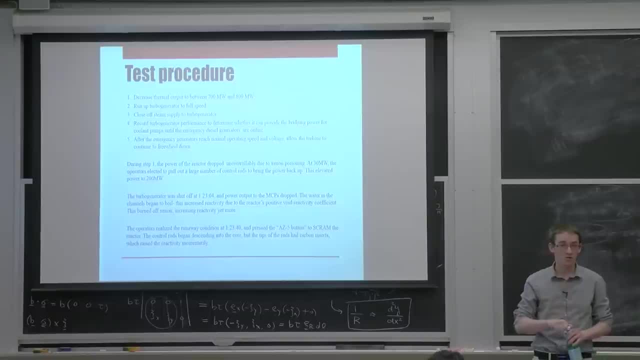 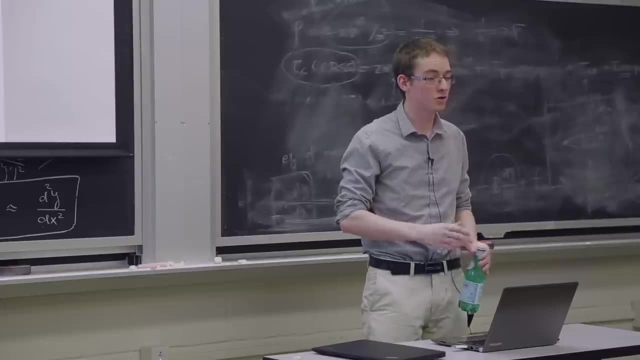 then cut off the steam supply, such that now you are just extracting energy from the spinning turbo generator. This would then be used to power the main circulating pumps, each of which took about 40 megawatts. There are eight of them in total. 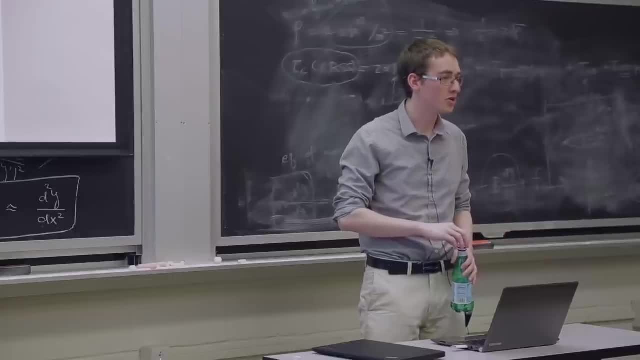 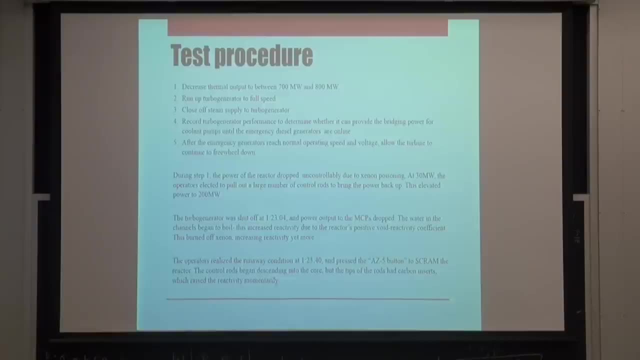 I believe six could be used for normal operation. The rundown would take somewhere in the range of 60 to 70 seconds and hopefully by this time your diesel generators would be turned on pumping water in. everything would be fine. What happened in the test was decidedly quite different from that. 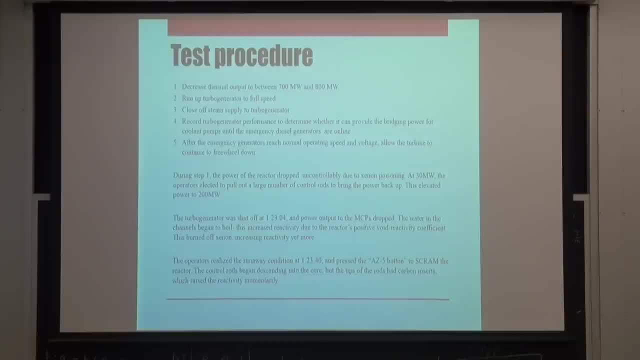 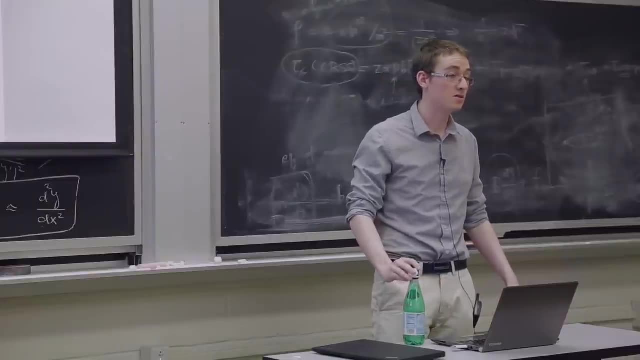 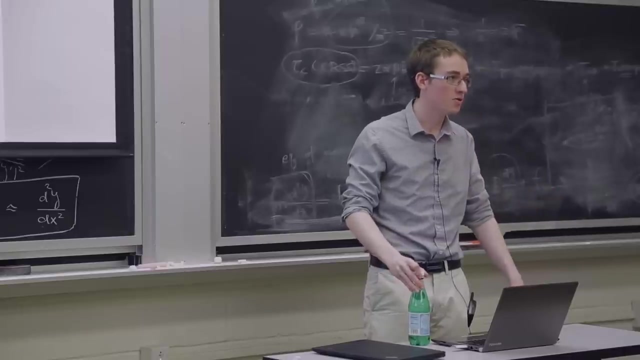 So on April 26th 1986, they attempted to begin this test about six hours behind schedule, because there was an incident in another part of Ukraine in which a coal power plant went offline. So what happened was the authority for the grid in the area. ordered that Chernobyl should stay online at full power for an additional six hours. They began the test by bringing power down, but as a result of running for an extra six hours, they built up a significant amount of xenon precursors in the core. So when they started turning the power down, the power started going down and down and down and they were unable to arrest its drop. What ended up happening was that the power dropped all the way down to 30 megawatts thermal and the reactor operators kind of panicked. 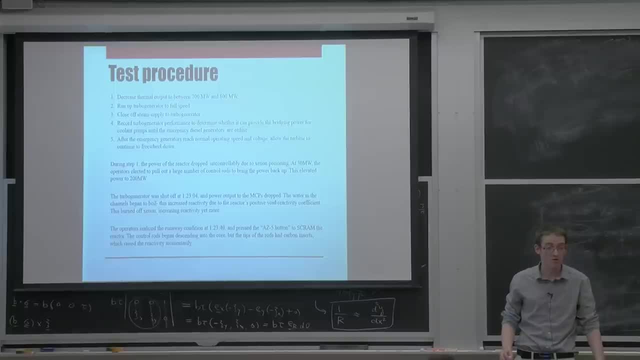 Their response to this, instead of canceling the test, was to pull out as many control rods as they could get their hands on. They did so, and this managed to rescue the thermal output of the reactor, and it bumped up to around 200 megawatts thermal. At this point the reactor was in an extremely unstable state. Mind you, almost all the rods that they could get their hands on were out of the reactor. The only thing keeping reactivity at a reasonable level was all the xenon that was built up in the core. 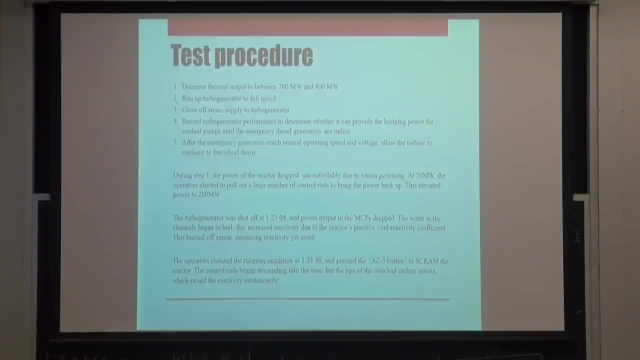 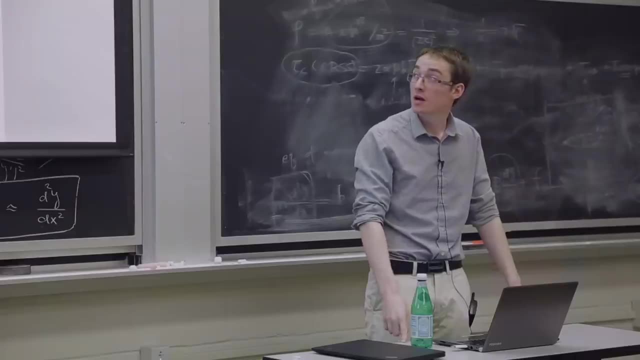 They began the turbo generator rundown test. They shut off steam to the main turbine or one of the turbines after it was run up to full power and then attempted to run the main circulating pump. The main circulating pump started drawing down the energy. 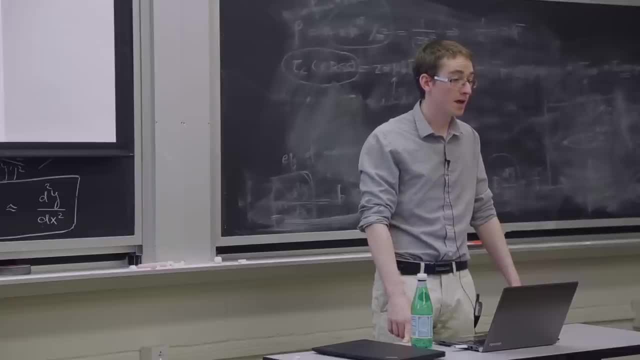 from the spinning turbine and, as a result, it ran slower and slower, meaning that the flow through the core was less and less. more water boiled, going into steam, which increased the reactivity. As a result, the power output of the core went up. 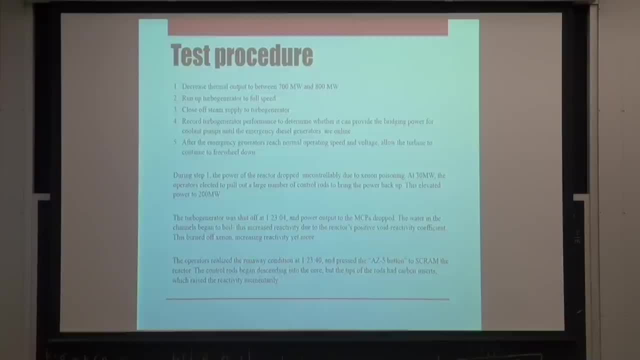 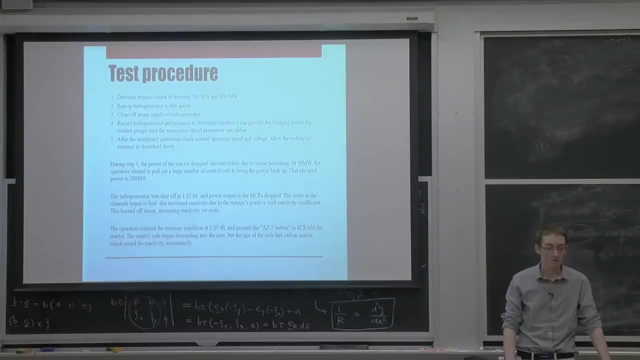 it burned out more xenon and the cycle continued. They noticed a power excursion about 40 seconds after they began the test and at this point recognized they were in bad territory and hit the scram button. This would jam pretty much all of the available control rods into the core. 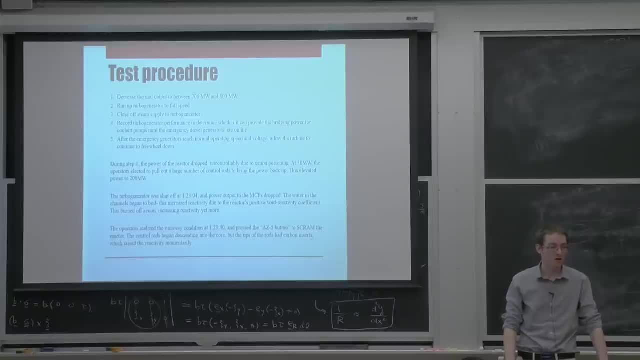 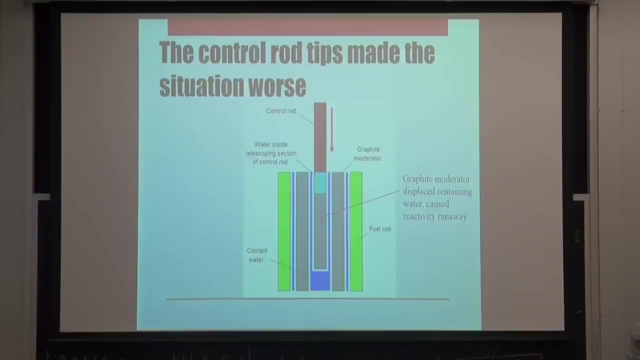 including some emergency extras and shut everything down. In most circumstances this would be a fairly safe move, but in the case of the RBMK it was most certainly not. RBMK control rods have a graphite tip on them. When jammed into the core, they caused a localized power increase. 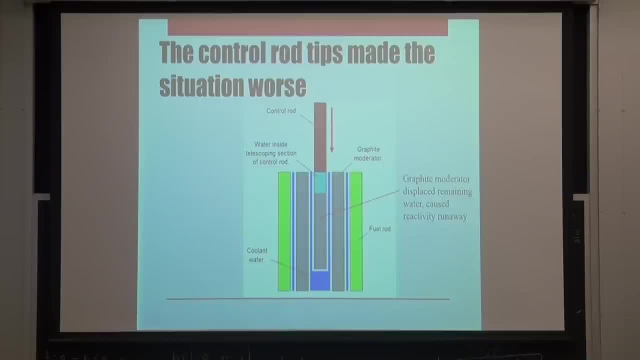 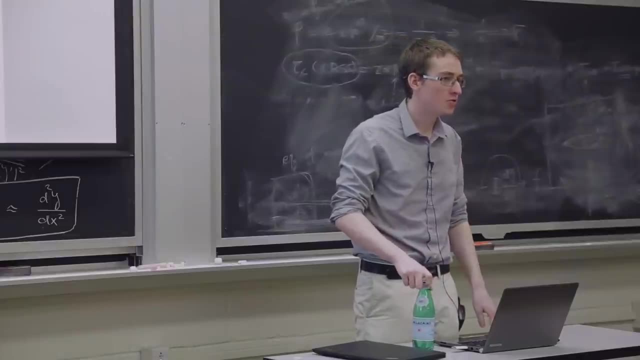 because the graphite is a great moderator and it is displacing water, which is a great absorber, And, as a result, after they made it a couple meters into the core, the increased pressure in the core from the power output, which was localized around the tips of the control rods. 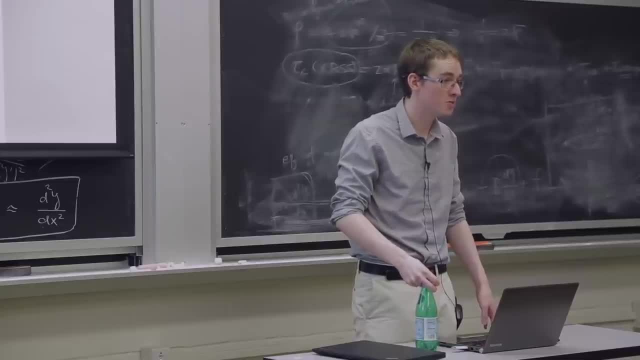 ended up shattering the control rod drive mechanisms and, instead of turning off, the cycle basically just continued. Power continued to ramp up over the next couple of seconds. It eventually reached somewhere around 10 to 20 times the maximum rated thermal output of the system. 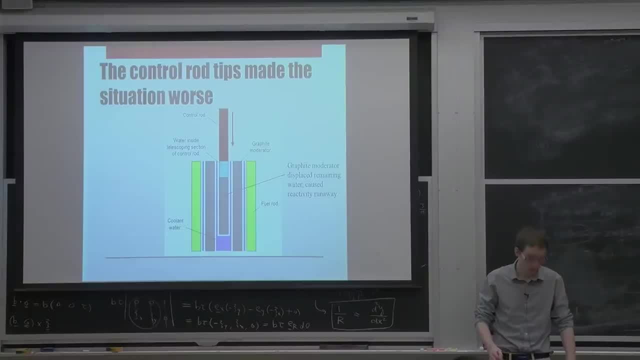 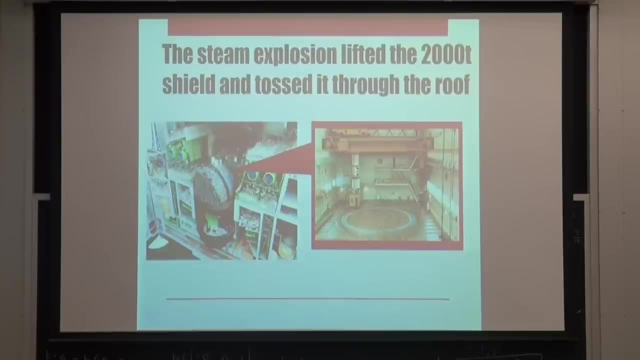 and a massive steam explosion ended up ripping through the facility. It tossed the 2,000 ton biological shield off on top of the reactor through the roof of the facility. It ejected a significant portion of the fuel as well as the moderator in the core. 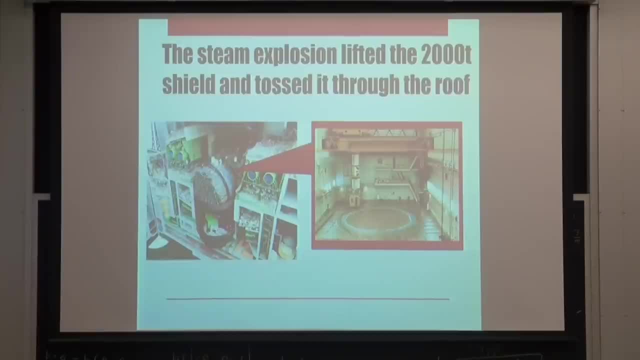 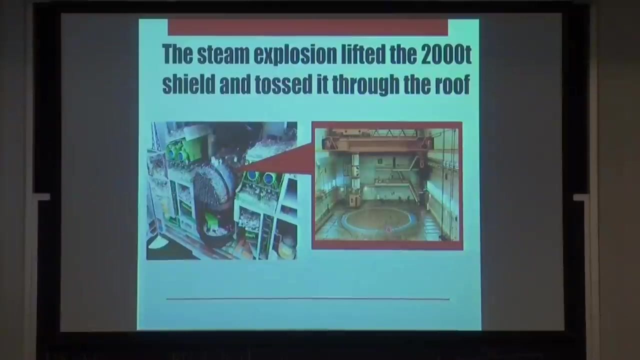 and it started a massive fire around the facility. Just to give you a good sense of scale, let's see if I've got the virtual laser pointer. That's a person right here, this little guy. This is the top of the biological shield, Elena shield. 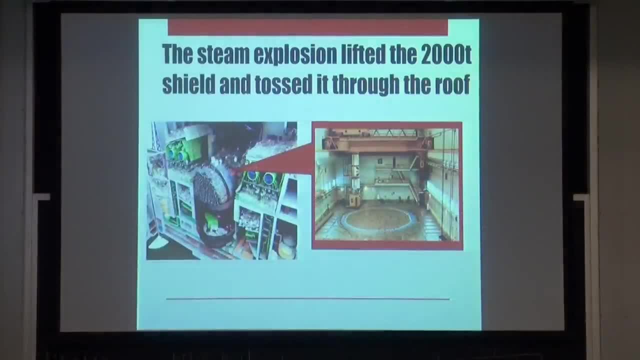 And then this is the top of the biological shield, Elena shield. And then this is the top of the biological shield, Elena shield. This is a model, a cutaway model of the Chernobyl reactor facility, with the shield, with the flipped shield. 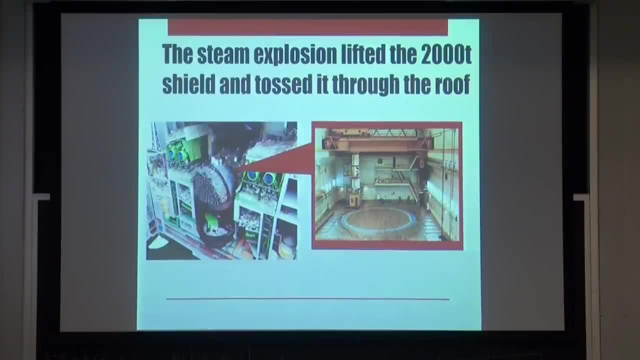 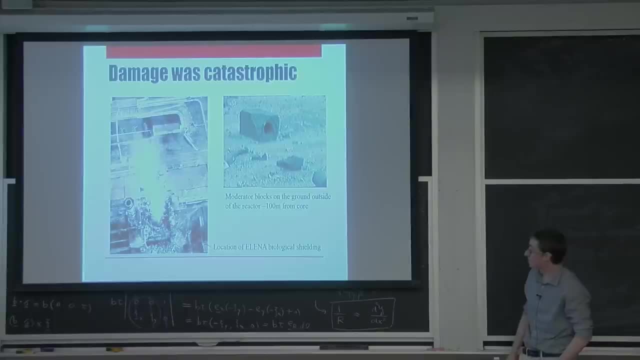 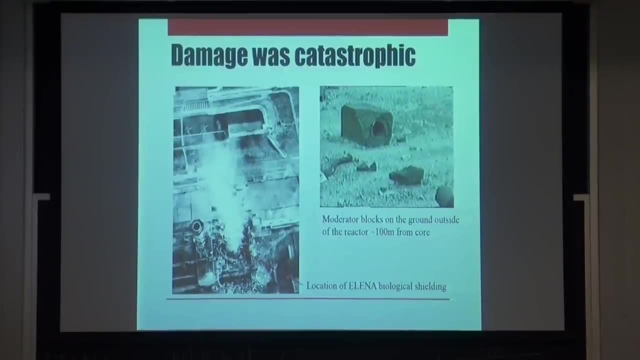 that went up through the roof and came back down. So, as you can see, it was an utterly massive explosion. So the damage to the reactor was immediately quite catastrophic. Moderator blocks- Fuel was spread all around the immediate area. If you look in this photo, it's rather difficult to see. 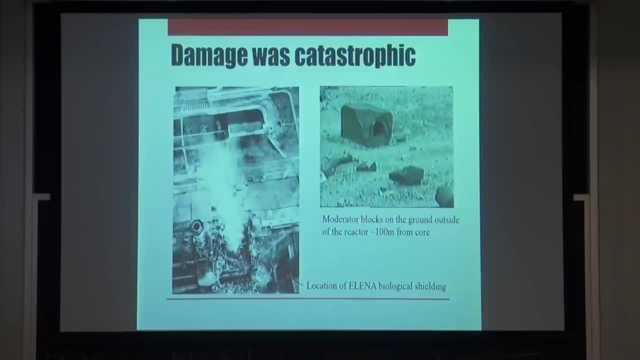 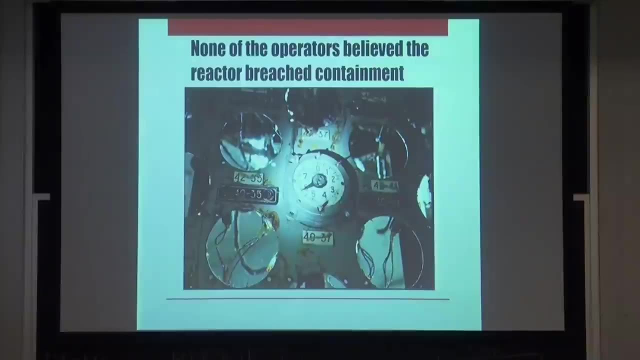 but at the bottom of that column of smoke you can actually see the bottom of the biological shield. Kind of gives you a sense of the scale of the damage to the reactor. After the explosion happened, actually none of the operators believe the reactor breached. 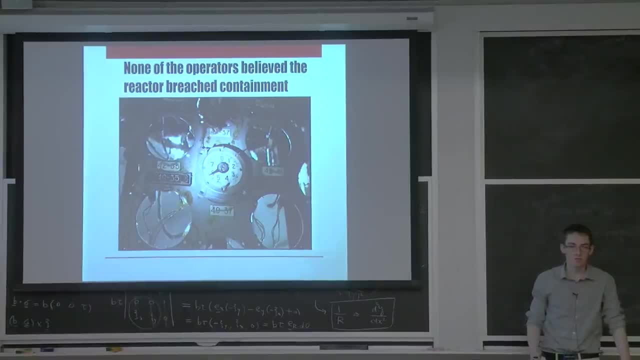 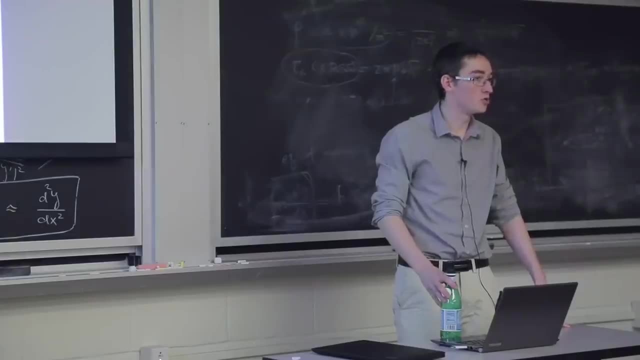 confinement in any way. They didn't really have an immediate way of seeing what had happened, So they opened the door and went to the main turbo generator building to investigate the damage. They believed it was perhaps one or two ruptured fuel channels, As it happened at, I believe, the Leningrad. 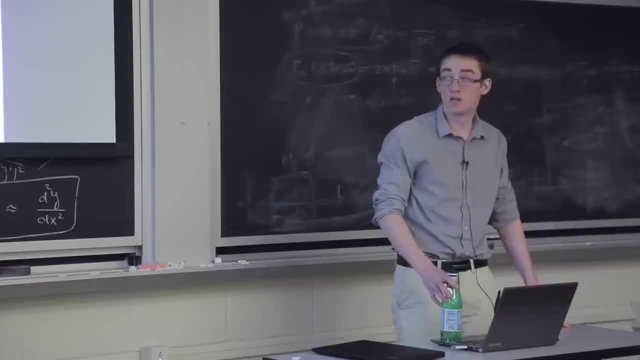 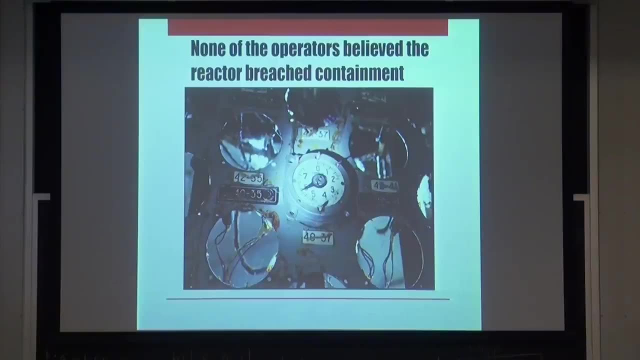 I think it was the Leningrad power station a few years earlier. in the few seconds that they were there, they received fatal doses and died in the hospital in May of 1986.. This is a photo from control room of reactor four. 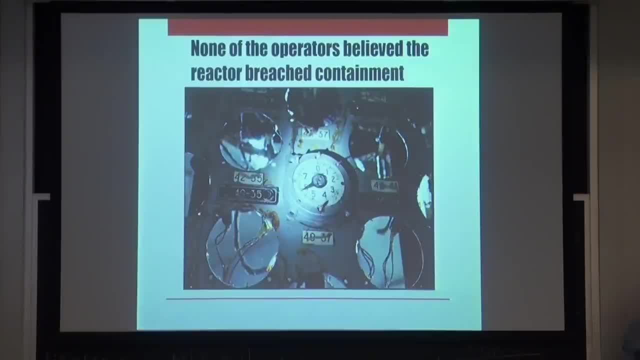 showing a jammed control rod drive at the six meter position. So this was probably a rod. let's see, this was probably a rod coming up from the bottom, in that it- yeah, seven meters would be all the way out, zero meters. 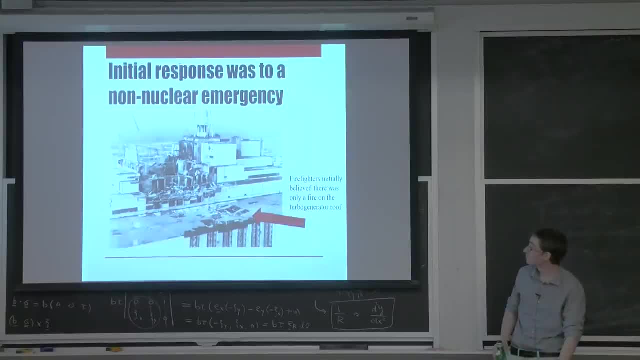 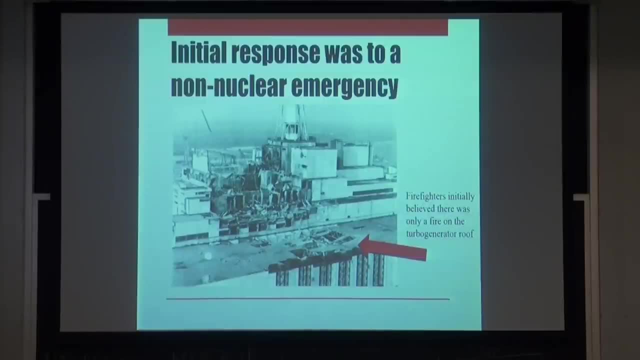 Zero meters would be all the way. in The initial response to this, despite the fact that the reactor operators, who were not yet dead, did realize that it was a full breach of containment, the response was to an accident that was non-nuclear in nature. 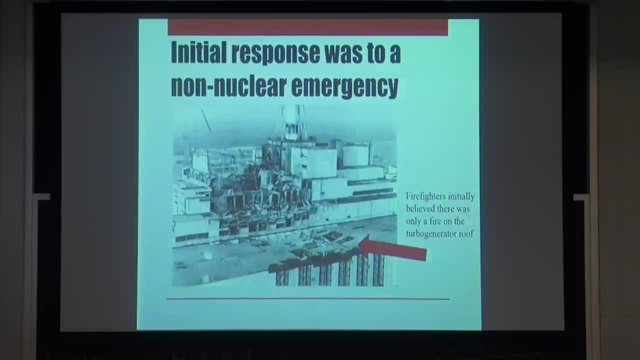 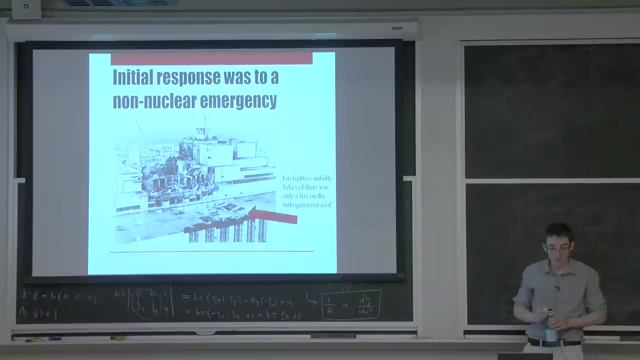 So when the fire department got a call from the authority at Chernobyl, the message that they received was: there's a fire at the reactor complex. As a result, what they showed up with was not equipment suitable for a hazmat situation in any way. 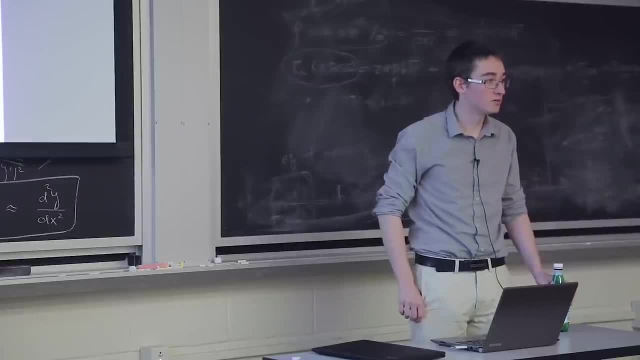 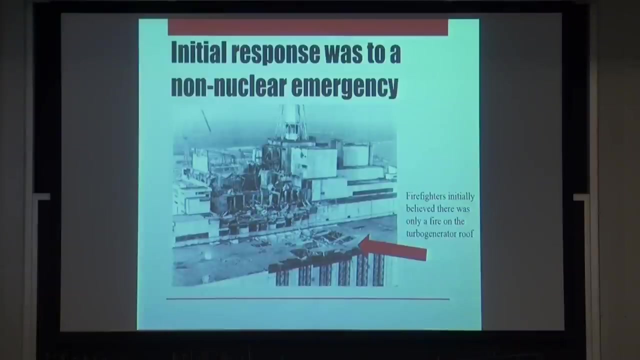 That said, there's pretty much nothing that could shield anyone from the extremely high radiation field that one would encounter around the reactor in the immediate aftermath of the accident, But nonetheless they were extremely vulnerable. It was night when this accident happened. As I mentioned, this happened at 1.23 in the morning. 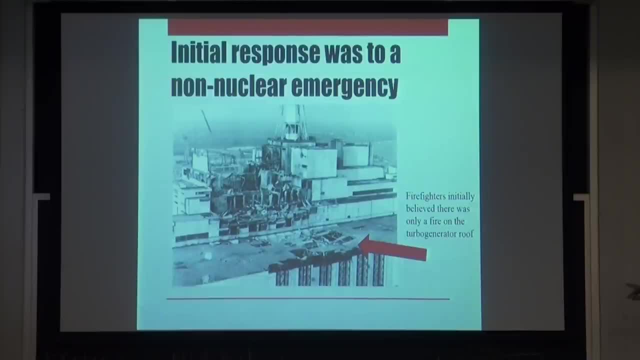 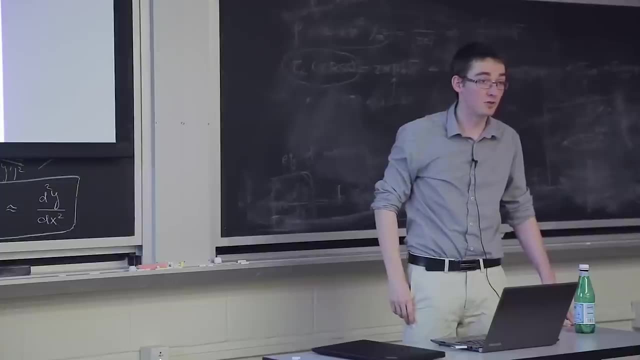 They actually couldn't see. They couldn't see the extent of the accident And they initially believed that it was just a fire on the roof of the turbo generator building. They attempted to fight the fire And some of them actually succumbed to acute radiation poisoning or acute radiation syndrome. 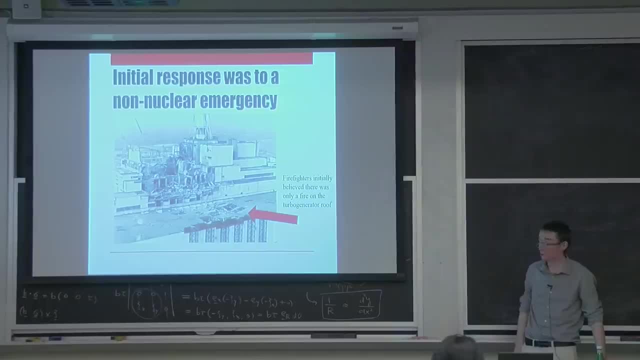 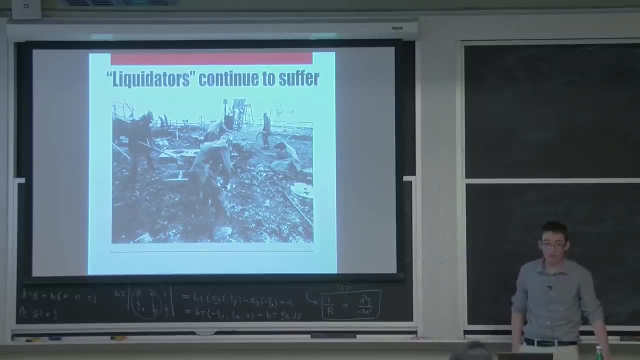 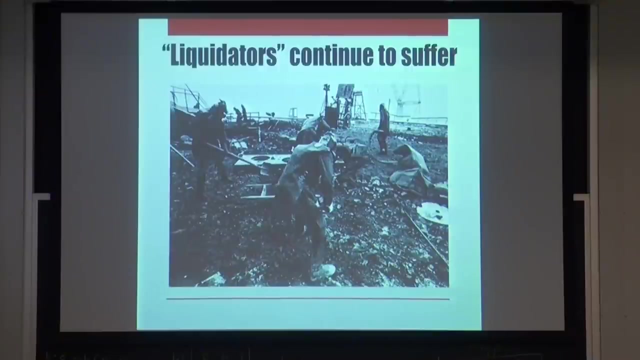 almost immediately, A number of firefighters went up on the roof and just didn't come back. The aftermath of the accident, the cleanup was handled by the Soviet army. The people that were involved in this were known as the liquidators. They would spend several minutes on the rooftop. 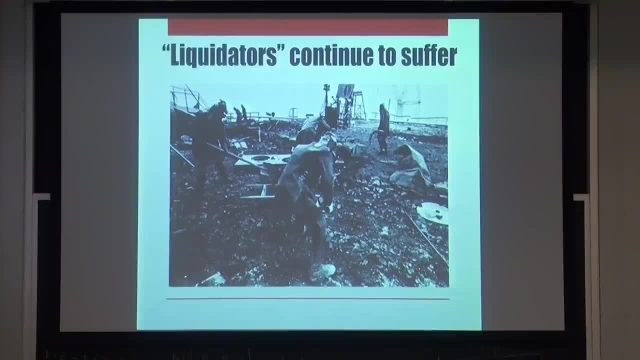 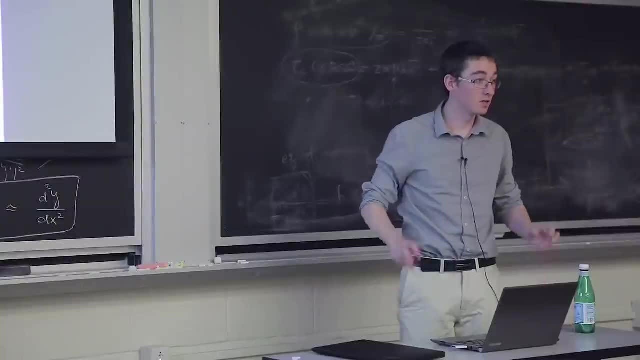 of the turbo generator building or up near where the reactor was, the reactor containment building was, And they would receive effectively a lifetime dose, which I believe their limit was 50 rem, And that would be a couple of minutes up there. Let's see. 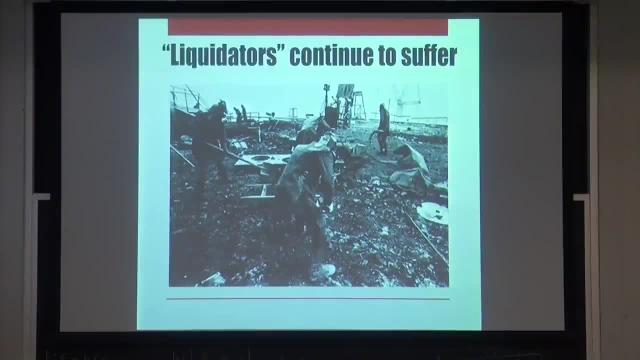 This photo doesn't show much evidence of it, but I suppose it shows a little bit of evidence of it. If you look around the bottom of the frame you can actually see a little bit of hazing in kind of a periodic fashion. Let's see if I can get my pointer on it. 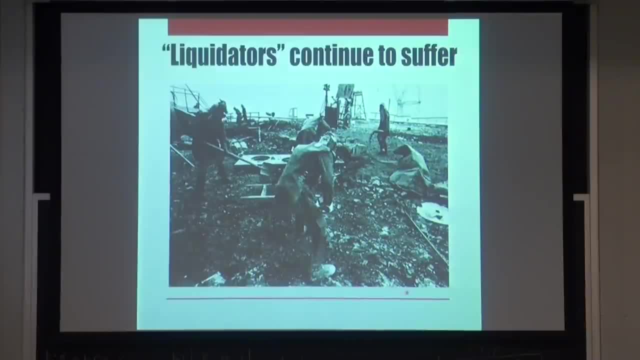 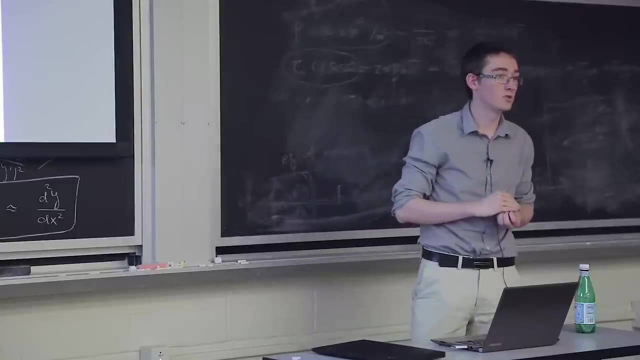 Here, here, here, here and here- That's the gear that moves the film- is actually shielding the film from radiation exposure. at those points The radiation dose rate was so high up there that most of the pictures that were taken just didn't turn out. 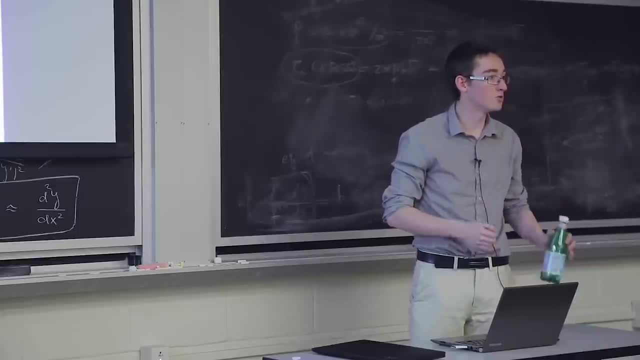 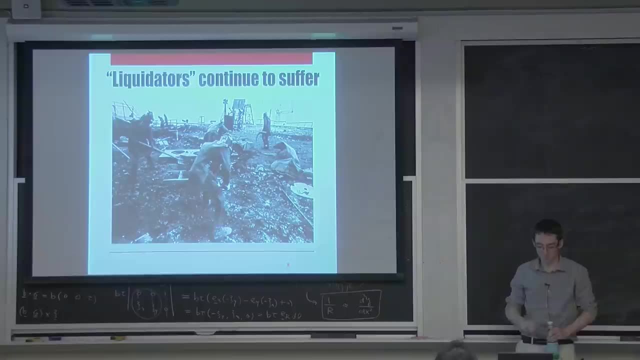 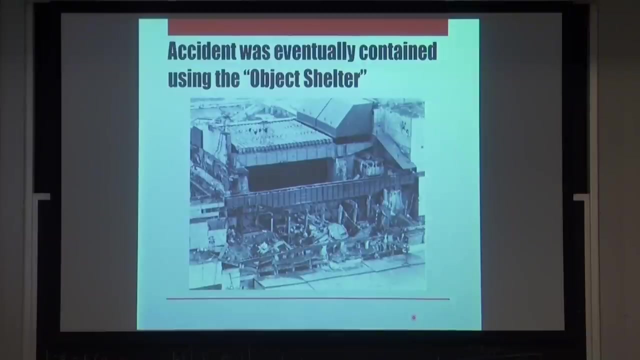 A few smarter photographers used a whole lot of lead and were able to capture photos like this, But nonetheless the dose rates were tremendous. The reactor structure itself was entombed in this thing that we call the sarcophagus. People in Ukraine call it the object shelter or the shelter object. 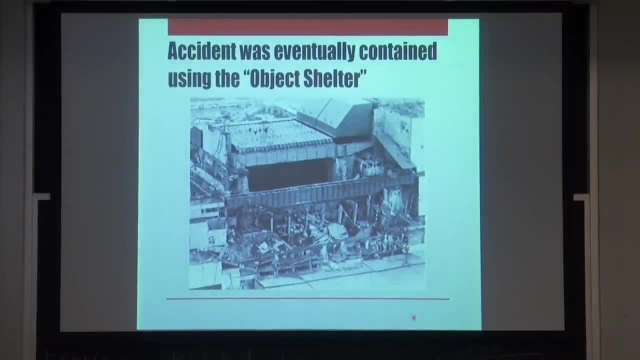 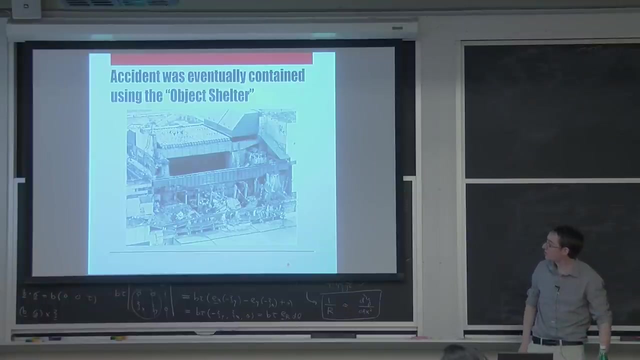 It was constructed in starting almost immediately after the accident, basically to keep radioactive graphite and fuel fragments from leaving the reactor structure and contaminating any more land. This is a photo from when it was under construction. Basically, what it consisted of were steel and concrete walls. 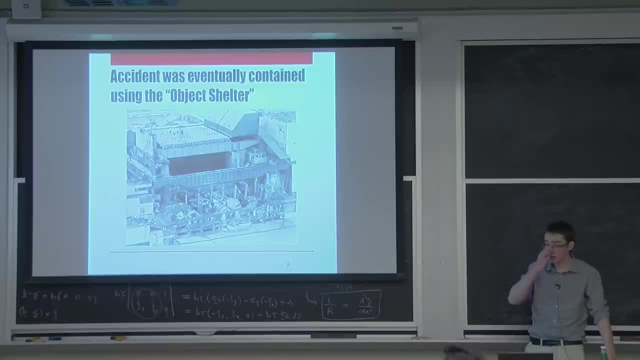 that were erected around the reactor using a variety of technologies. They at first attempted to use robots that were almost immediately rendered useless by the high radiation field. Later on, they ended up using- quote- bio robots- people to move things into place. 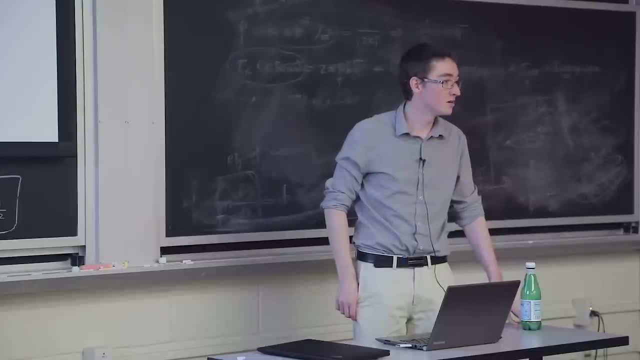 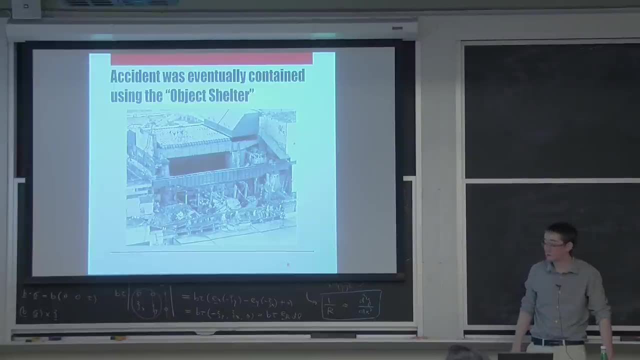 As I've said before, a whole lot of people died in this accident, both immediately and after many, during the construction of the sarcophagus- Actually during the initial firefighting measures, as the core remained burning for a number of weeks after the accident, they attempted. 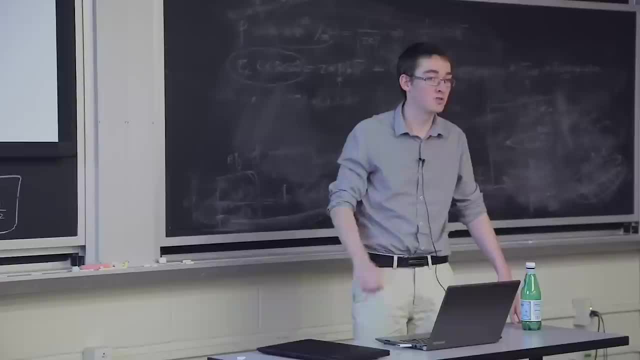 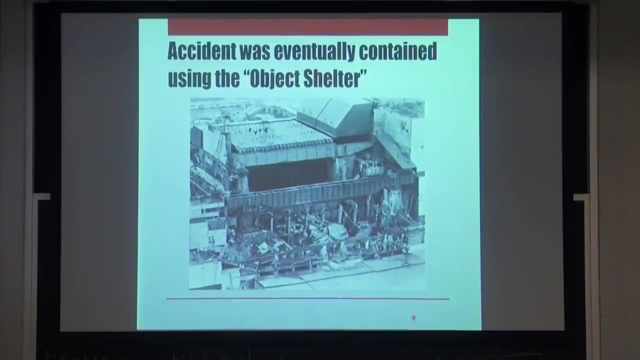 to put it out with bags of sand dropped from helicopters, And during that effort, a helicopter actually ended up hitting one of the cranes that they were attempting to use for this and falling into the reactor, And a good portion of its remains remain entombed. 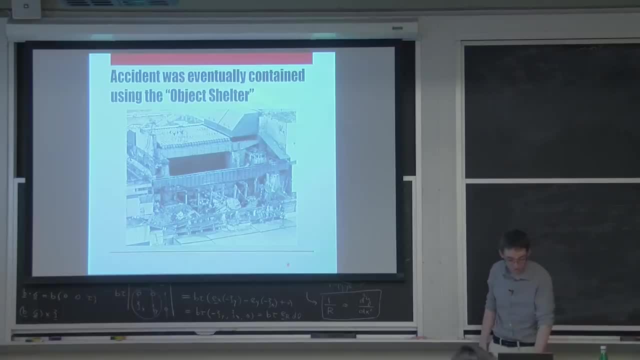 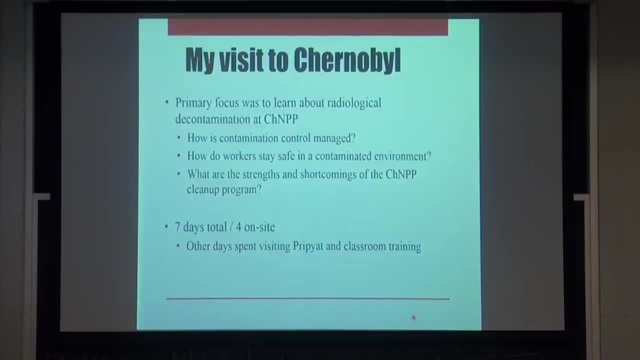 within the sarcophagus, from what I understand, All right. so my visit to Chernobyl. Why would anyone ever want to go there? The primary focus was to learn about radiological decontamination at the site. Basically, how is contamination control managed? 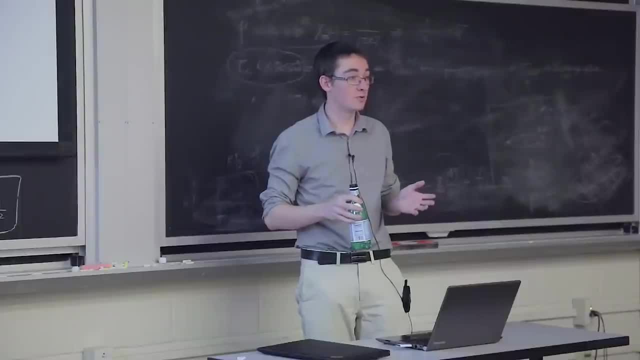 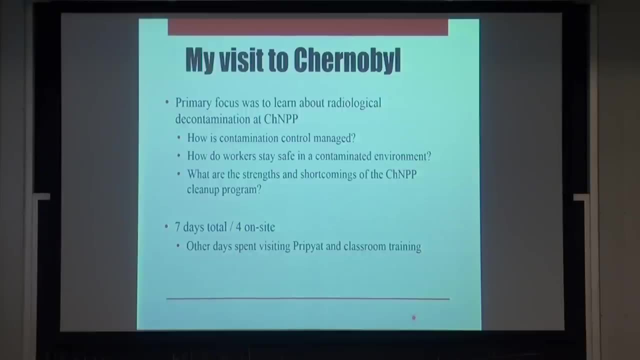 How do workers stay safe? Mind you, there are 3,000 people that go to work there every day, And what are the strengths and what are the shortcomings of their radiological program? It was seven days total, four of which were on-site. 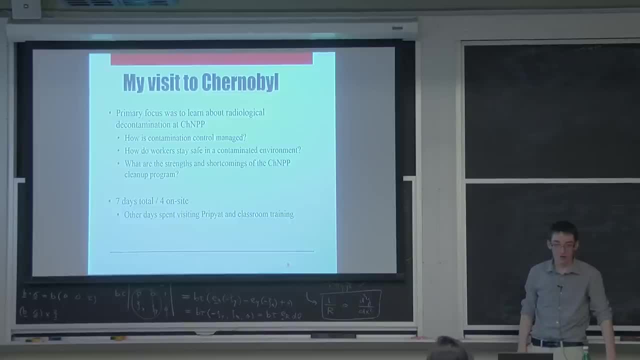 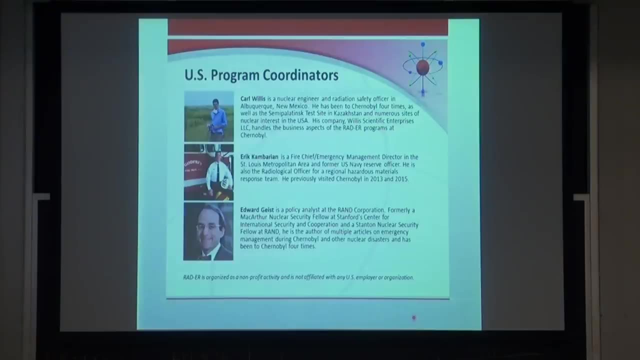 Other days were spent in Pripyat, as well as in some classroom training, which I've got great photos of, So this is a slide stolen directly from the PowerPoint that I was sent on day one, But this was organized by three people. 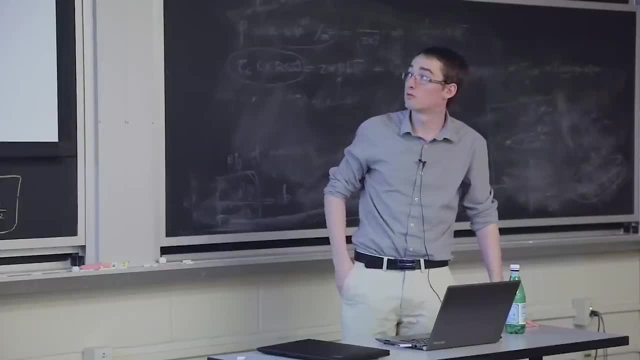 Carl Willis, Eric Cambarian and Ed Geist. I've known Carl for a few years now. He lives in Albuquerque, New Mexico, and is a radiation safety officer at a company that I think they do advanced energy storage technologies. 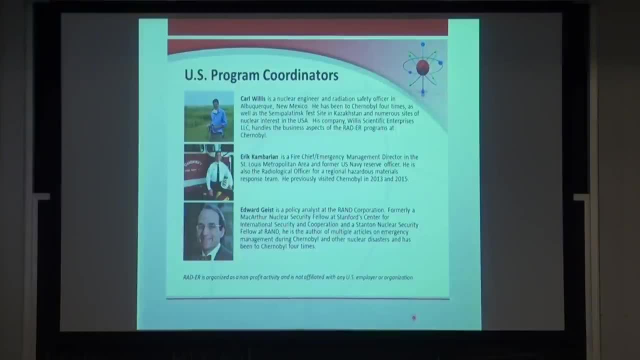 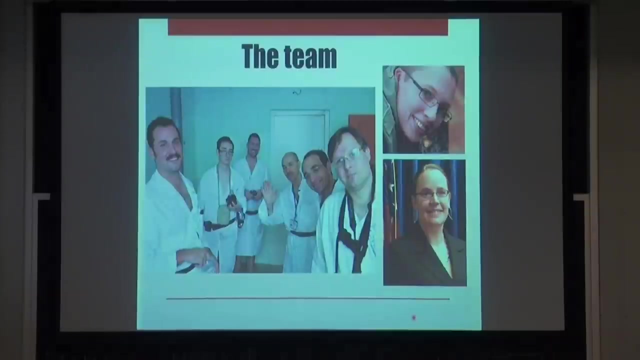 I'm not exactly sure. Eric is a firefighter and specializes in radiation emergency response, And Edward works at the RAND Corp and does nuclear history and nuclear security research. This is the team this year. So we've got. let's start here. 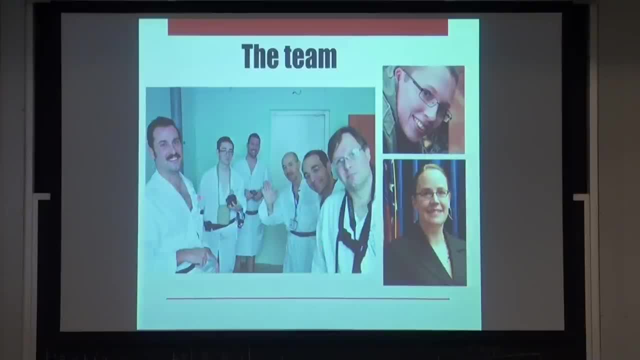 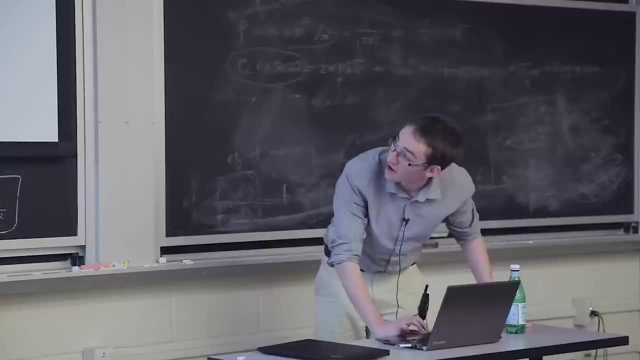 This is Lucas. He does environmental radiation monitoring. That's me, after having no sleep because I did a 22-6-11 p-set the night before. I know I look so happy to be there. This is Nathan. Nathan builds organs as in the musical instrument. 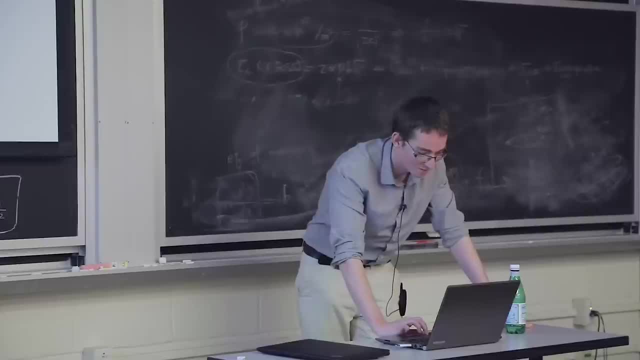 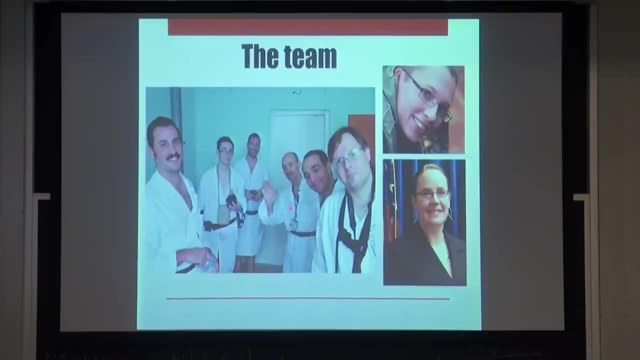 He was along, because he was working along, because he's always been interested in Chernobyl but didn't really have any experience in the field. This is Stanislaus. Stanislaus was our guide from the Chernobyl Authority. He's been working at the plant since 1991. 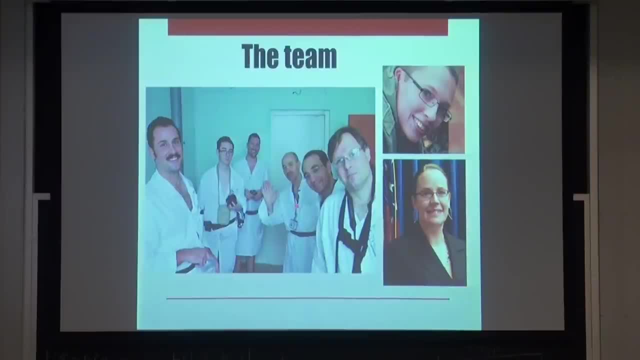 and is a fantastic resource for information. This is Ed, who I believe I talked about earlier. This is Ryan Pierce. I'm not really sure what he does. This is Iris, who is a friend of Carl's and works in, I believe. 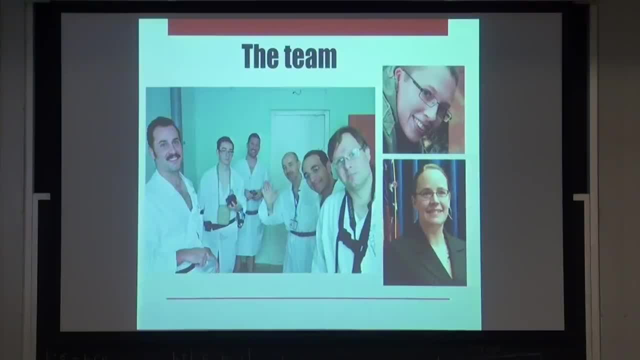 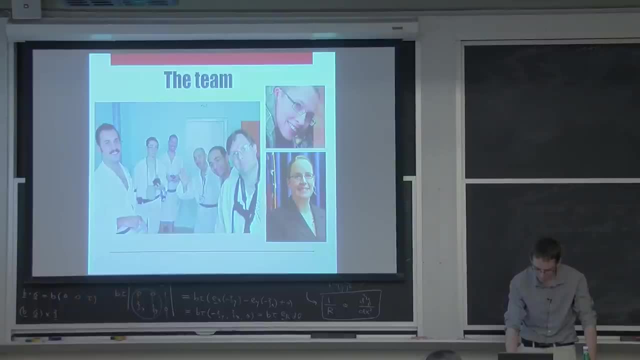 radiation oncology. And then Danelle Hogan, who's an educator based in Phoenix, Arizona, who works with the DOE. By the way, if you're wondering why we're all wearing those absurd robes, it was before we were going to go into another. 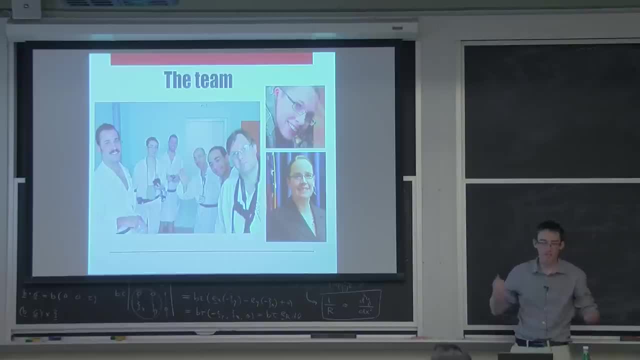 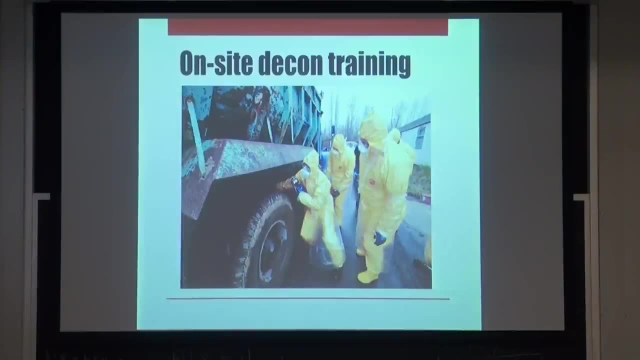 room and change into basically coveralls which are easy to decontaminate. One of the activities that we did was real decontamination training. So that is a truck. This is a truck from the Novarco worksite which, by the way, 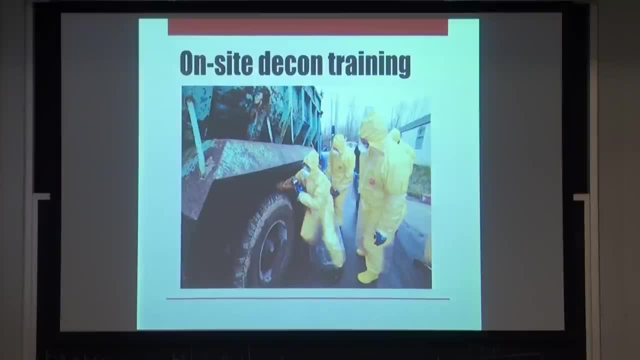 that is me with the Geiger counter. I'm surveying for contamination. We then pressure washed the truck. As it turns out, there's a very specific technique one needs to use for pressure washing when you're dealing with a contaminated object, so as to not blast contaminated dirt. 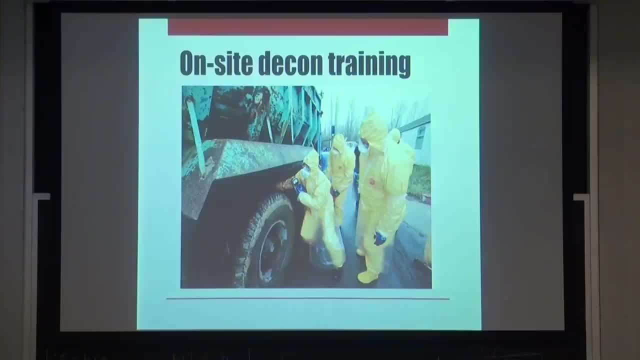 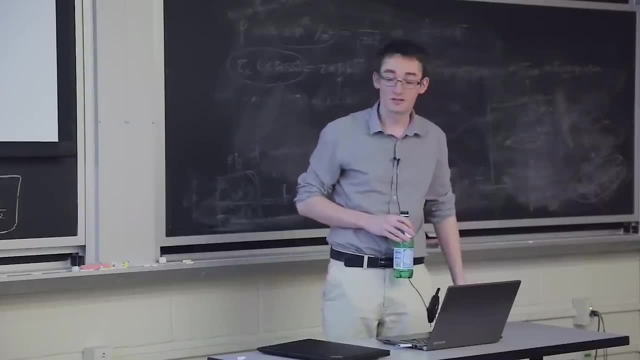 up back onto the truck. This was a very interesting experience and also one that was very entertaining for the workers involved, because they don't actually wear that When they're doing decontamination, because their respect for safety protocols are, shall we say, a bit. 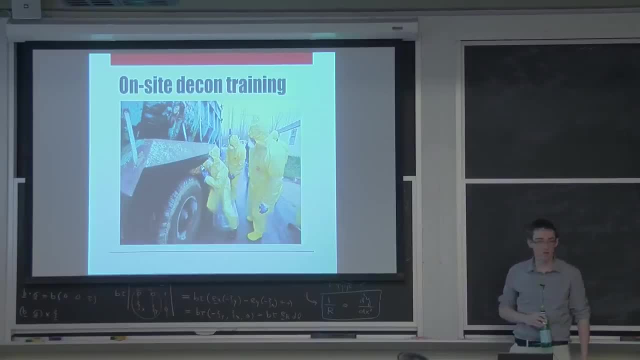 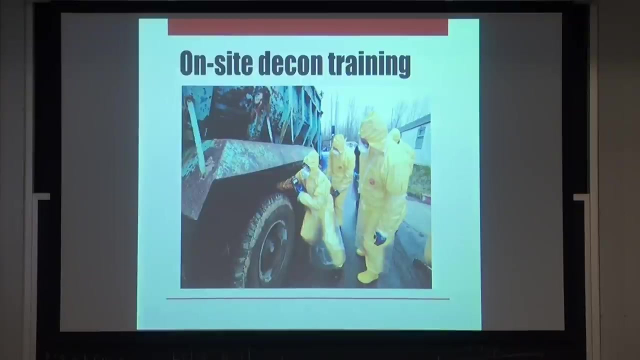 different. So they got to see us wear the absurd rubber ducky suits while they stood by smoking and laughing at us. I believe you can actually see the corner of that guy's jacket back there. He's just wearing everyday clothes. We also went on the New Safe Confinement worksite. 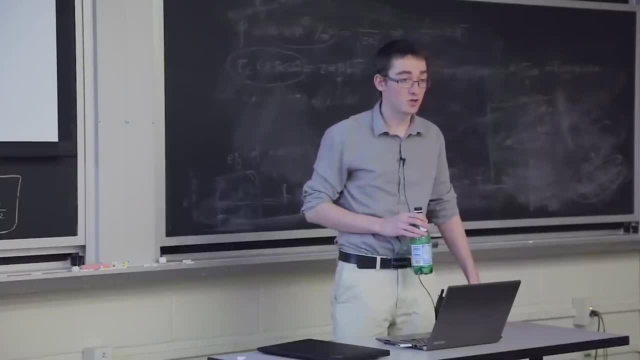 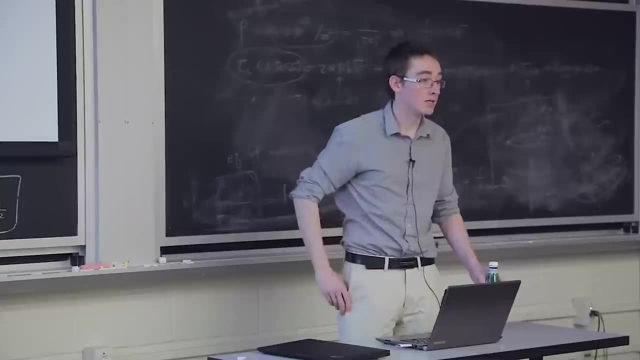 So I haven't talked about it earlier in this presentation, but I suppose I should have. There is an object called the New Safe Confinement arch that consists of basically a giant stainless steel structure on rails which is being slid over reactor 4,. 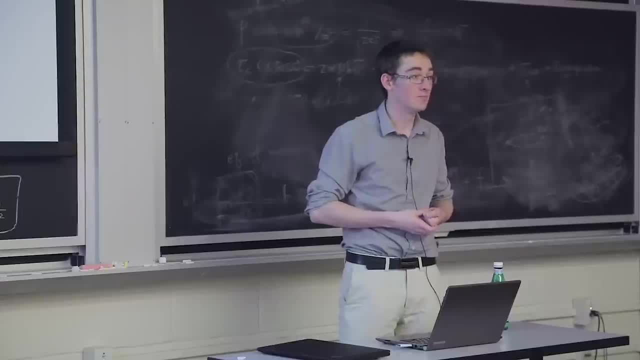 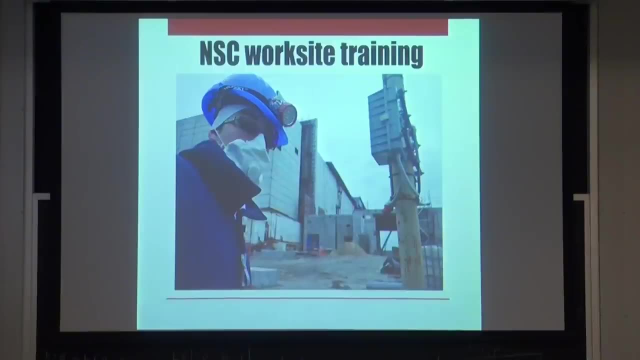 so as to prevent the spread of any sort of contamination from it. This is known as the New Safe Confinement or NSC arch. It's been under construction since 2007, and it just- and it just moved for the first time, actually, while I was there. so, on the 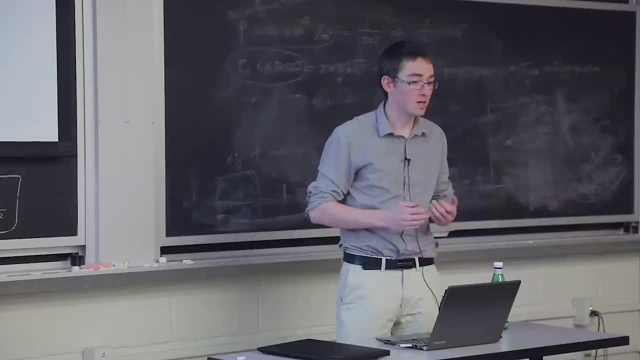 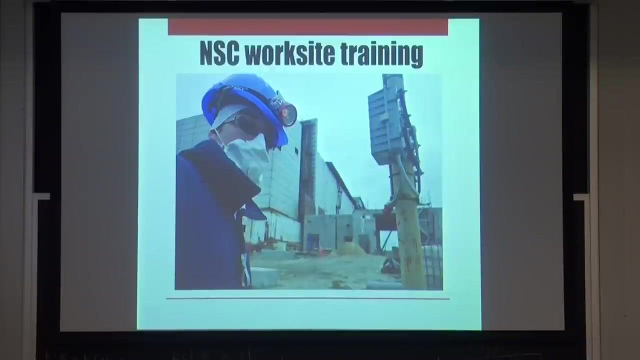 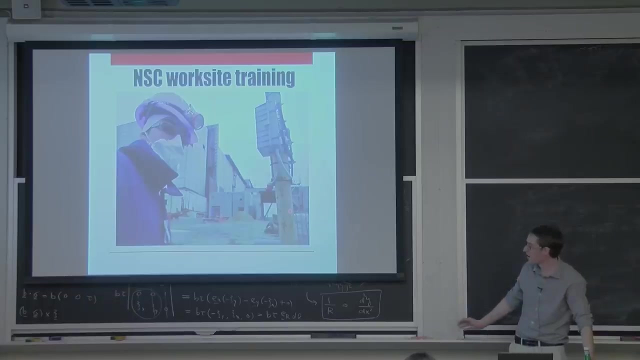 12th of November. it's supposed to last for a hundred years and hopefully in that kind of time span they'll be able to take apart what remains of the reactor. so actually, what you see here is the corner of the sarcophagus, and then, if you were to pan over this way a little bit, you'd see the right set of 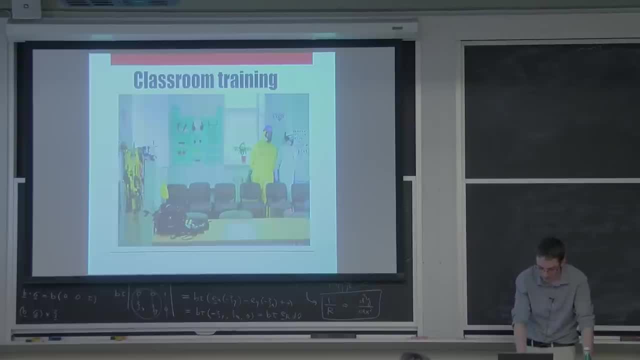 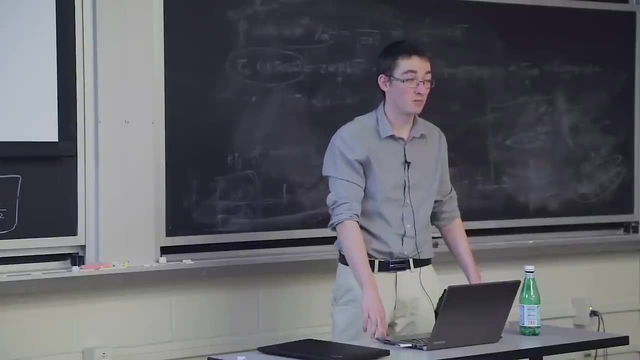 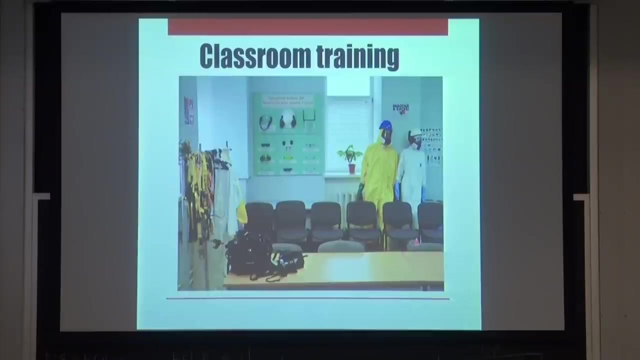 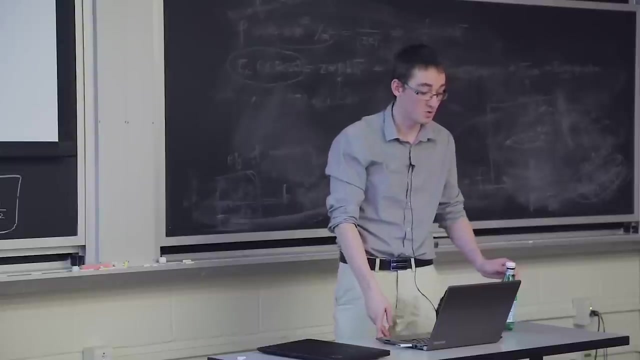 tracks for the new safe confinement arch. we also did some classroom training. admittedly, the classroom training was the most disappointing part of this. the instructors were not particularly interested in showing us really anything other than YouTube videos and other things. that would just waste our time here. That was. that was the one part of this trip that I did not enjoy, regardless, we 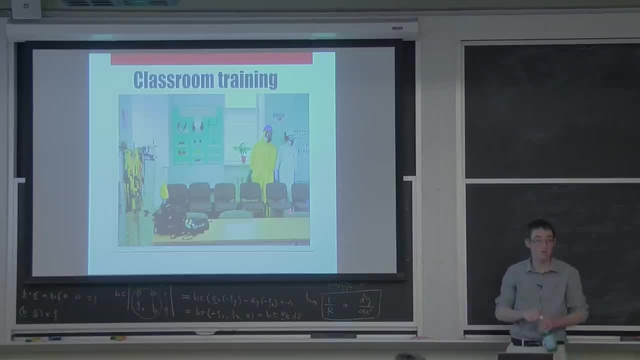 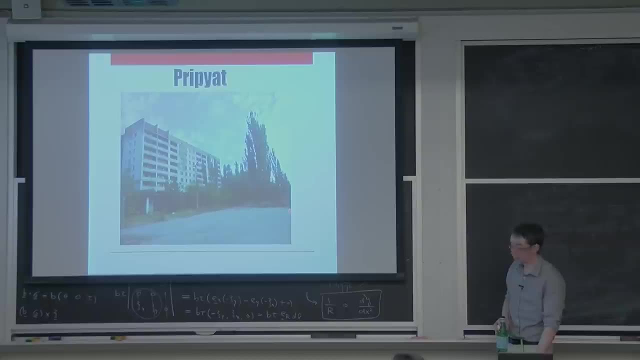 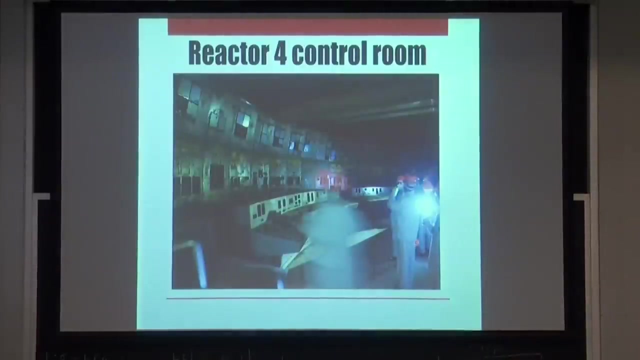 did get to learn a little bit about the various hazmat get-ups that folks would wear when working on site. as I mentioned, we also got to visit Pripyat, which I have more photos of later, as well as the reactor for control room, which is inside. 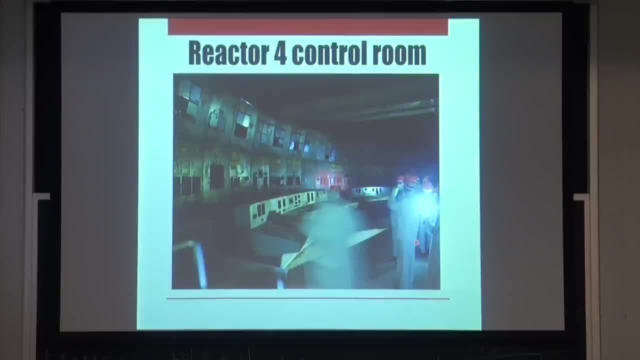 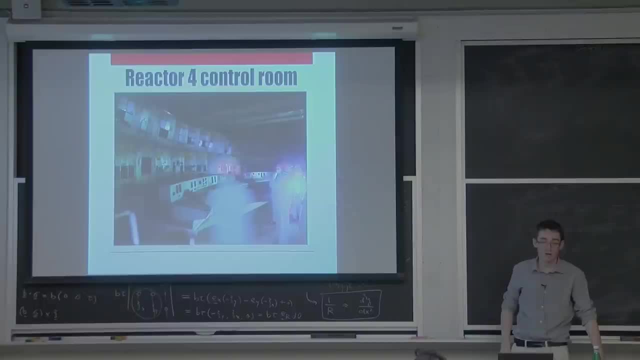 the sarcophagus, which is quite a treat to visit the reactor for control room, is not terribly contaminated as a result of decontamination efforts during the accident. the dose rate would have been somewhere in the range of five to ten rem an hour, but today it's in the range of 10 m rem an hour. this is the 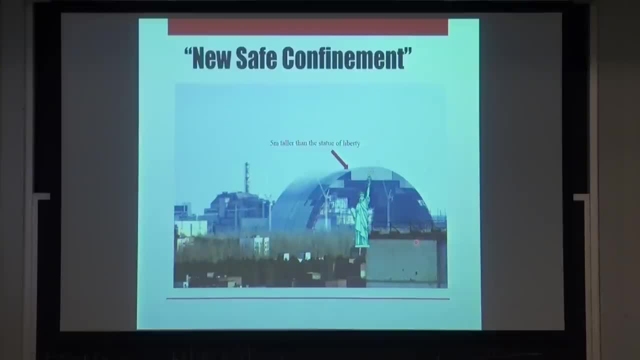 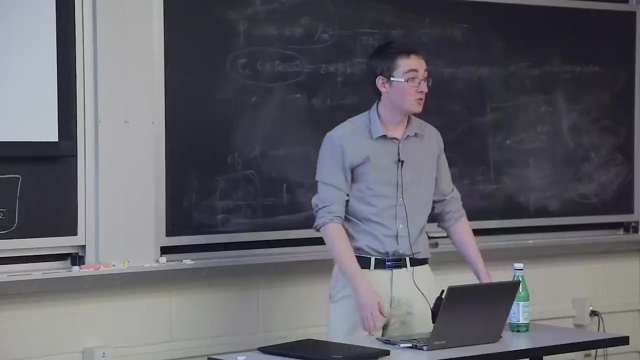 new safe confinement arch that I've been talking about. this is actually a photo from 2015 with a clipart Statue of Liberty on it, but to give you an idea of how huge it is, you know, five meters taller than the Statue of Liberty And it's on rails, which is interesting. it's actually too big for wheels, so it's. 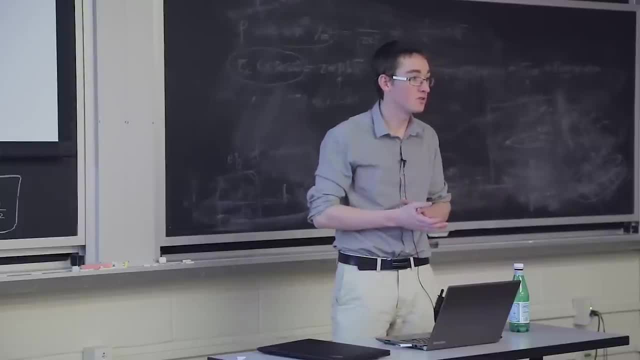 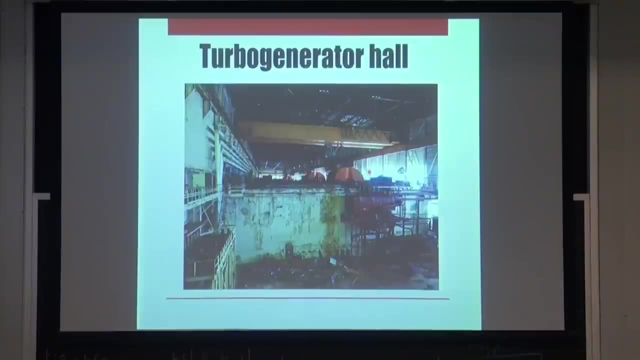 not on rails like with wheels on them, it's on rails with giant Teflon scoots. This is the inside of the turbo generator hallway. remember that long building that I showed you: the connected reactors one and two, and three and four. this is right outside. 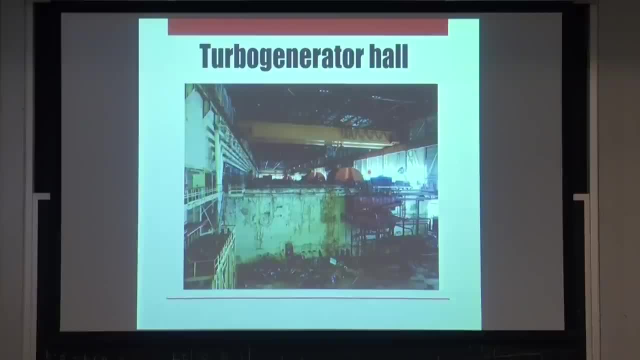 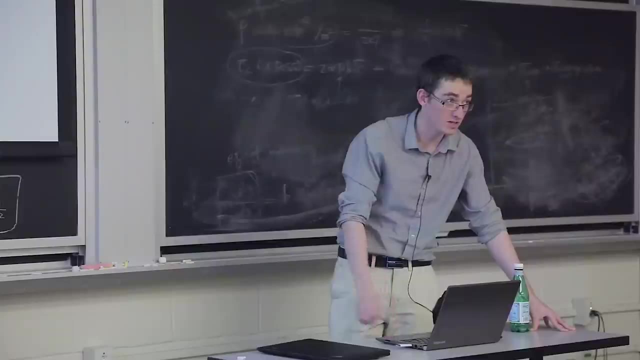 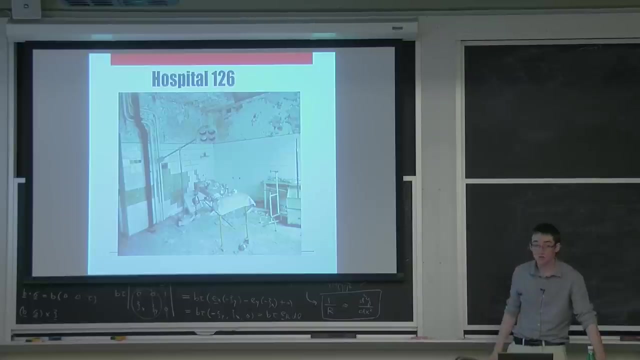 the reactor three. part of it. there are, I think I'll show you these photos later. there are chunks of the turbine from reactor four that are down here in this area that are quite visibly radioactive and are very easy to detect if one swings a Geiger counter about Within Pripyat. we also visited a hospital, 126, which is where 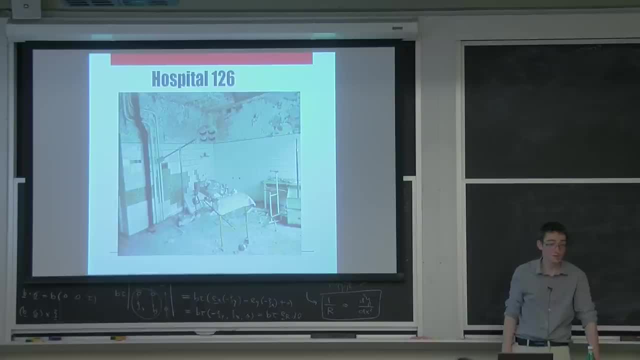 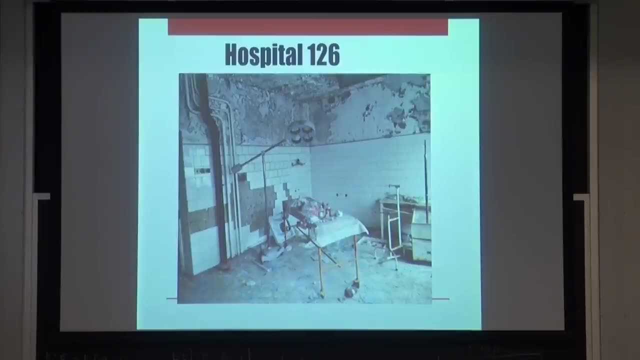 the firefighters went immediately after the accident, that is, the ones that made it off the roof. This garment here- we're not exactly sure what it was because none of us were going to really touch it, but we think it might have been part of a cover that would go under one's helmet- was extremely radioactive. It was contaminated. 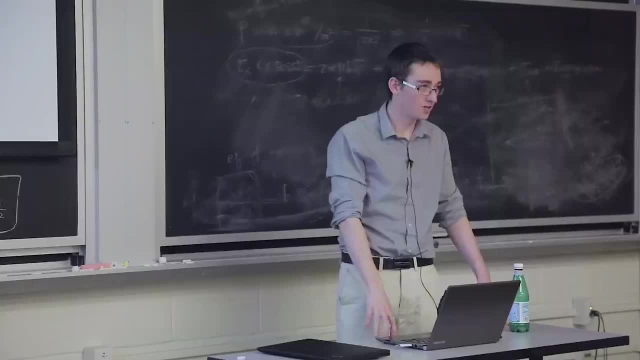 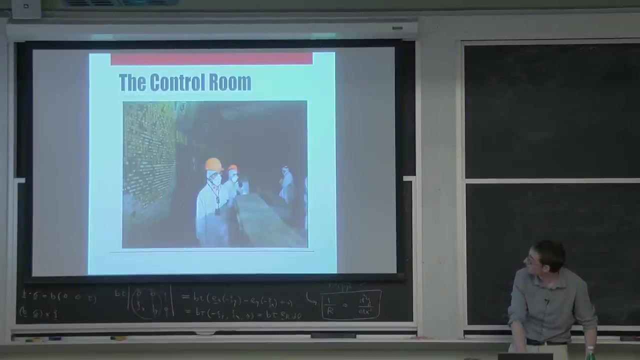 with alpha, beta and gamma, which is fairly unusual. Alpha contamination is fairly rare around the Chernobyl site and was somewhere around 50 to 75 mR an hour on contact. I think I already showed you photos of the control room, Yep. 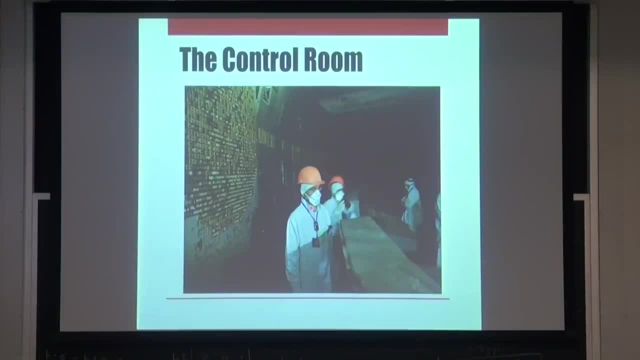 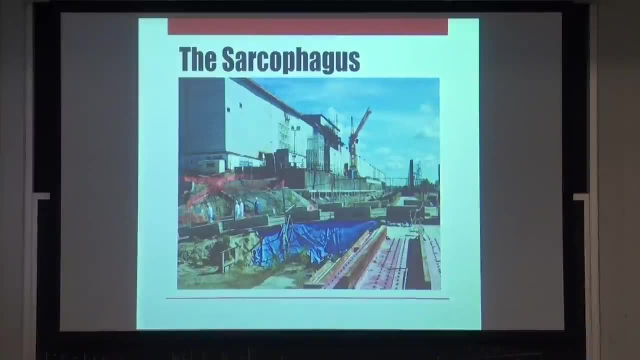 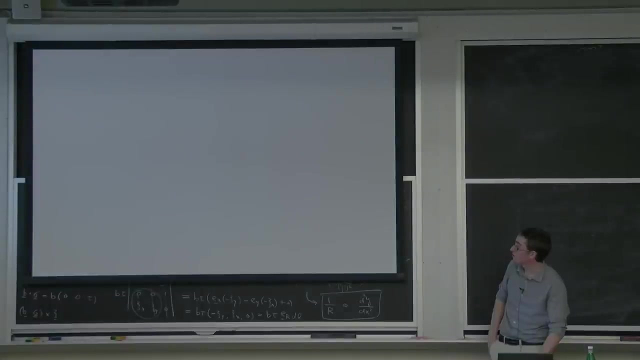 Unit four. This is a diagram that would display various parameters of the reactor for each fuel channel, depending on how one configured it. That's an external photo of the sarcophagus, and I think that that's it for the PowerPoint slides. I do have a bunch of photos, though, that I 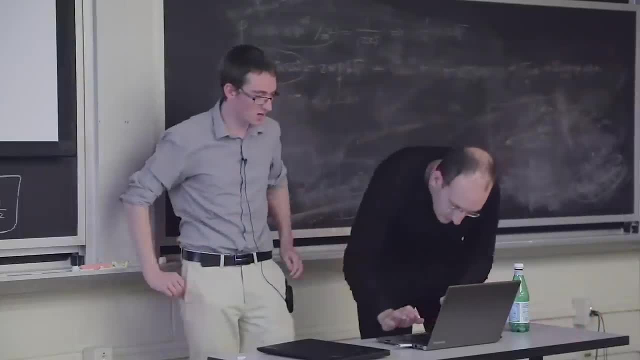 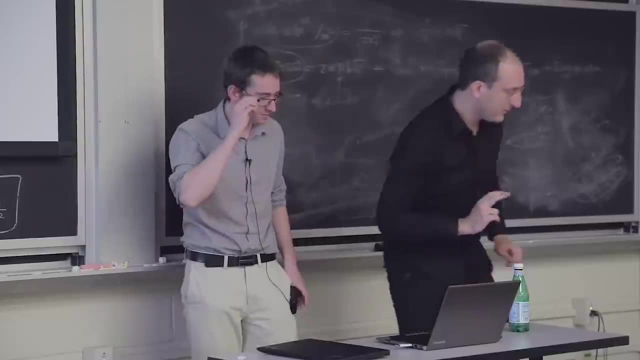 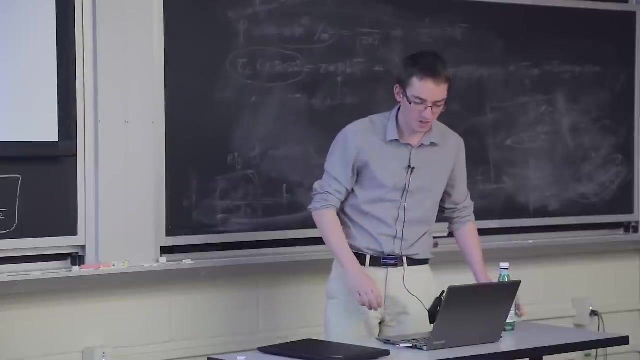 think you will find interesting. I apologize if it's a little disorganized. This was put together relatively recently Because, well, I just got back from Chernobyl and then I went to a conference and then I came back here and tried to get work done. 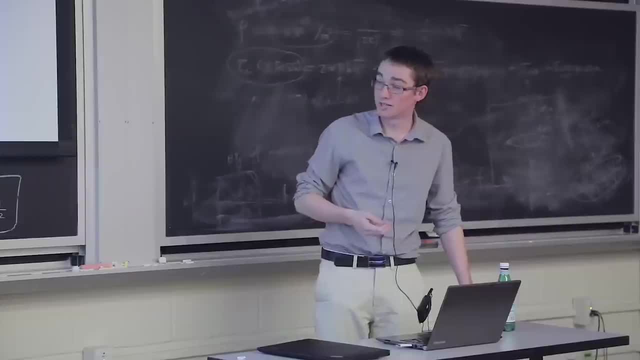 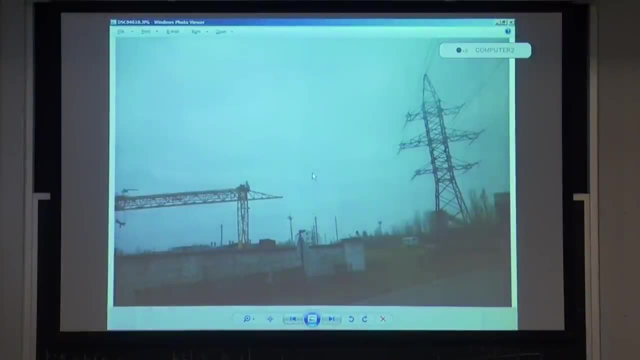 Alright, so these are in chronological order. roughly, I'll go through and hopefully tell you guys a little bit about what the site's like. Yeah, please do the Okay. so this is on day one. We're driving to the Chernobyl nuclear power plant site. 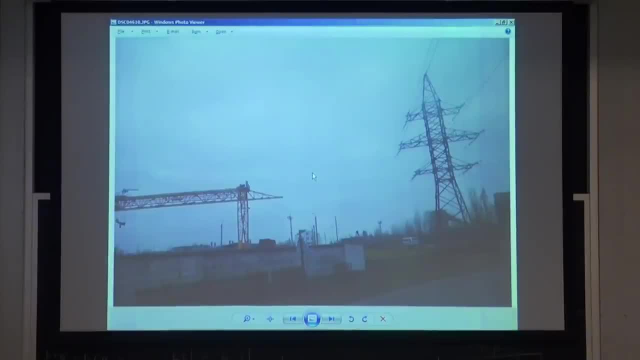 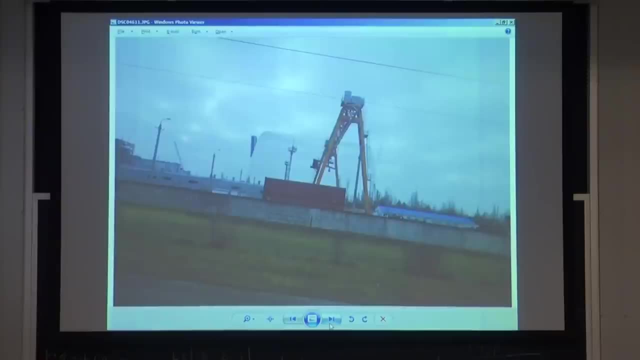 That blue and white bus is pretty much what everyone uses for transport around there. Alright, so we're not really supposed to be taking photos in this area, so everything's tilted because I was taking them out the window with a camera like that. That's the new safe. 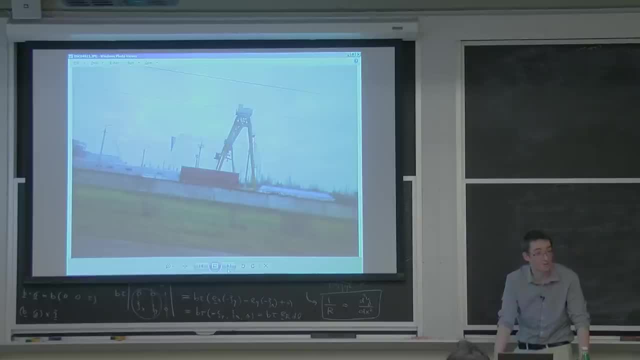 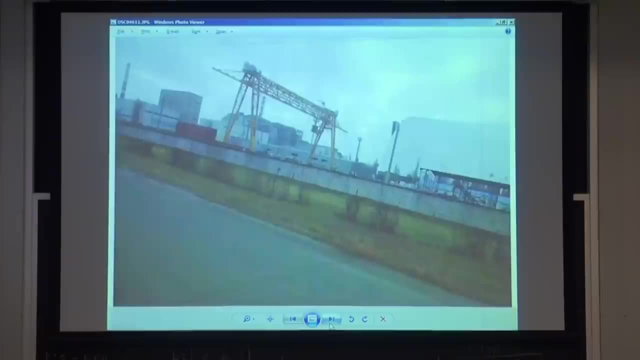 confinement arch. It's in considerably better shape than it was last year at this time. They have done a fantastic job of putting it together. It's actually almost a year ahead of schedule. There it is again. You can see the sarcophagus with the new support wall. 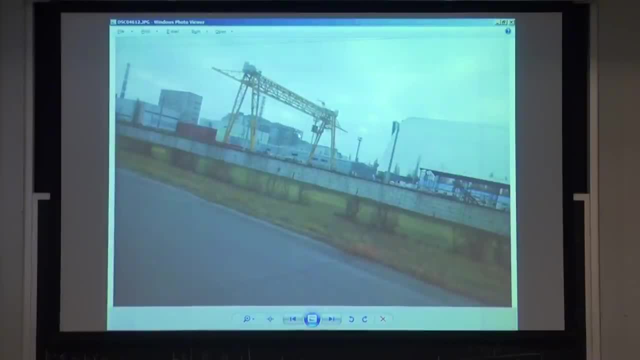 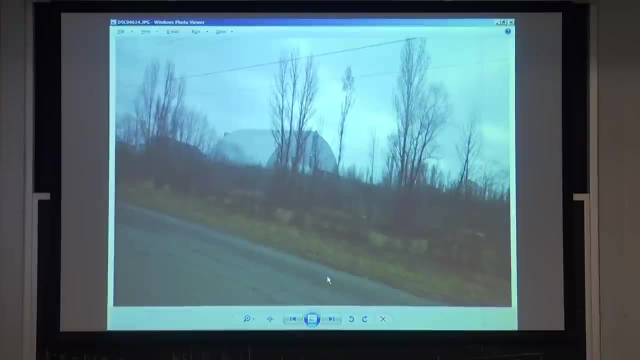 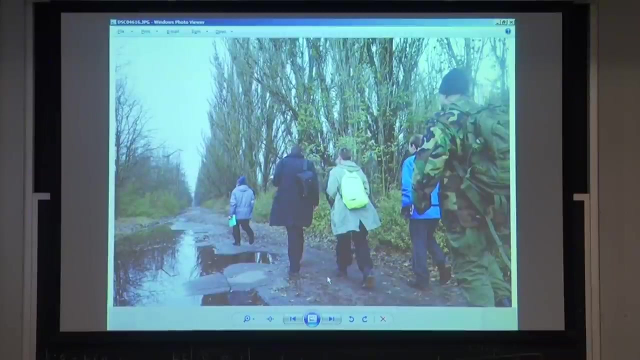 which is that right there. Okay, Alright, so this is our excursion into Pripyat on our second day. So this is the group led by Stanislaus. As you can see, there's not very much left, Just in comparison to what. 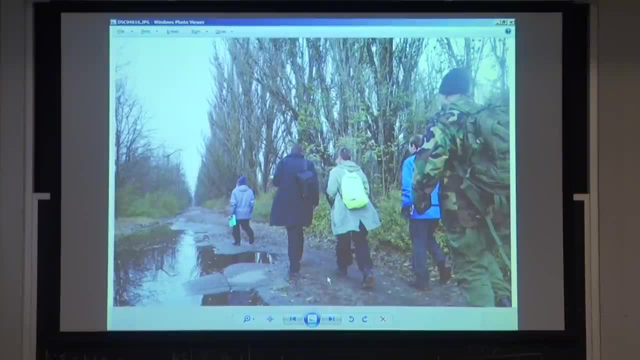 we saw last year, the number of buildings that had been taken apart for scrap metal- illegally of course- was pretty huge. Yeah, In I don't know- five or ten years, it's going to be very difficult to see much of. 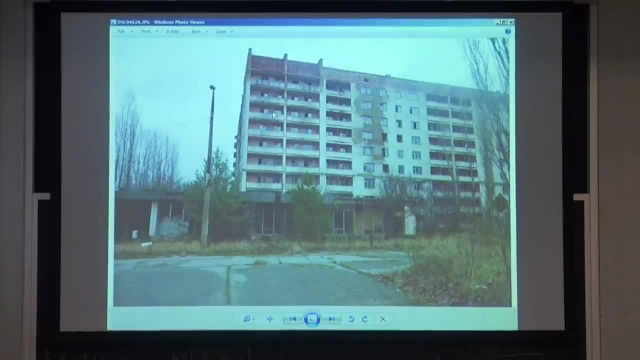 Pripyat at all, frankly. So this is a standard apartment block in Pripyat. As you can see, a lot of broken windows, a lot of bricks have fallen off. These things are pretty dangerous. A lot of tourists do go into them If one decides to do a tourist expedition to Chernobyl. 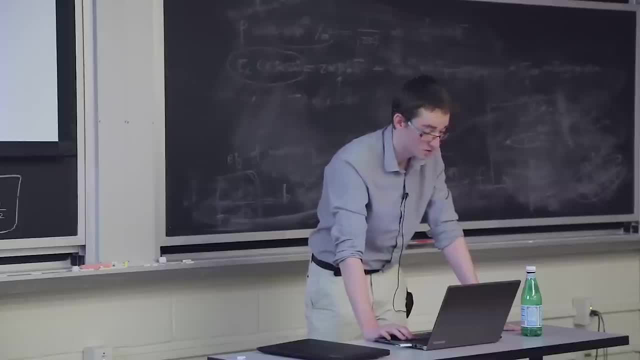 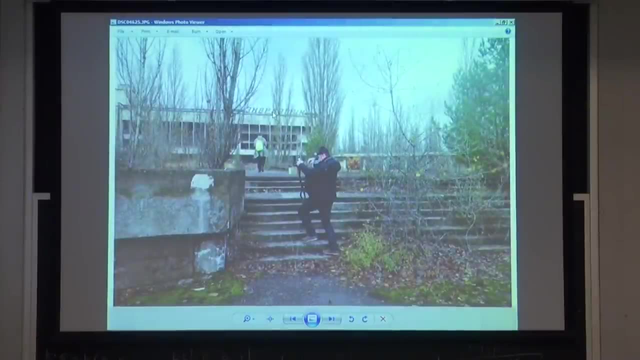 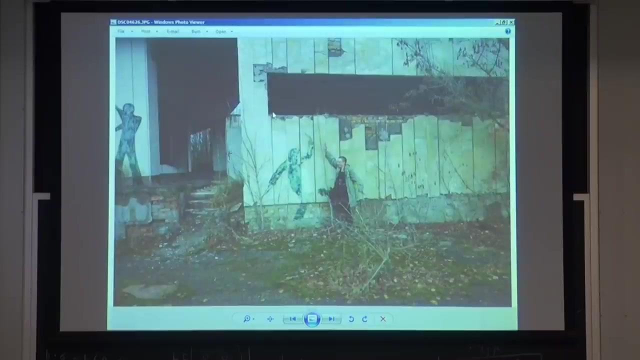 which I don't particularly recommend. don't go in the apartment blocks. This is on the way to one of the schools. Okay, This is Lucas, who has more detectors than anyone I've ever met. He was wearing seven at the time, so I had to take a photo of him. This is Iris imitating some of the 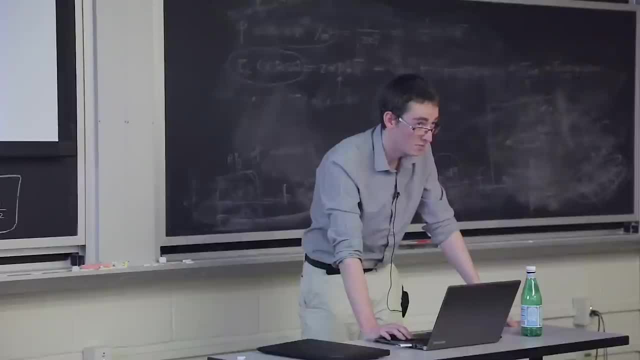 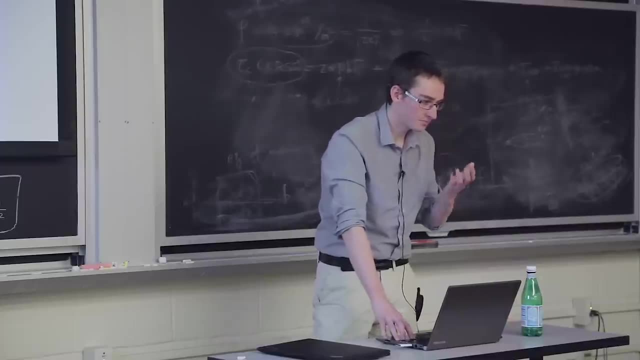 graffiti which, unfortunately, has popped up all over the place. Pripyat itself is really decaying quickly. As I've said, there's a huge problem with looting. In addition, there's a huge problem with graffiti and vandalism. It's really depressing, honestly, to go there. 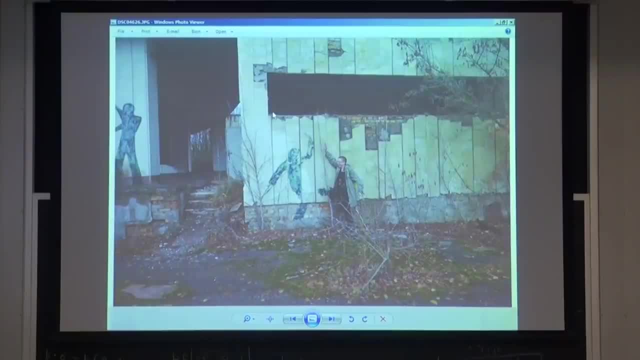 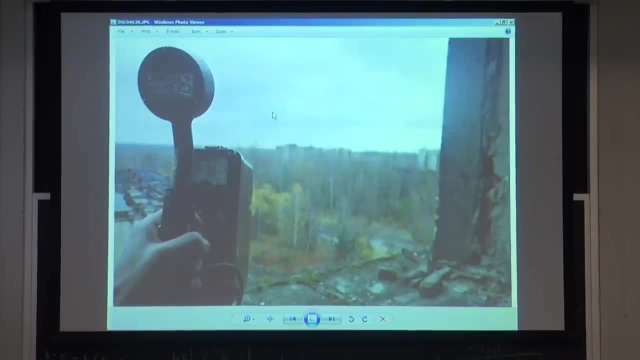 and see how much has changed. How much has changed just in a year. So, despite my earlier warning, we did go in an apartment block. This is just a measurement showing that the background up there actually is not terribly high. That's Iris, not particularly. 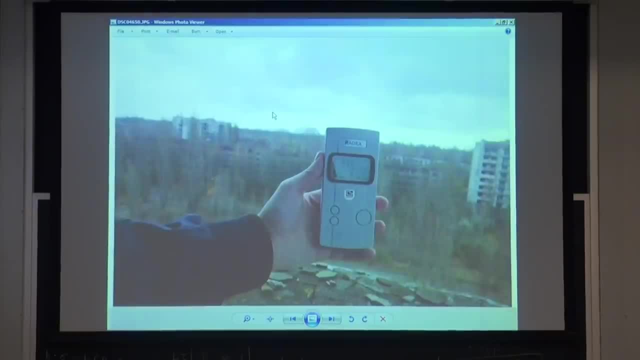 safety conscious at times. This gives you a good idea of how far away Pripyat is from the reactor. Pripyat is not very far, about two kilometers, So you can see the new safe confinement arch to the top left of the detector Background. there is about in this particular apartment. 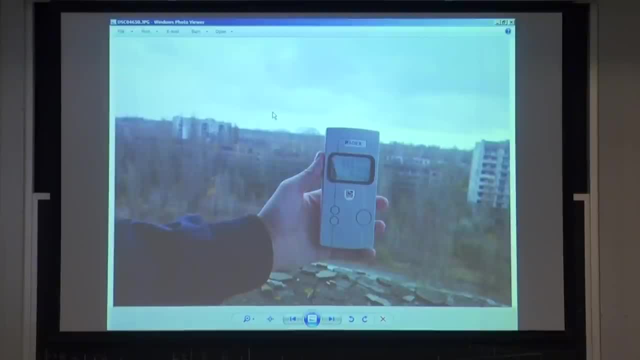 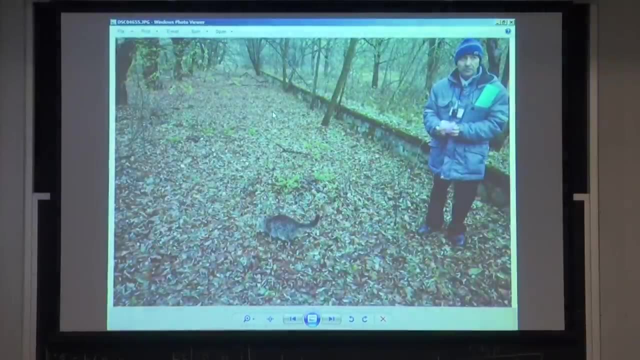 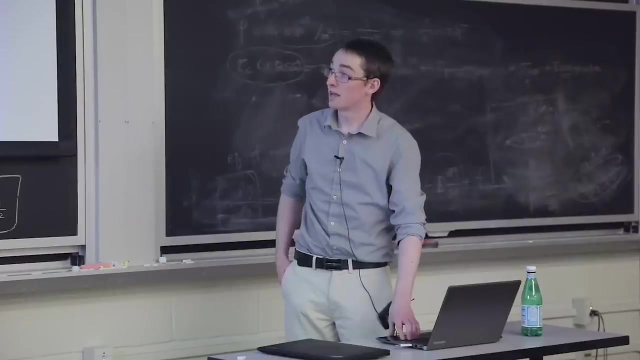 block at this particular time was about four to five times what you would see in downtown Cambridge. There are wild animals in Pripyat and the rest of the exclusion zone. This is a huge problem. So, despite the fact that the cats are very cute and the puppies are very cute, 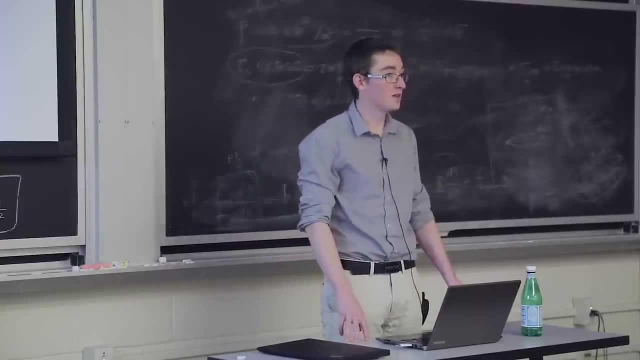 they also have rabies- Not all of them, but a very large number of them. In 2009,, five workers were injured by, I kid you, not a rabid wolf. There's a YouTube video of this that you can look up on your own time if you so wish. This is because Ukraine doesn't have 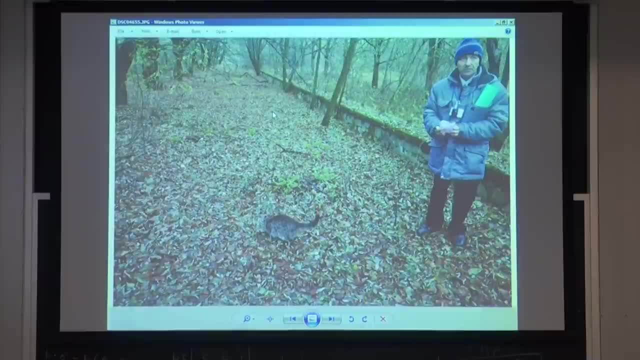 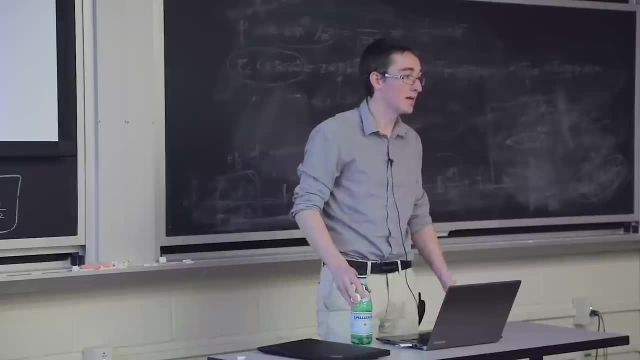 a lot of money so they have not been able to continue with their vaccination program. They actually use baits that have a rabies vaccine in them to normally support their lives. They actually use baits to suppress rabies in wild animal populations, but Ukraine doesn't. have any money. They killed the program about five years ago and, as a result, there's a huge, huge problem with especially rabid foxes, because everyone thinks foxes are cute, especially tourists And foxes. when they get rabies. some of them go through a stage in which they 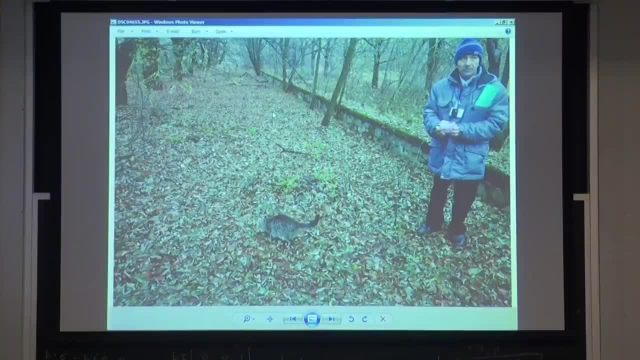 appear to be very friendly. As far as I know, no one has gotten rabies from a rabid animal at Chernobyl, but it's certainly a possibility. So Stanislav was being a very bad example by feeding one of the wild cats. 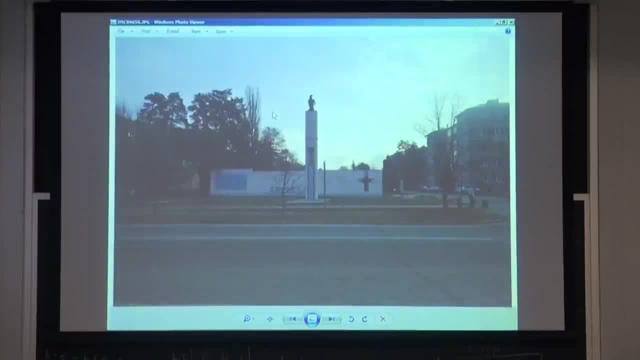 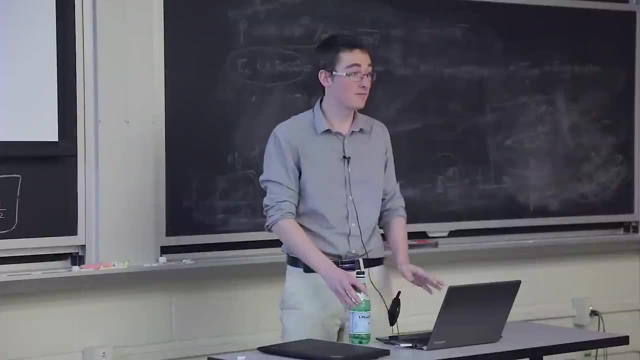 So that's why I took a picture of it. This is one of the many memorials that you'll find in downtown Slavutich. We stayed in this city that was built effectively as a replacement for Pripyat. It's actually a fantastic town. 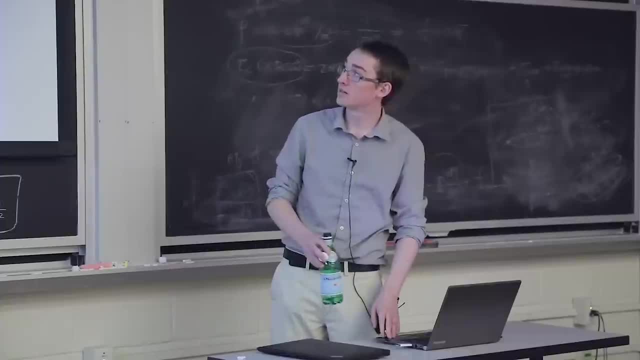 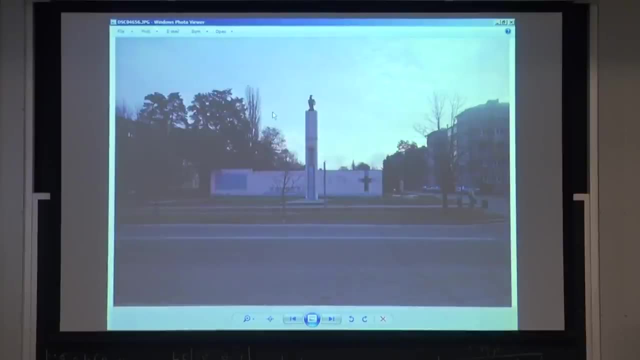 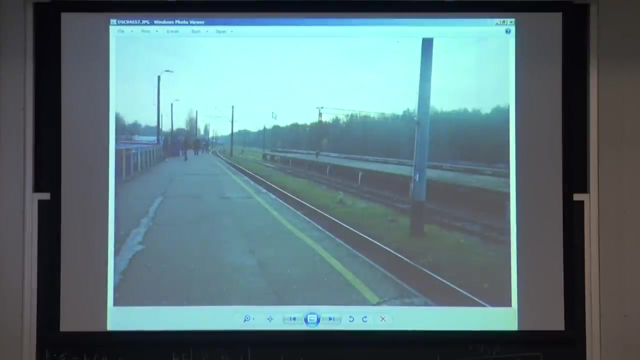 I really enjoy Slavutich And, as one might expect, there are memorials everywhere, because the entire population is basically the folks that were removed from the town of Pripyat. This is a train we would take every day. Slovutich is separated from Pripyat by a little isthmus of Belarus that drops down. 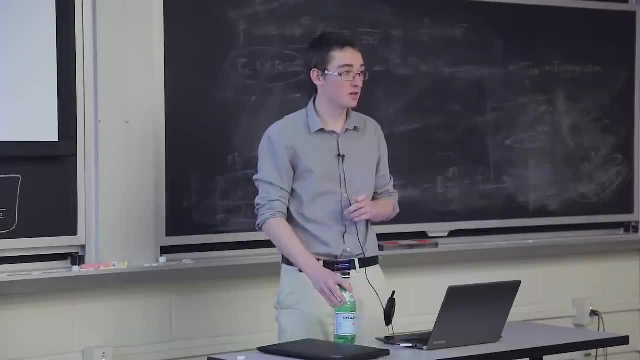 So that's bad because you can't get a visa to Belarus. It's not really a thing you can do as an American. I mean, you can apply for one. you'll just never hear back. Belarus is Europe's last dictatorship And it's not someplace one wants to go for any reason. 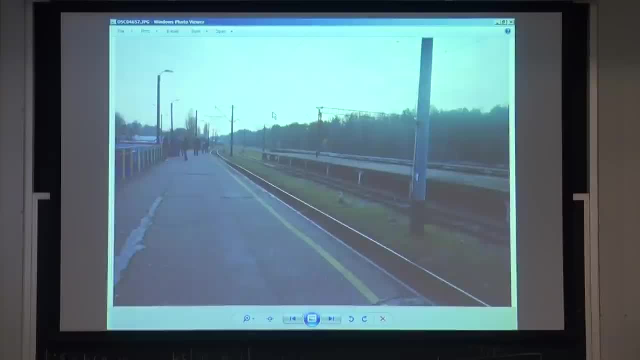 So when we would get on this train, the doors would shut. We would go through Belarus and we would all pray that it didn't break down, Because then we would have to spend some time in a Belarusian prison. But yeah, this is the train yard, bright and early. 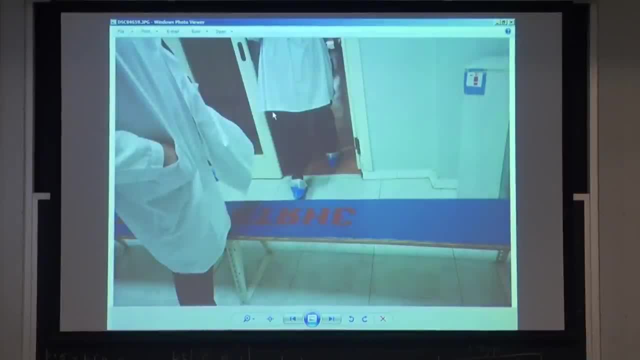 The various zones on the reactor site for cleanliness, so to speak, radiological cleanliness, are separated by these benches effectively that you have to step over So that it reminds you that, hey, this is the clean area. You need to be wearing boot covers and you know. 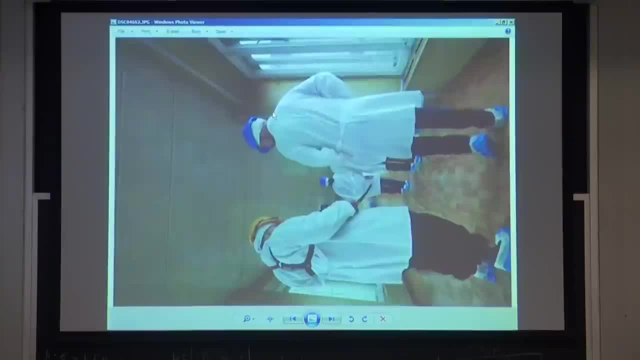 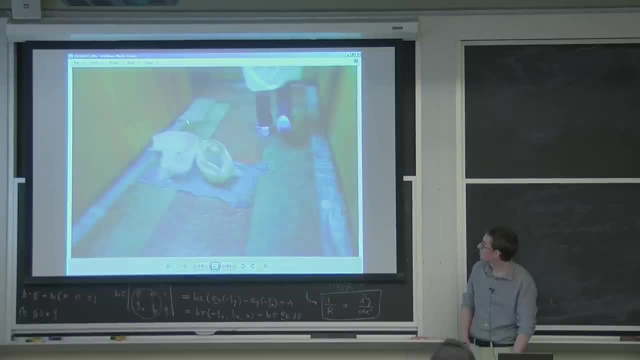 at least these garments, in order to go here Sideways. for some reason This is part of the all right. I don't know why these are all sideways, But regardless, you get the picture. If you notice on the top of the screen, which should be the left of the screen. 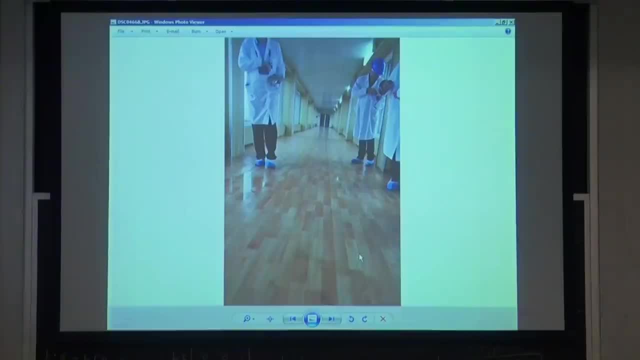 let's see if I can rotate it. That's a giant. That's a giant puddle of water. This place is falling apart Despite the fact that they have money from the European Bank on reconstruction and development for the new safe confinement arch. 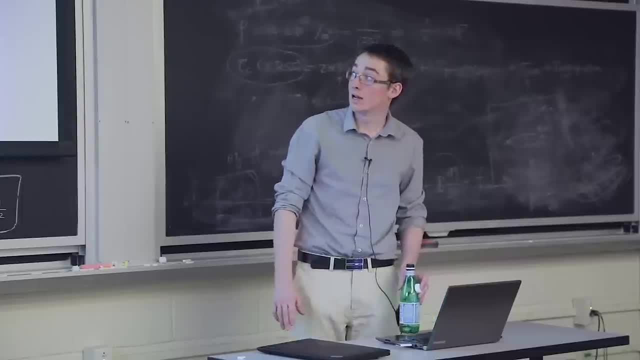 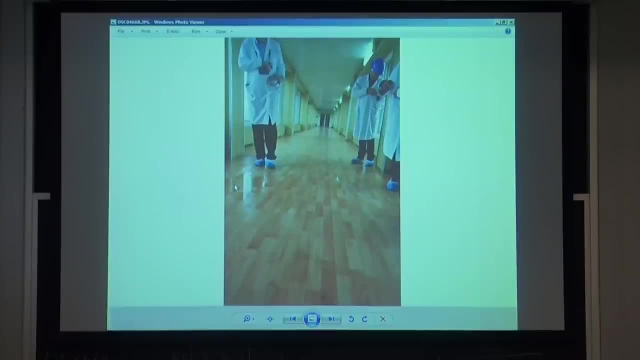 the Chernobyl site itself does not have a lot of money And as a result, things are falling apart and the amount of contamination that is getting into places where it very much shouldn't be- like this quote, clean area- is fairly high. 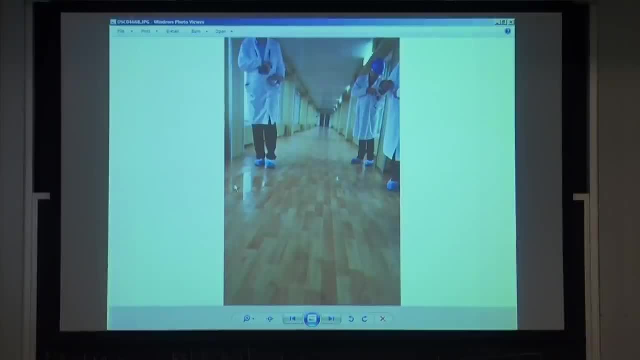 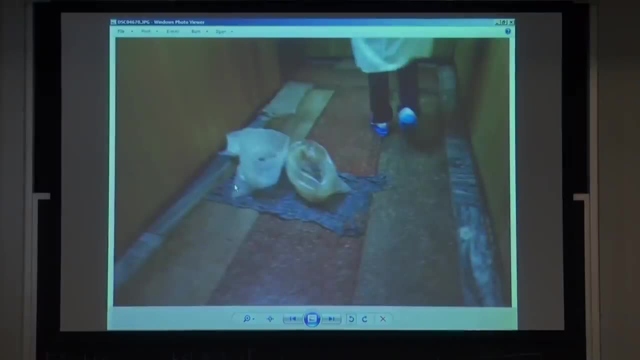 That puddle of water was pretty toasty: something like 5 to 8 MR an hour on contact. That's generally quite bad. As I said, water is coming in everywhere and in this case they were using leg covers to catch the water. 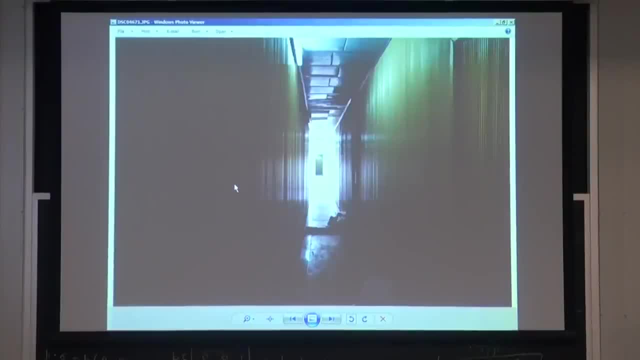 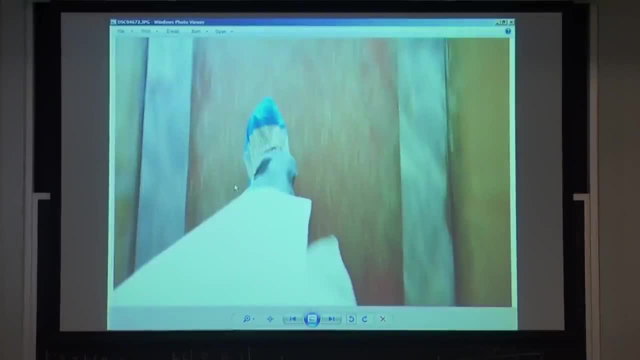 Another one of the hallways that had water leak into it and therefore all the lights are out. The footwear which we were issued, which breaks after walking about a kilometer, which is not particularly encouraging if one wants to take their boots back. 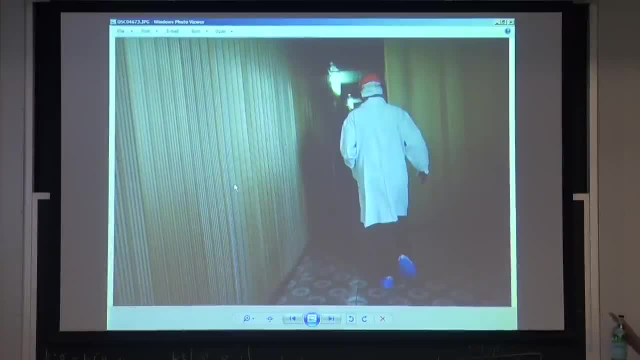 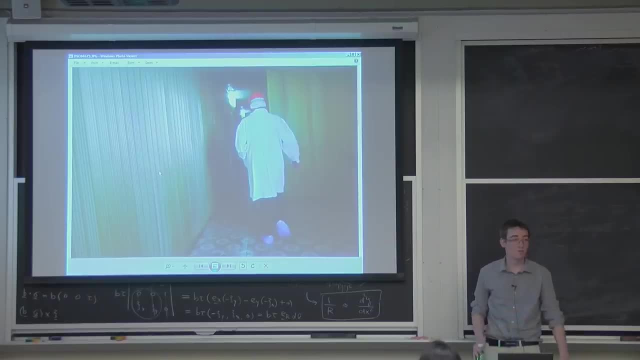 Again walking down the hallway, if you notice this gold corrugated material that you see on the sides, it's aluminum that is anodized and it's placed there because it covers up all of the sheets of lead that were affixed to the wall. 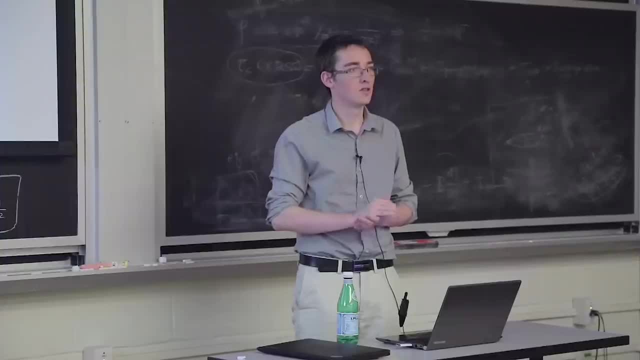 What happened is in the aftermath of the accident. the entire facility was just hopelessly contaminated And you can scrub all you want, but ultimately it's very difficult to get radioactive contamination off of things, So what they ended up doing was getting it down to a somewhat acceptable level. 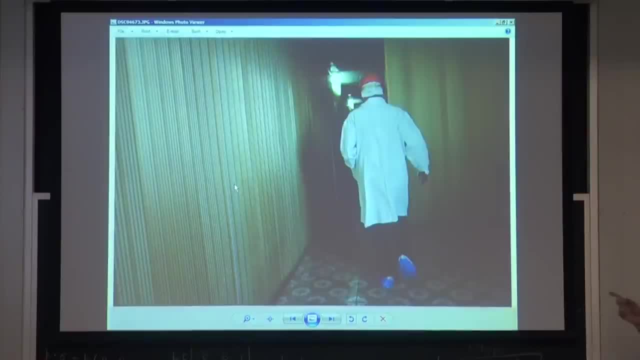 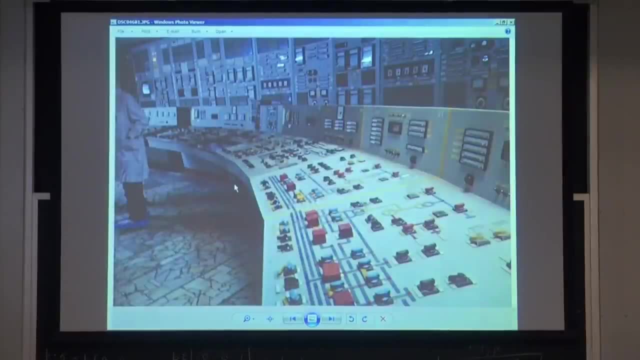 and then fastening sheets of lead over it and then fastening this stuff over the top of that. This is Unit 2's control room. so this is what a fully fleshed out control room looks like. Unit 2 was shut down in 2000.. The reactors actually continued operating after the 1986 Chernobyl accident because Ukraine was in such desperate need of power. As a result, the fuel is still fairly hot, It's producing a reasonable amount of decay heat, and there is a crew that sits in the control room at all times monitoring it. 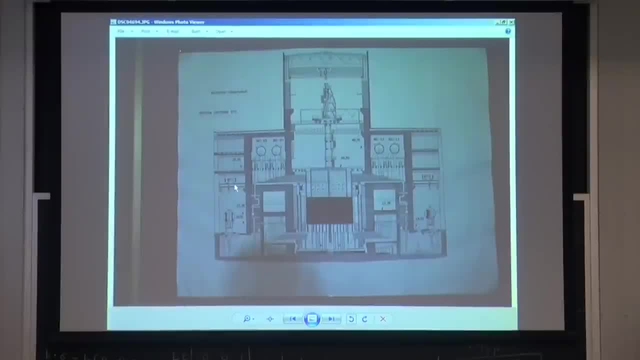 That's Nathan. This is actually. I took a picture of this because it's a very good diagram of the Chernobyl reactor. that's simplified. It shows the core and the relative locations of these steam water tanks. This is the Chernobyl reactor. 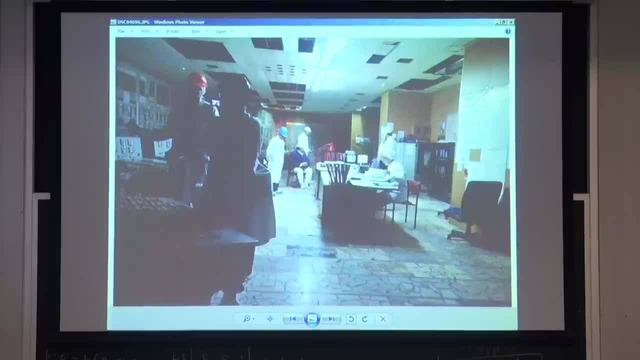 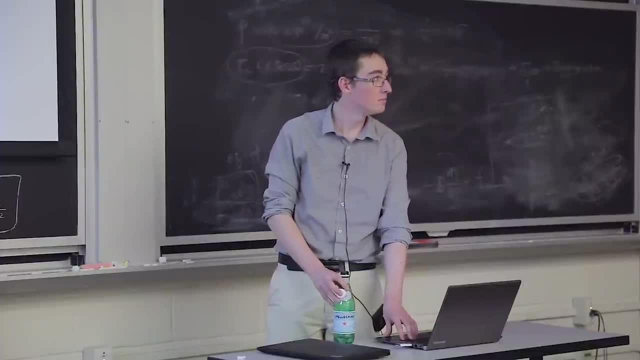 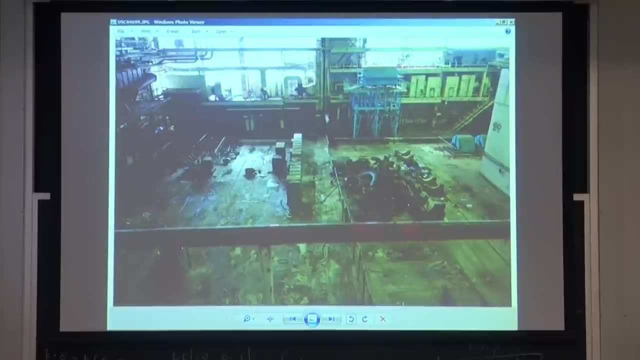 which I have to imagine has to be a bit of a surreal job. This is inside the main, inside the turbo generator hall. Those chunks that you see here are from the turbo generator hall. They're actually a generator of reactor four, So they're quite contaminated and quite easy to detect. 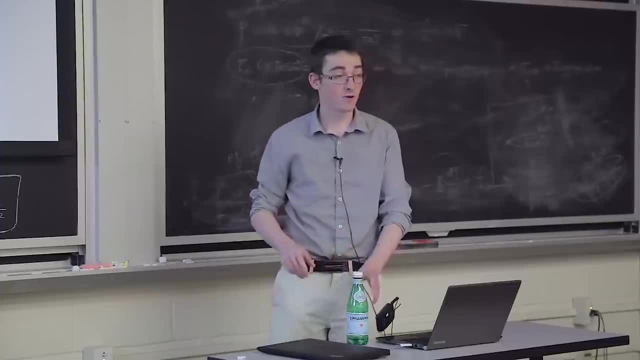 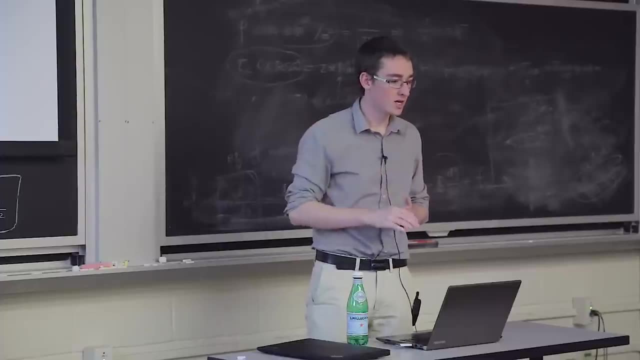 Actually there's a good story behind this. So we were trying to figure out exactly what was making the dose rate so high in the area when we were up there. So we got a group of us to stand in a circle minus one person, so there's a gap. 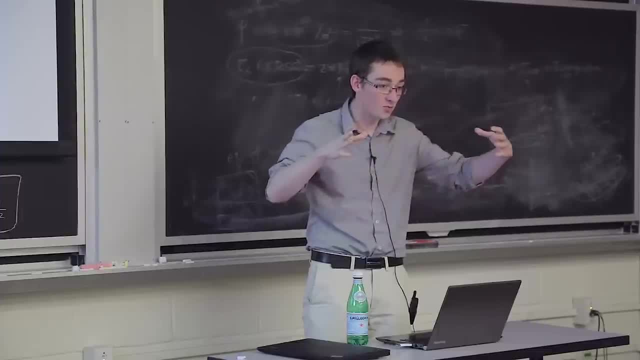 and we got a person in the center with a scintillator and we all kind of rotated around until we found in which direction the scintillator reading was high enough. So we basically made like a two-pie meat shield. It worked fairly well. 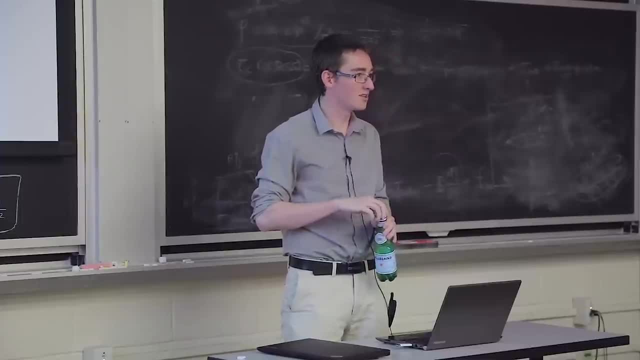 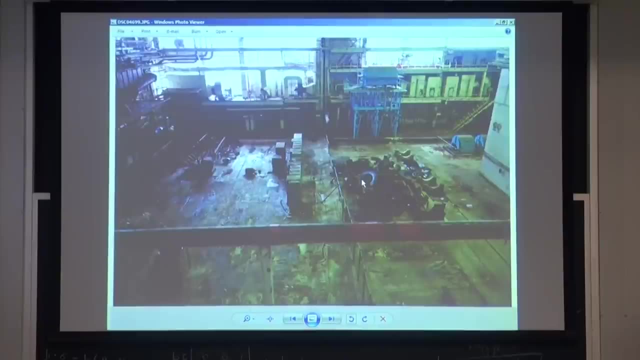 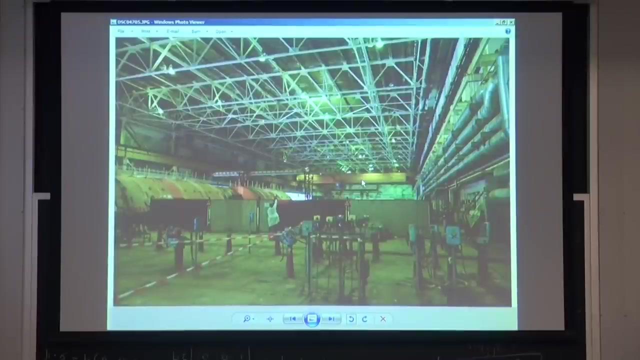 It thoroughly baffled all of the guides that were with us. They were like: what are you doing, linking arms and spinning around? Regardless, that is a good way to find sources if you're in a pinch. This is looking the other direction from that same vantage point as in the last photo. 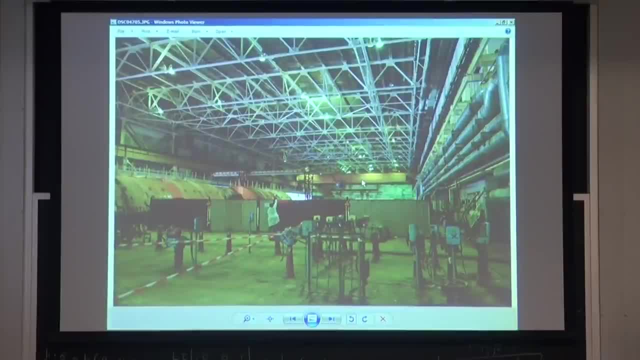 Behind those walls with the little radiation signs on them are chunks of the ventilation stack, Which is fairly iconic. They've been fairly well decontaminated At that fence area. the dose rate, or more accurately the exposure rate, was 10 mR an hour. 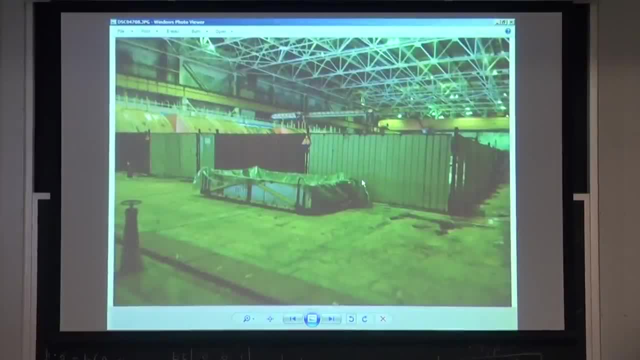 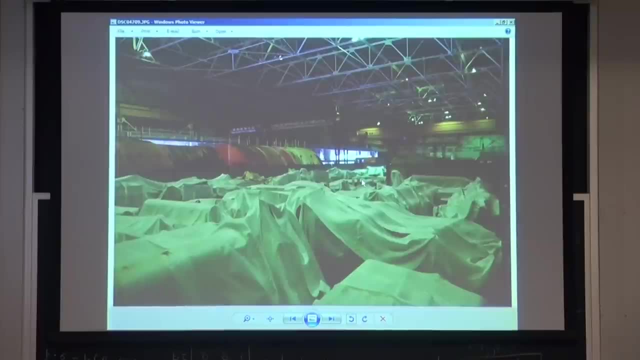 And yeah, that's another close-up photo of it And I managed to sneak my phone over the top of it and get a good shot. Unfortunately, none of the pieces are uncovered. I would really have liked to see the orange and white of the ventilation stack, but I did not. 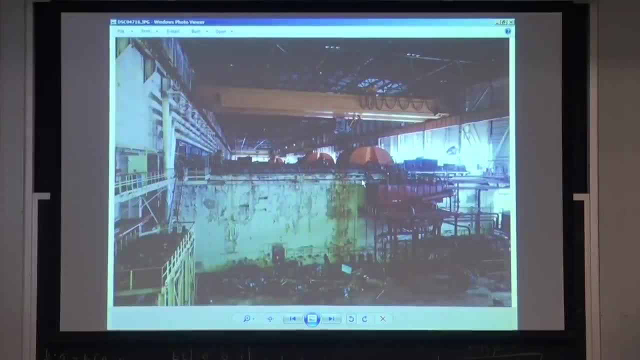 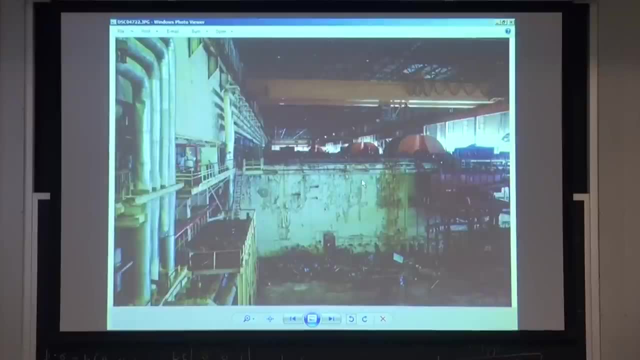 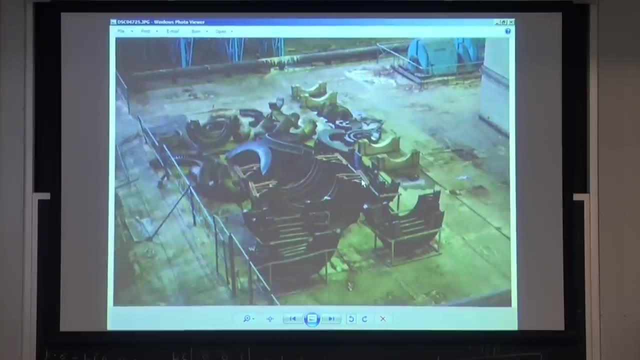 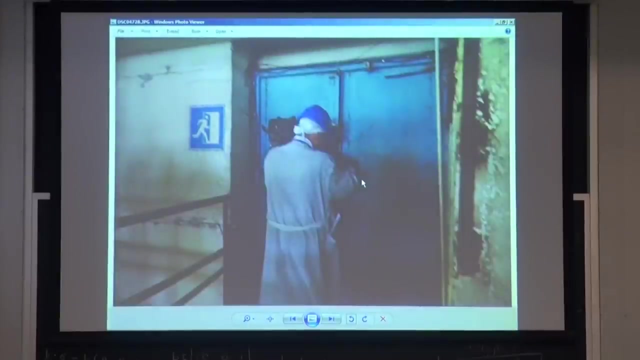 Again same shot, Slightly different shot of the turbo generator hallway looking in the Unit 1-2 direction: More detritus. Oh, here's a slightly better close-up of those components. One of the interesting things I found out about the facility is the way that access is controlled. 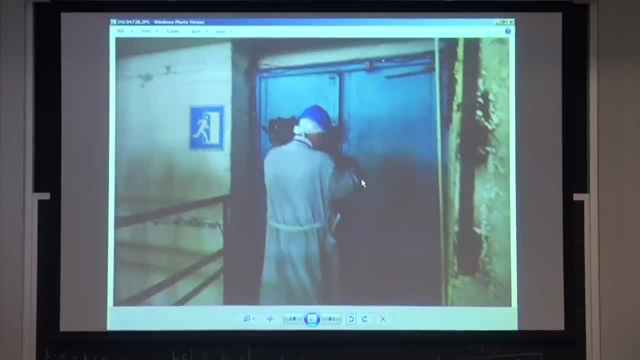 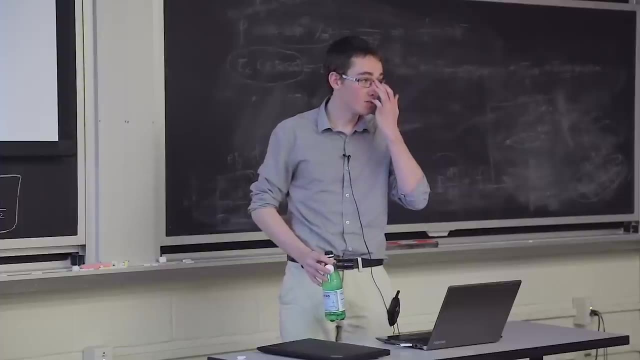 So instead of having, like an RFID card or something like that, they've got cameras and operators. So what you see here is a camera. So Stanislaus would scan a badge That would automatically call someone who is an operator. Stanislaus would say: hey, I'm at this door. 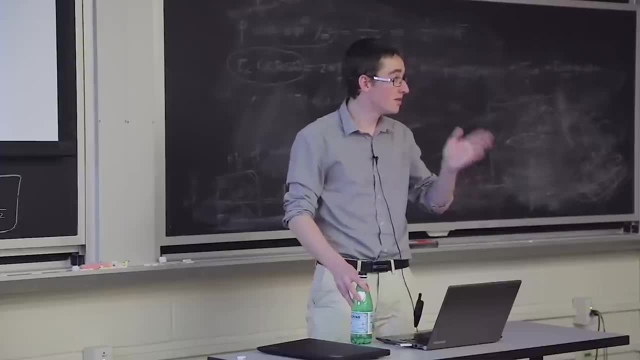 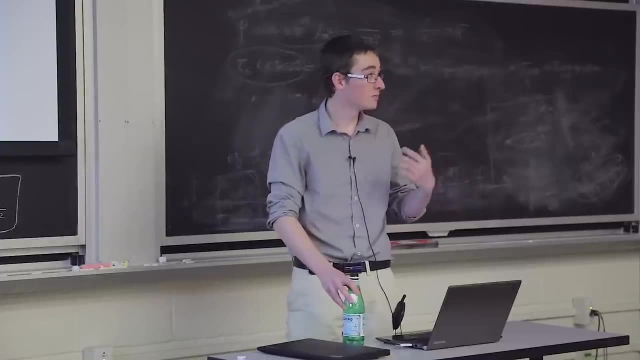 I want to go into this location. Will you let me in? And then they would look at the camera, determine that, yes, that is Stanislaus. He does want to go into this area, And then they would approve it and let him through. 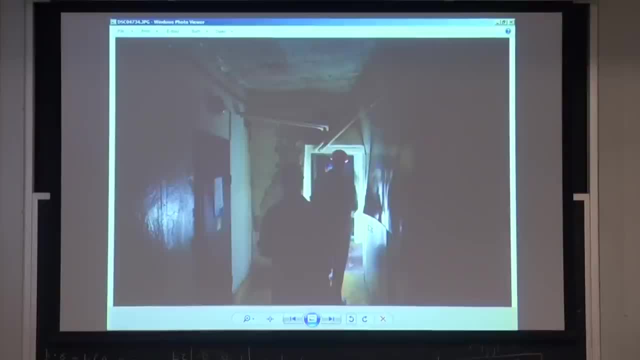 Walking through the corridors of the sarcophagus you can actually see up here those lead sheets I was talking about. I don't know how thick they are on there or how close they are to falling off for that matter, But I'm sure several thousand pounds of lead is right there alone. 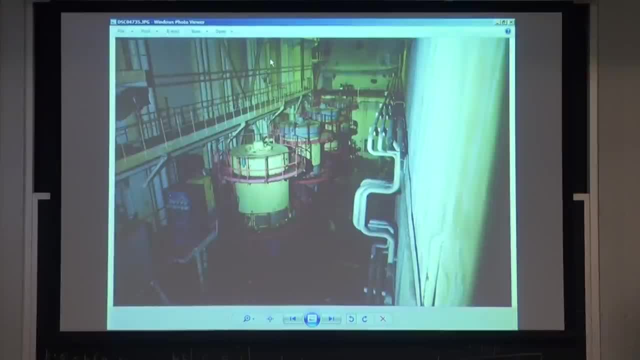 These are main circulating pumps- Well, one-half of the main circulating pumps for Reactor 2.. And each one of these things takes something around something around 40 megawatts to actually operate. These were. these are aligned differently and are of a different type. than the ones used in Reactor 4, because Reactors 1 and 2 were of an earlier design. Ironically enough, Reactors 1 and 2 actually don't have all of the safety measures that Reactor 4 does, which is a bit terrifying to think of. 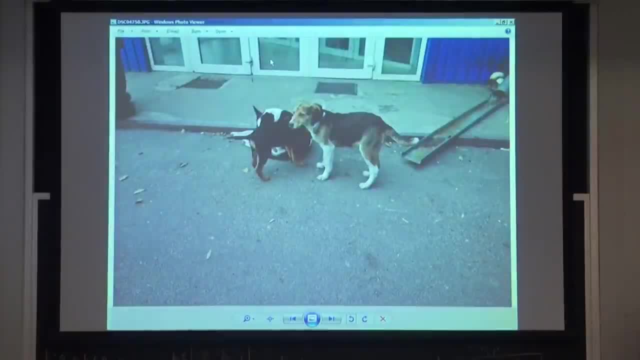 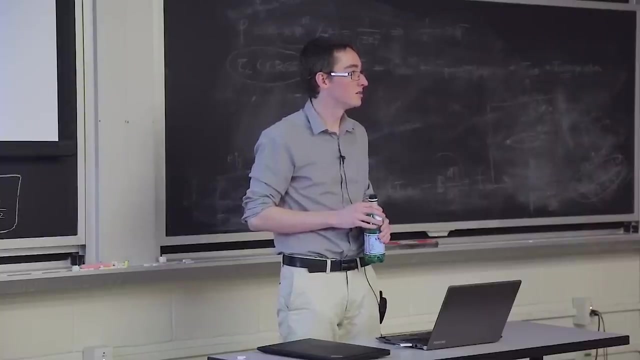 Get more photos Right. As I said, dog problem at Chernobyl. This is right outside the entrance to a clean facility and occasionally these dogs would wander in. Unfortunately, dogs are large furry piles of easily airborne contamination, So they would walk in. you know, people would go to shoo them out. 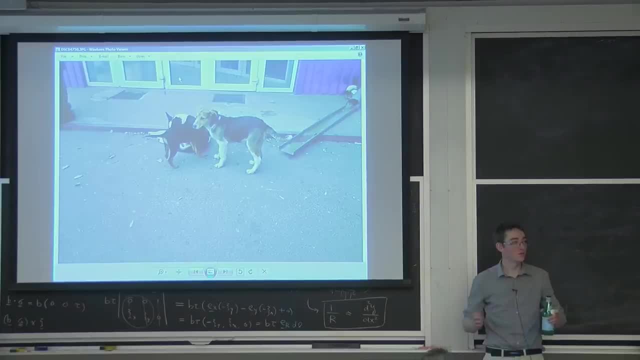 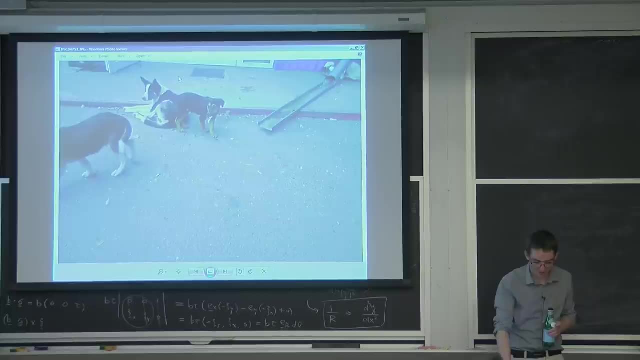 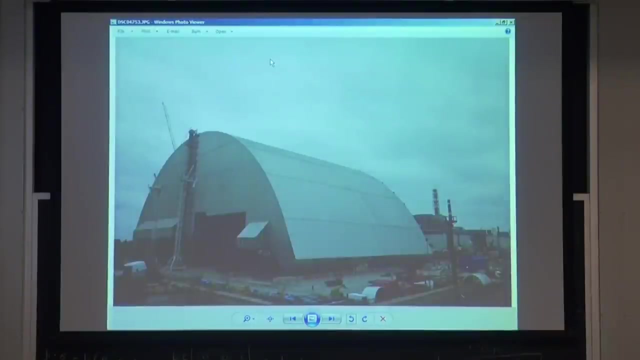 they would shake their coats or whatever. and then you know, clean up on aisle 3, because now there's contamination everywhere. More sad-looking puppies, New safe confinement Yet again. to give you an idea of scale, let's play. Find the Workers. 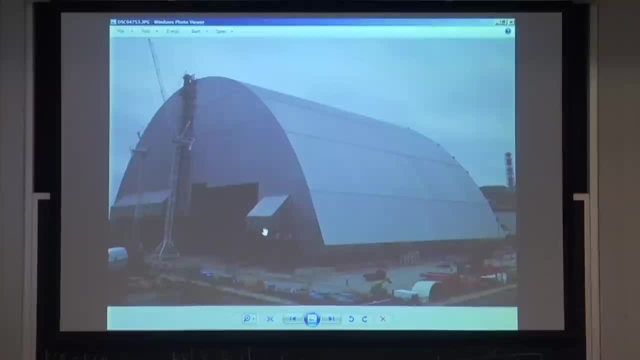 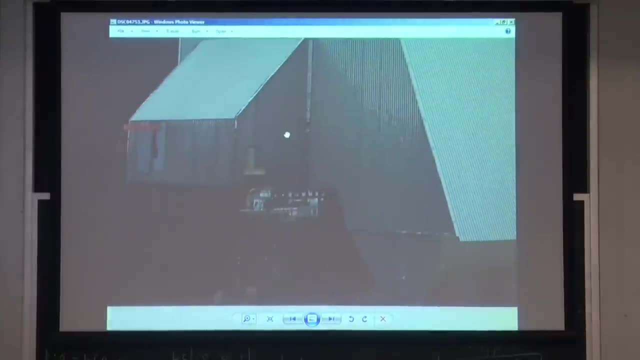 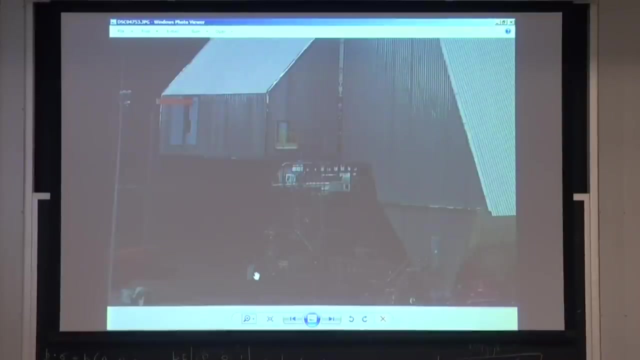 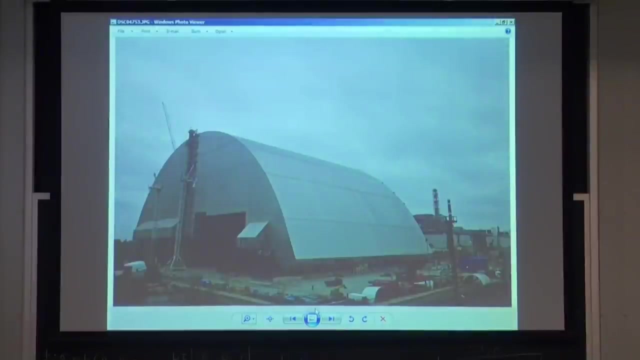 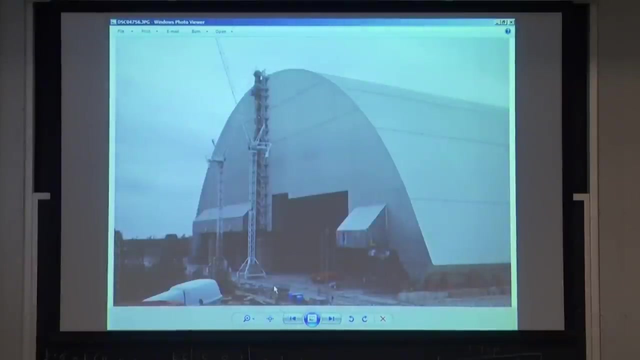 Zoom in. Those are workers Right there. Can you guys see them? Yeah, They're really small next to this facility. Yeah, I think I've got a slightly better shot here. Oops, That's a guy right there. There's also another dude right here. 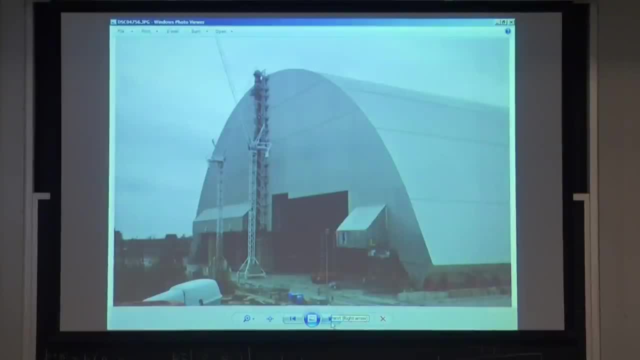 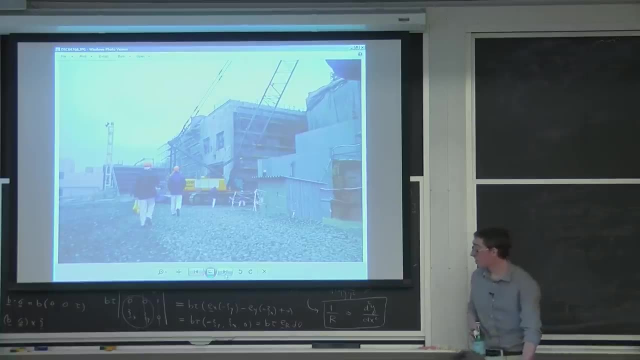 Yeah, This place is, or this structure is, absolutely enormous. It's really hard to wrap your head around exactly how large it is. So this is in an area called the local zone, so it's the immediate several hundred meters surrounding the reactor. 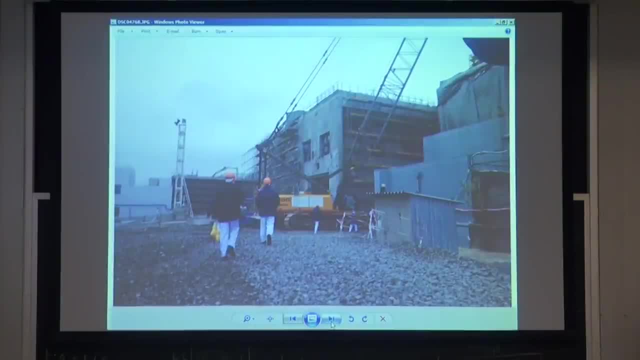 As you can see, the hazmat equipment that we're wearing there is significantly different from what we would wear inside the reactor or inside the sarcophagus, mostly because the threat from dust in this area is pretty huge. As you can see, we're walking on fill. 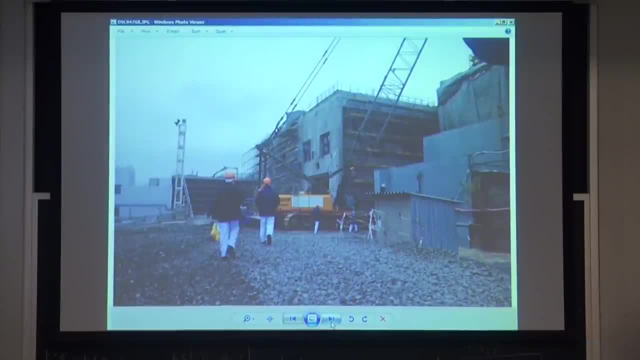 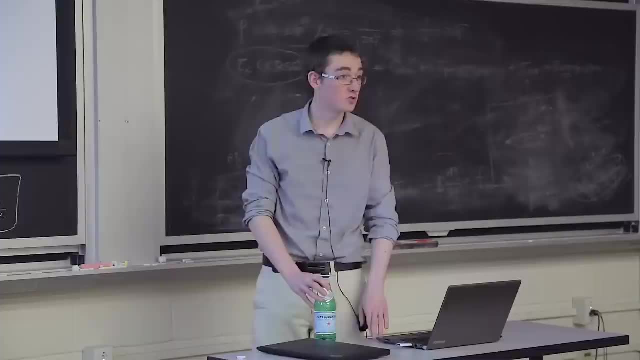 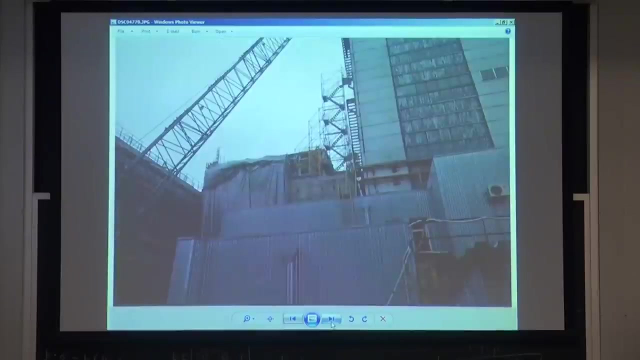 It's actually meters and meters of fill, because the ground was so contaminated that they scraped it away, put fill in there, put fill on top of that, because just the residual contamination was enough to make it hazardous to use as a work site. Though they're not shown in this image or, I believe, any images here, 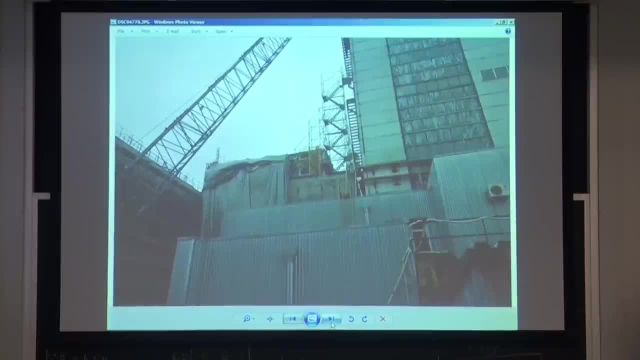 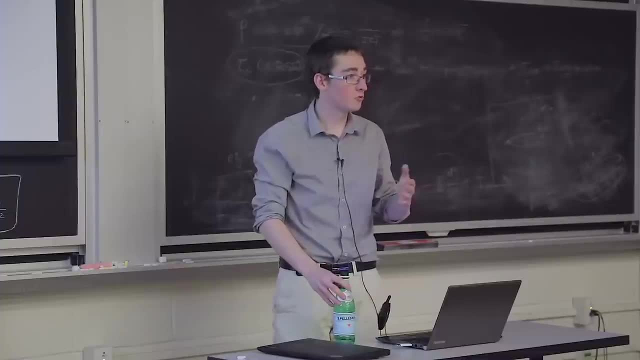 there are little concrete and lead structures that the workers take breaks behind, because you have a dose limit that is enforced while you're working there and if you're going to take a smoke break- as a huge fraction of the population of Ukraine smokes- or you're going to take a break of another sort, 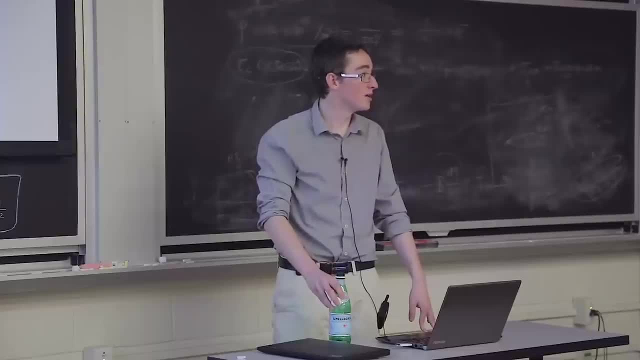 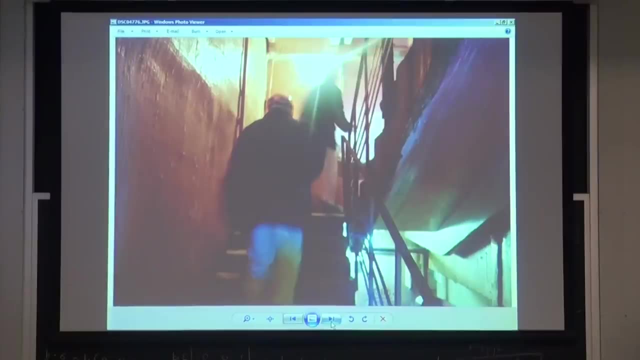 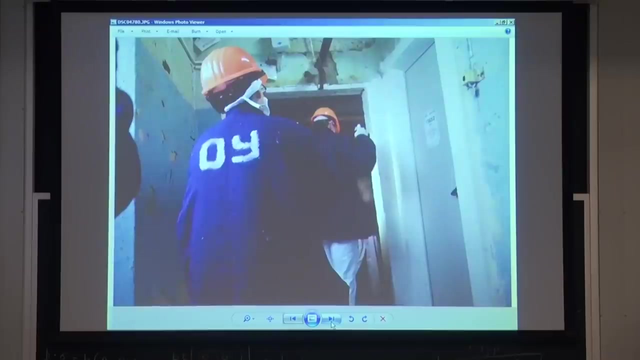 they don't want you racking up dose during that time, so you basically hide in a little concrete shack for a while, with a few inches of lead between you and the reactor. Yet another shot inside the sarcophagus. Ed explaining something about which I'm not sure. 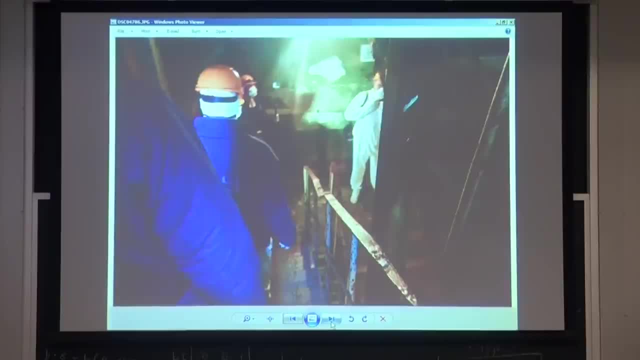 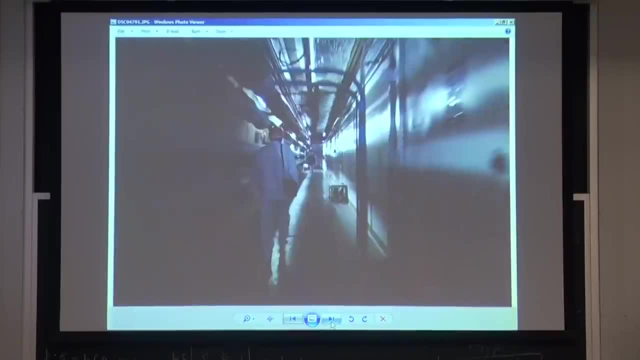 As you can see, this place is not exactly in the best condition on the inside, and one thing that did concern me a lot was the amount of dust that was very, very easy to kick up in the area. This is inside control room of reactor four. 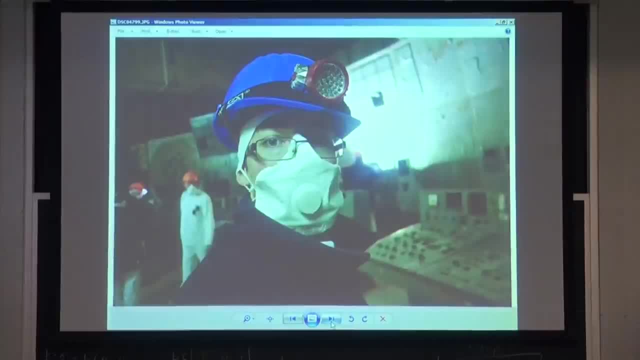 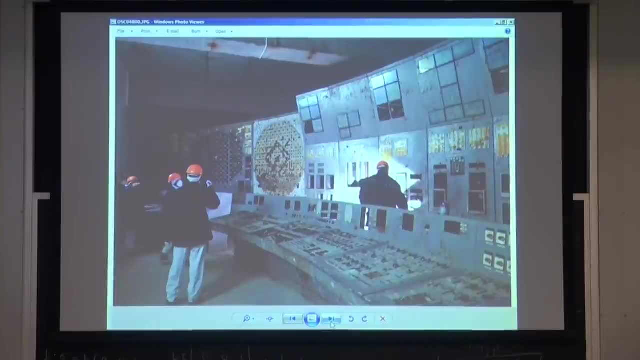 Selfie, which I didn't mean to have in this album. Control room four hasn't changed a whole lot since last year and there is a dividing wall that actually separates reactors three and four. that's being put together and it cuts right through the edge of the fourth control room. 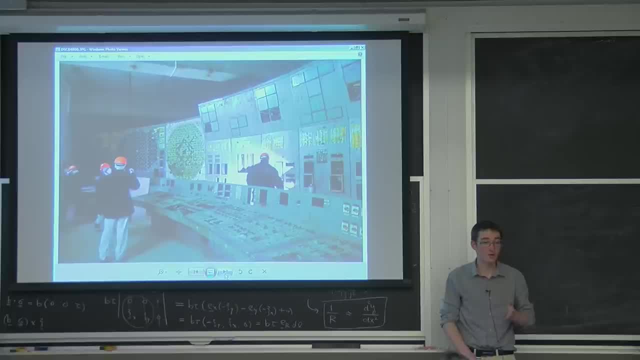 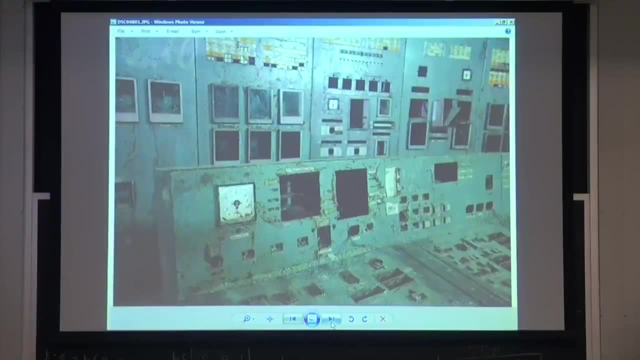 and for a while we actually didn't know whether or not we were going to be able to visit it at all because of ongoing construction. I'm very glad that we were able to. Most of the instruments have been removed. It's unclear as to why. 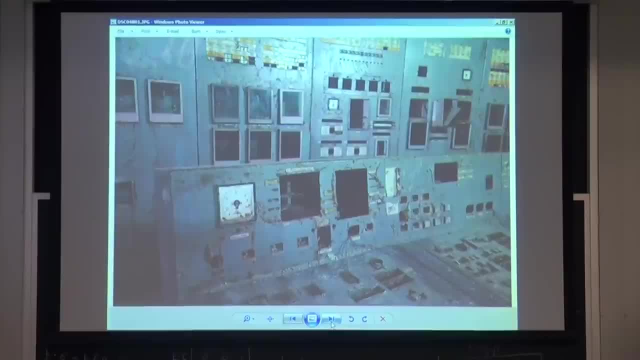 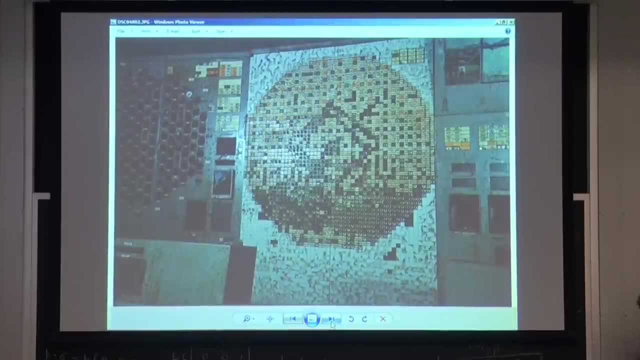 We've been told that some of it was because of contamination, but the pattern doesn't really make sense. This is the reactor control room cartogram- Excuse me- reactor core cartogram which, as I said, was lit and could display various parameters. 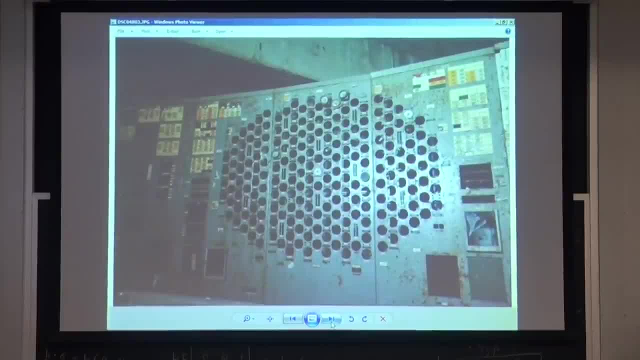 regarding the various fuel channels, There's only two control rod indicator. Well, yeah, there are really only these control rod indicators left, and we believe that actually, some of these might not be original. Someone might have stolen the real one and put another one back. 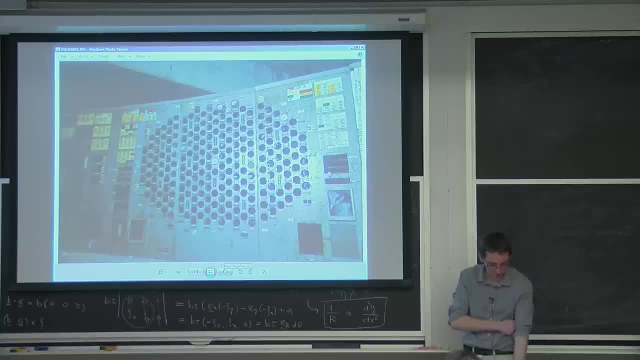 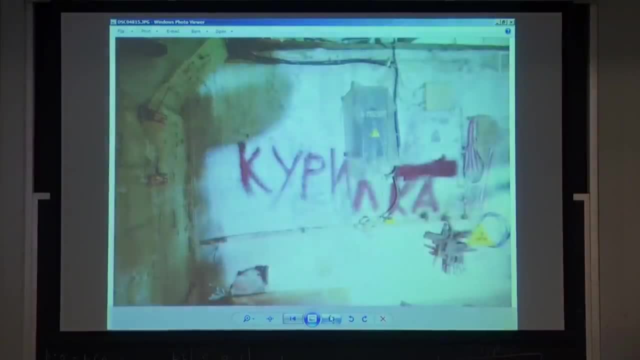 I don't have any evidence to support it, but I suspect that there's significant looting that happens in here. This is a rather entertaining photo. that means smoking area. That's in the control room. You shouldn't be smoking. You shouldn't take your mask off for any reason. 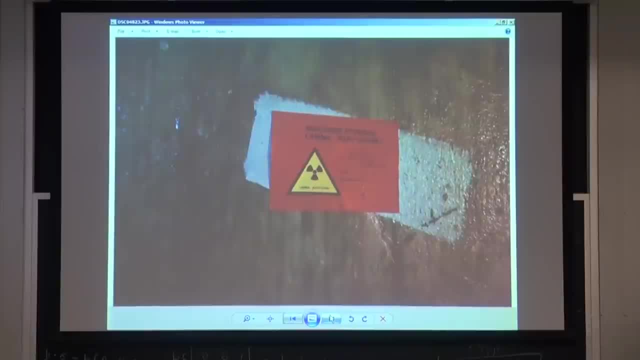 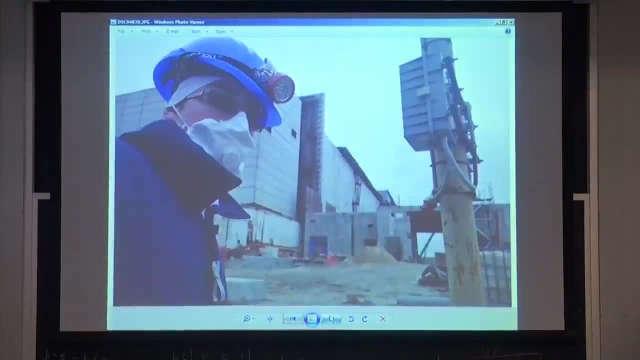 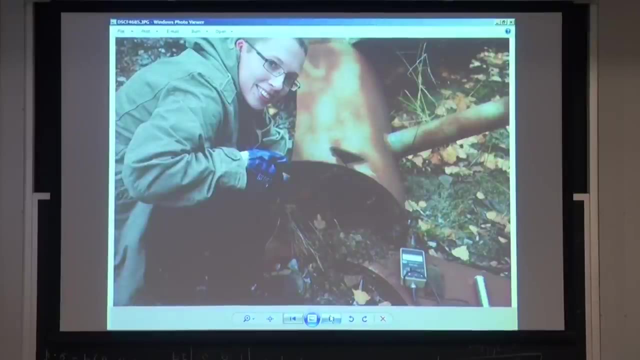 It's a high gamma radiation warning sign. It was in fact not that high of a dose rate, somewhere in the range of 30 mR an hour. We also explored a little bit outside of the more formal part of the reactor premises. 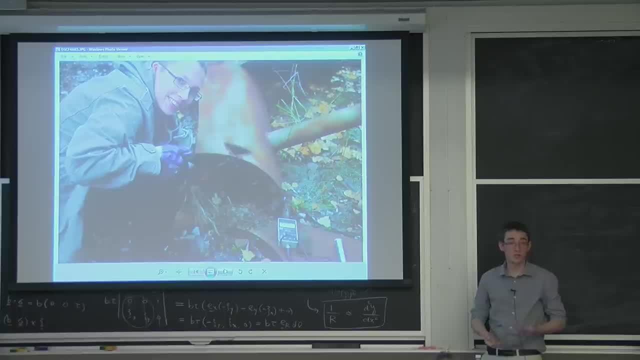 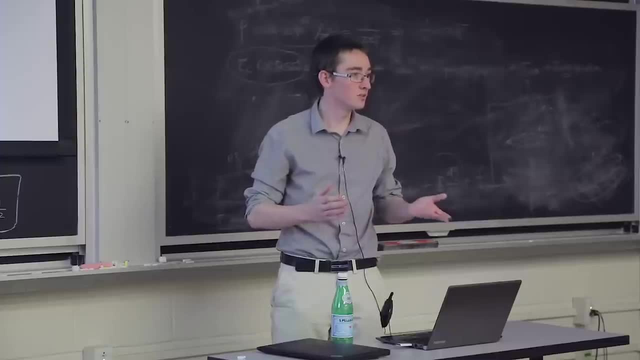 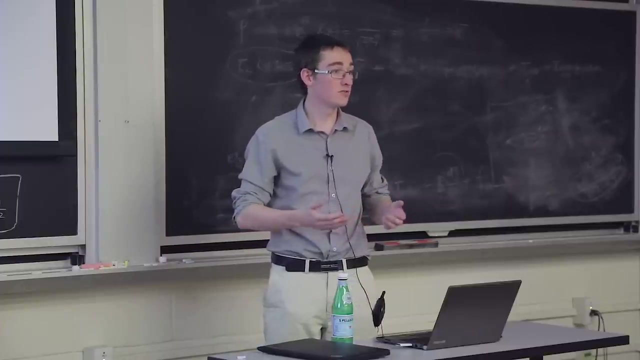 Namely, we went to this place called Buryakovka 2, which is a burial facility for waste from the reactor- Not waste as in nuclear waste, but waste as in chunks of metal and other things that are contaminated and therefore removed- when the new safe confinement arch was being built. 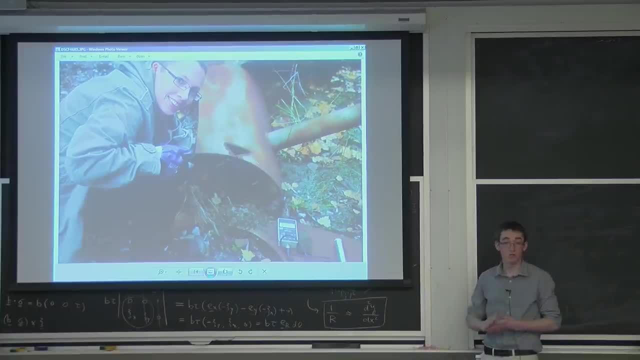 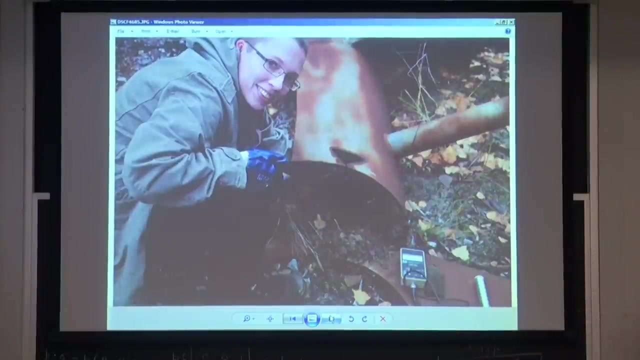 or when, let's say, they were building the separation wall between reactors 3 and 4. And there were some incredibly hot spots, so I might I think I have some more photos later, but just under that little triangle the dose rate was 150 mR an hour. 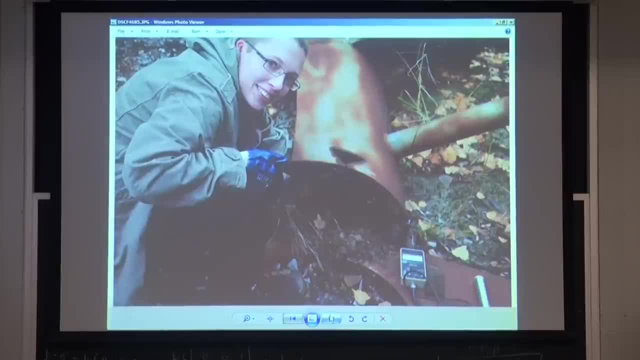 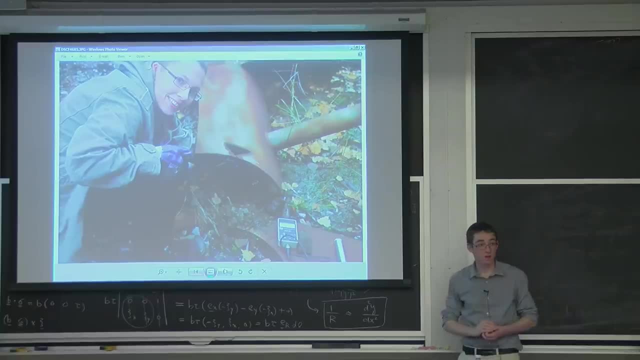 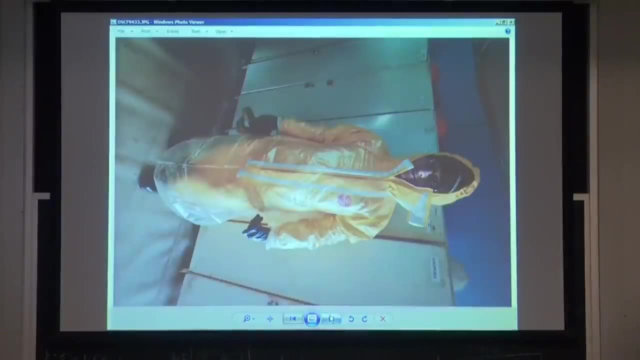 So 0.15 rem an hour. It's extremely high. And that was just in a field basically Not controlled, not patrolled, No warning signs, Getting dressed up, Lots of fun. That was the truck we were sent to decontaminate. 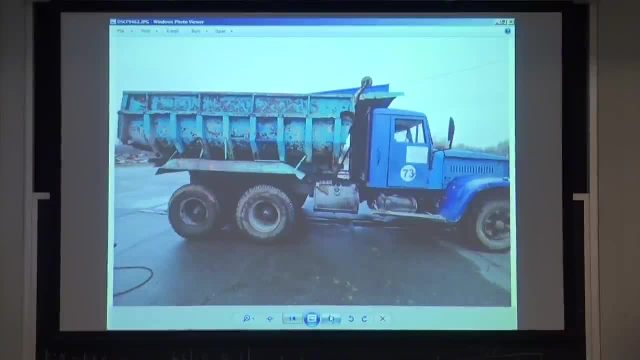 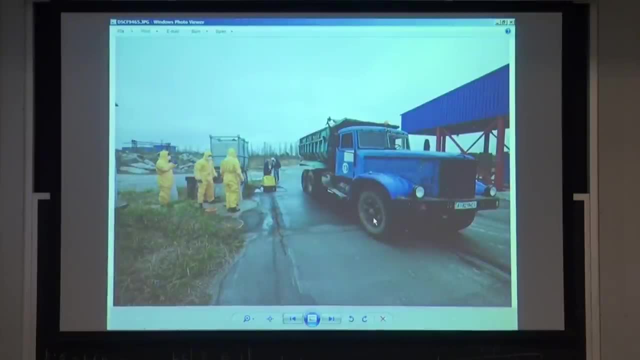 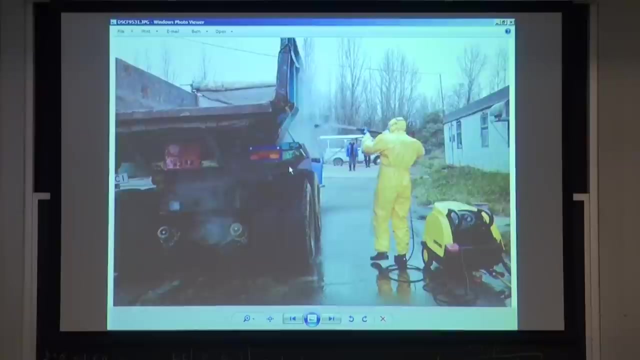 Honestly, it wasn't particularly contaminated in the first place. They weren't going to give us real fun things to play with. It's all of us. And then, as you notice, the real workers here are not wearing even a fraction of what we are. 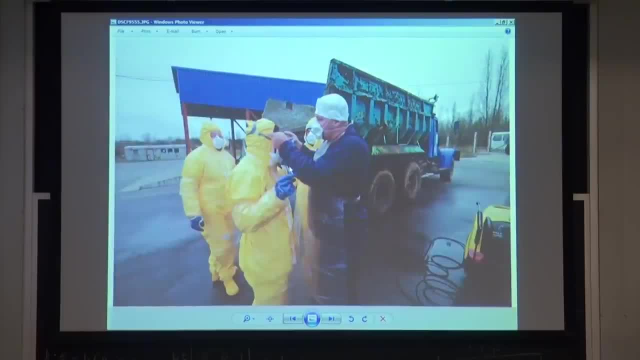 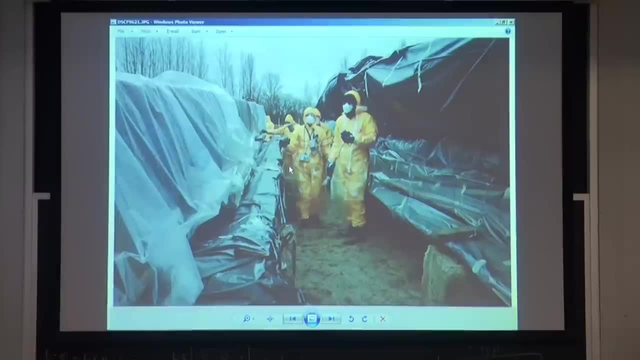 More decontamination? Yeah, see Barely anything. These are chunks of metal that have come out of the reactor. We're not exactly sure what parts they are. No one was really able to answer them. We didn't answer our questions about them. 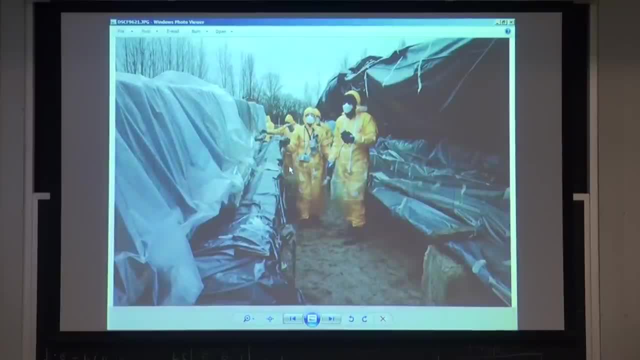 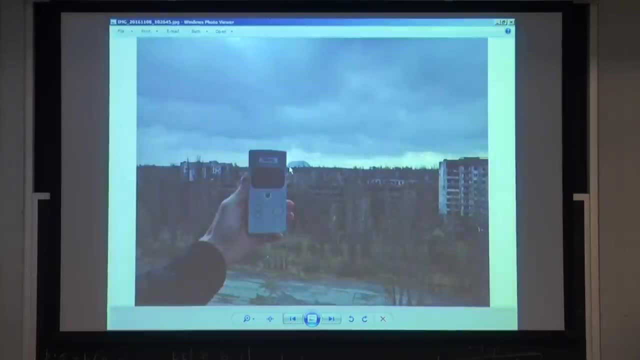 But they were also rather contaminated somewhere in the range of 50 to 75 mR an hour on contact in some spots. More photos of Chernobyl or of Chernobyl from Pripyat Dr J. I want to take a quick break. 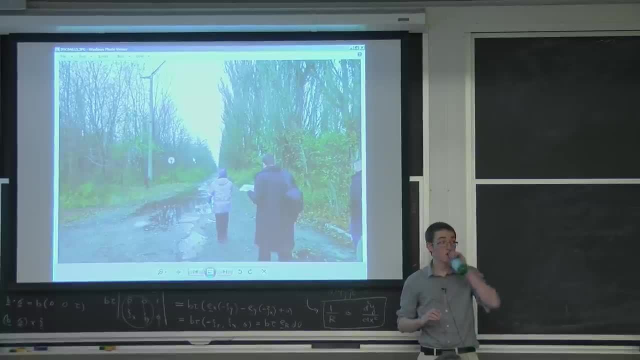 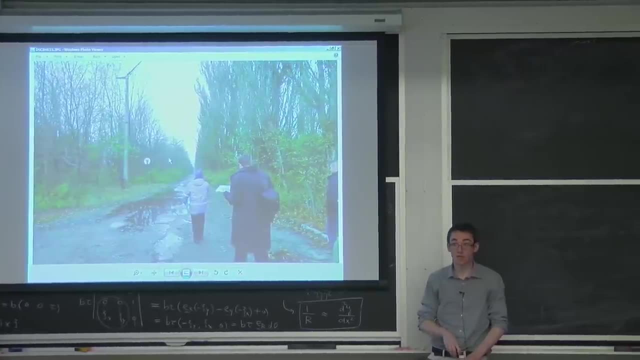 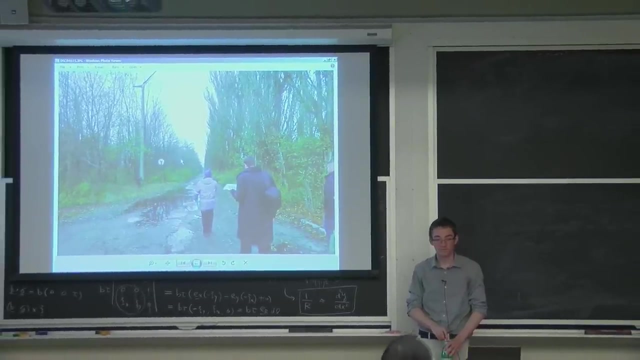 and ask the folks if they have any questions on what the experience is like when they talk: Yes, Did you suffer any adverse health effects or anything? Only the cold. I picked up on the way back The total dose that I received on this entire expedition. 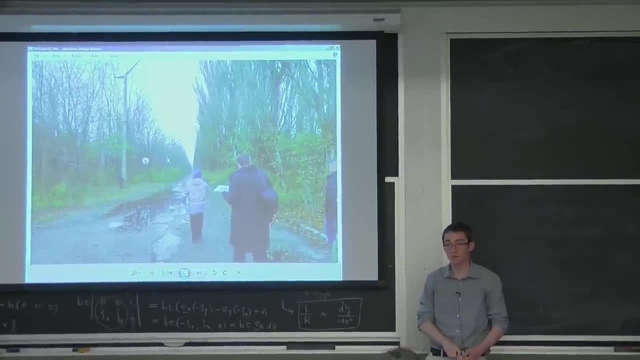 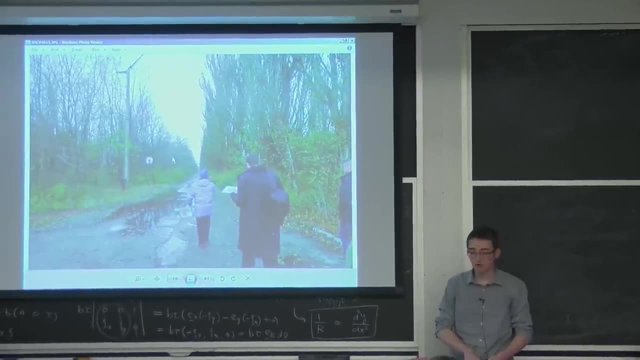 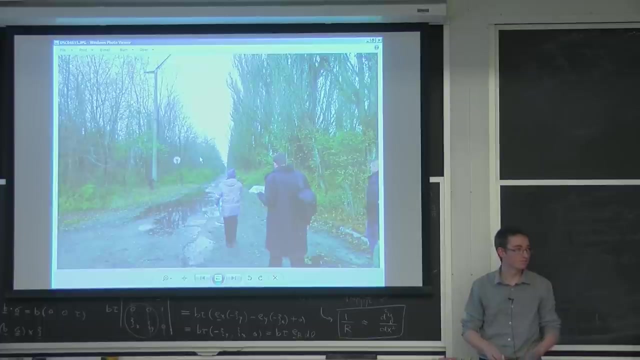 minus the flights there and back was 0.6 millisievert, So effectively nothing. Well, all of the high radiation areas that we were in, we were encouraged to walk quickly. That's basically what it comes down to. 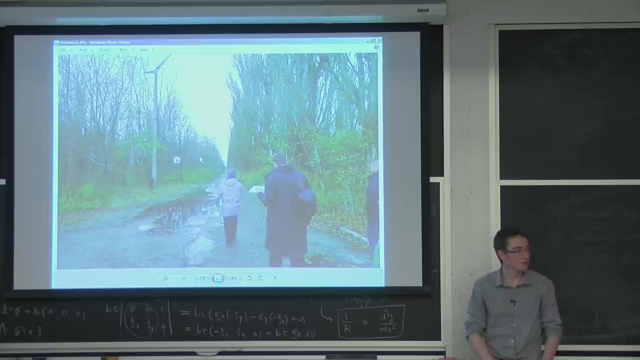 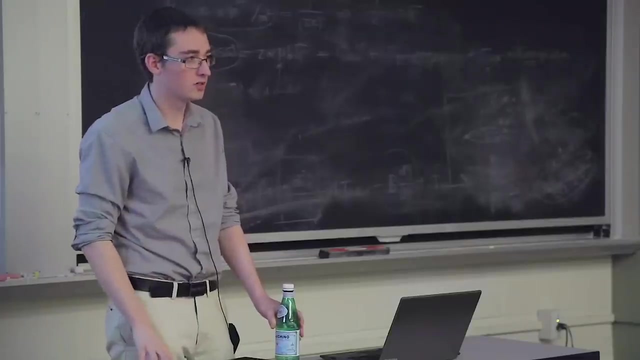 The time portion of time, distance and shielding was emphasized. Further questions: Yeah, Are there cutoffs for like radiation area versus high radiation area? Do they use the same levels? No, Radiological control in Ukraine is a totally different game than it is in the US. 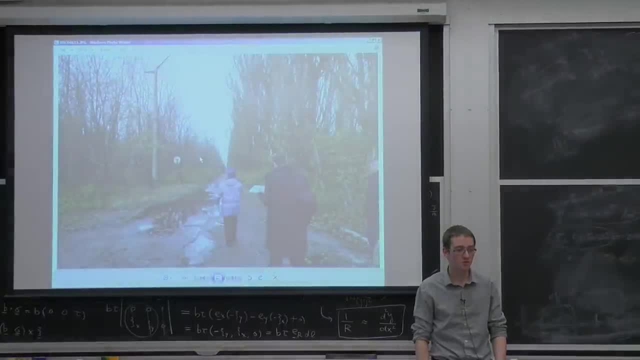 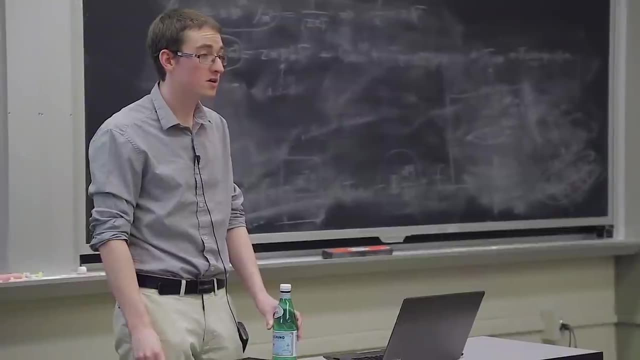 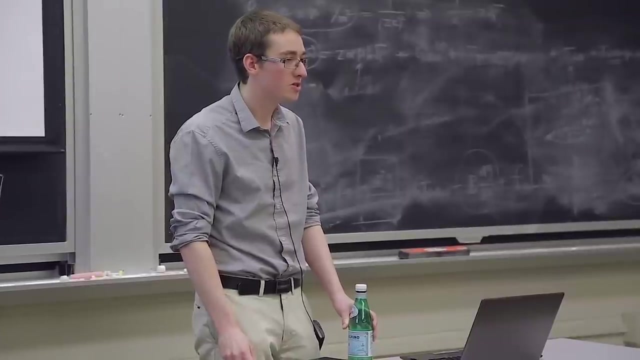 There are the same types of controls that exist in the US, just don't exist At that site. There are for areas that are immediately dangerous to your health. you know, 10 rad an hour, something like that from what I understand. 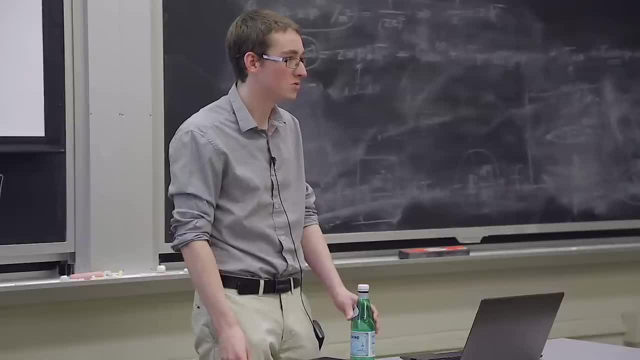 that there are locked doors that prevent one from accessing those accidentally, and there are warning signs in a variety of locations, but I don't think that there is a the same standardization of. you know, 5 mR an hour is a radiation area. 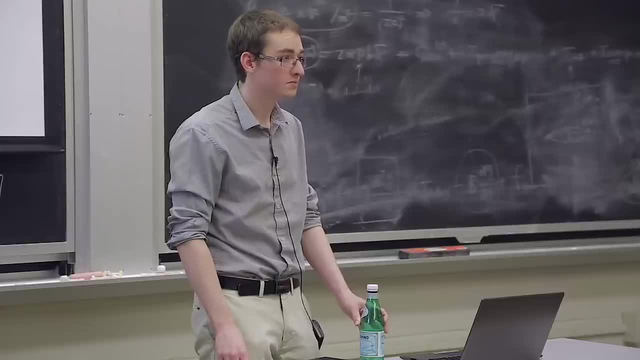 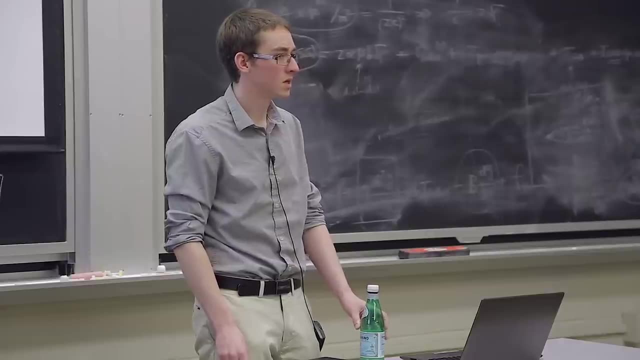 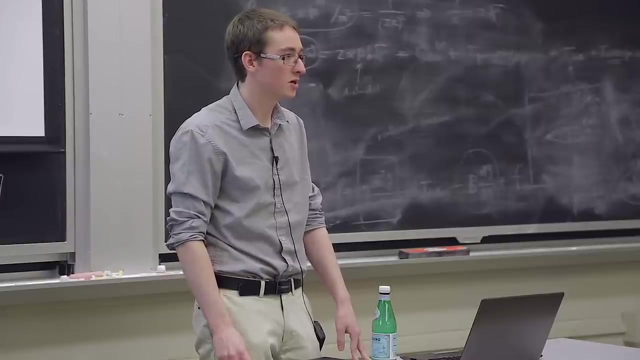 et cetera, et cetera, Yeah, Further, Are folks still going to be running these tours pretty continuously? No, You won't be able to see the sarcophagus itself, because it will be contained within the new safe confinement arch. 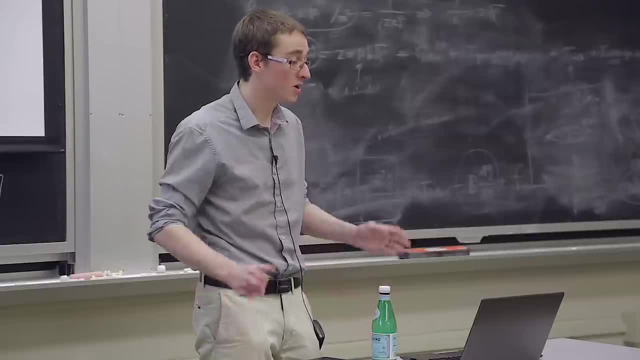 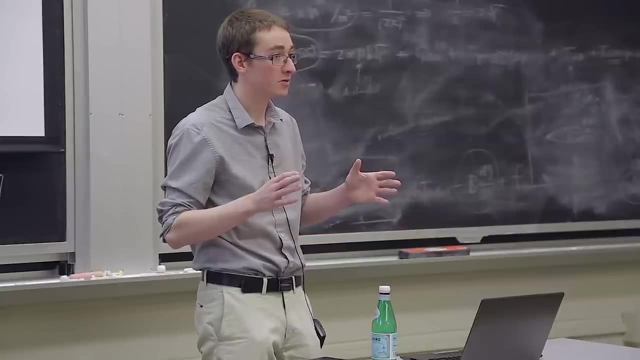 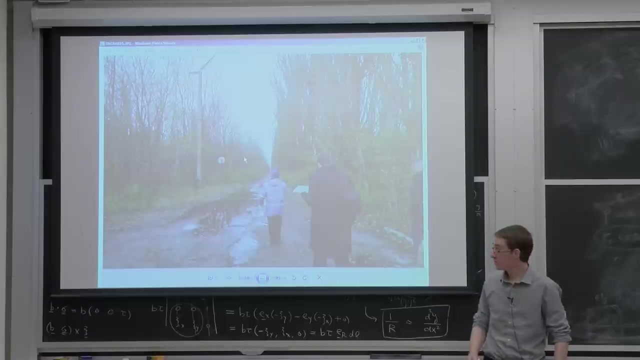 pretty much. now It's 75,. right, let's see. Last I checked, the new safe confinement arch was 75% of the way over the reactor itself. Regular tourist visits to Pripyat will continue to happen. This program that I went on. 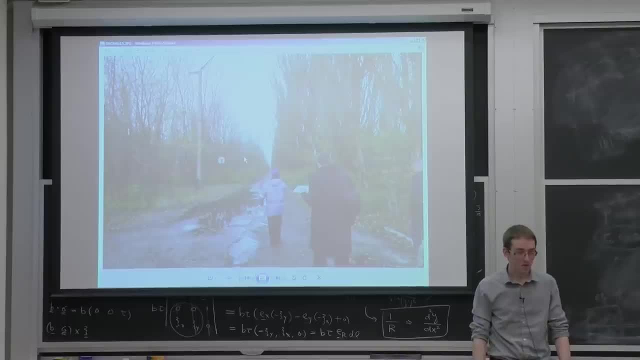 is something very special. Carl, Ed and Eric have done this type of thing once before. That was the trip I went on last year, and they intend on doing it once a year as long as they can, but that's pretty much your only opportunity. 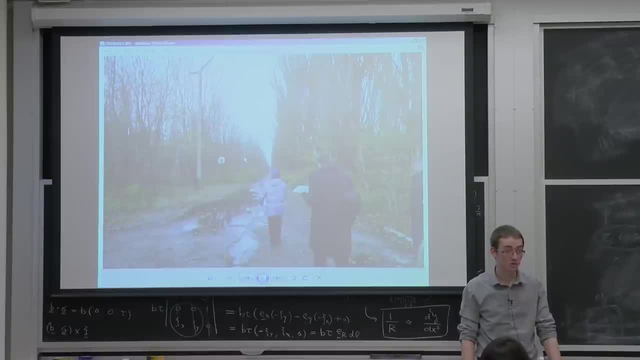 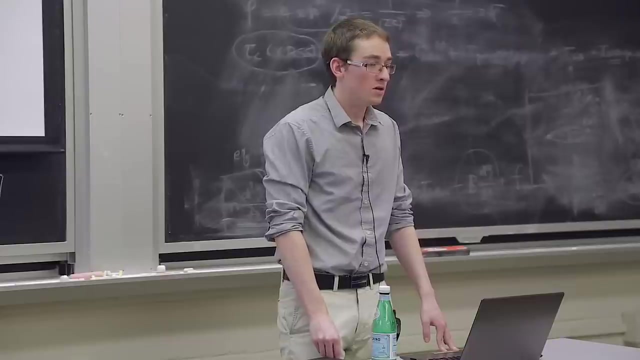 to get that kind of access to the reactor. It takes a lot of work. Anyone else got questions for Jake? It's rare to meet someone that's actually gone to Chernobyl in the state. Yeah, Do you think it's haunted?